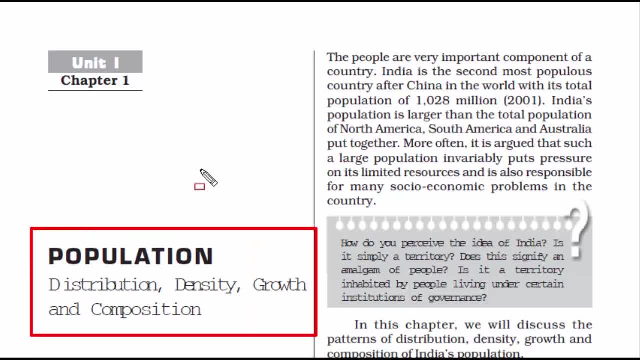 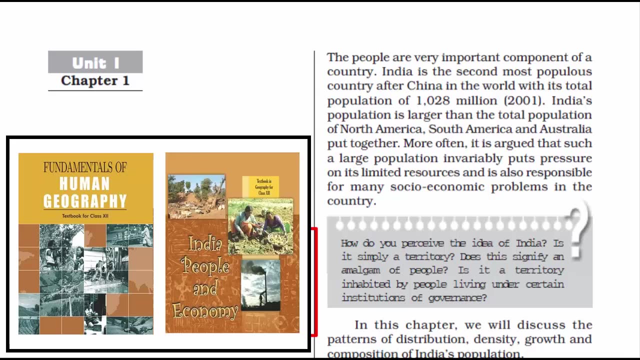 Chapter 1. Population, Distribution, Density, Growth and Composition. This is the first chapter of Class 12 Geography: India, People and Economy. There are two NCRT Geography books in Class 12.. The first one is Fundamentals of Human Geography and the second one is India, People and Economy. 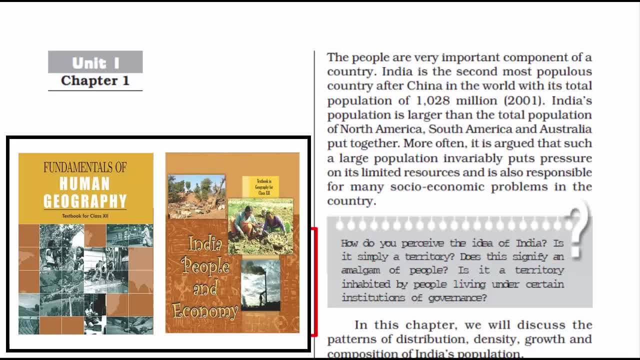 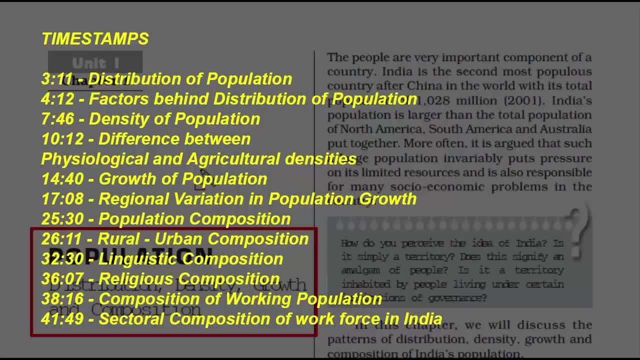 I have already covered the chapters of the other book. The link to that playlist is available in the description. Please have a look at it. The timestamps of this chapter are available in the description. If you want to skip over and save some time, please do that. So, without any further ado, let's begin. 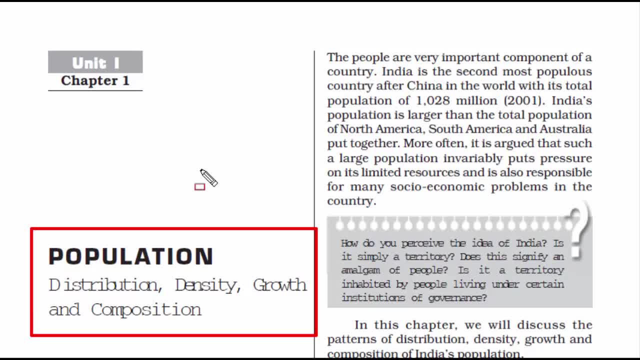 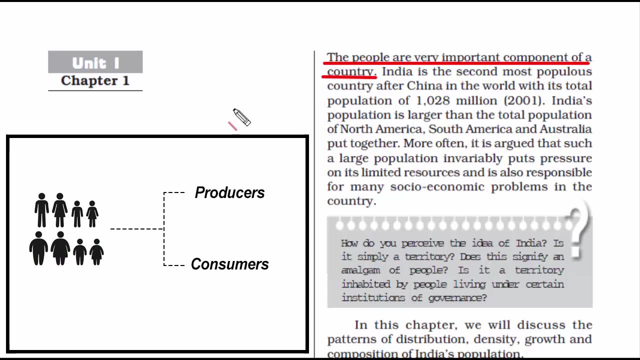 Since the title of this chapter is Population. therefore, we will learn a lot around the topic Population. So here it's written: the people are a very important component of a country, And the reason behind that is people are both the producers as well as the consumers. Human beings can make things, and it is the same human being who will consume that thing, And that is what makes the economy work. 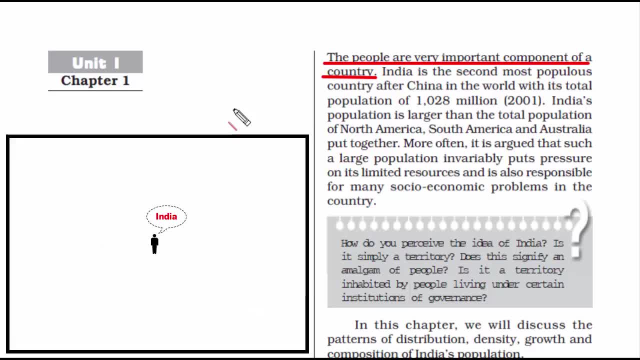 Another aspect is if you see the word nation or a country, basically it is an idea. It's like a social contract between a bunch of people who have this like-minded idea, where they choose to associate themselves with a particular tribe, society, state or a country. 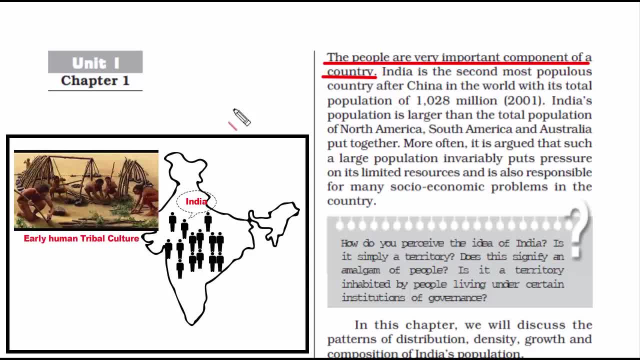 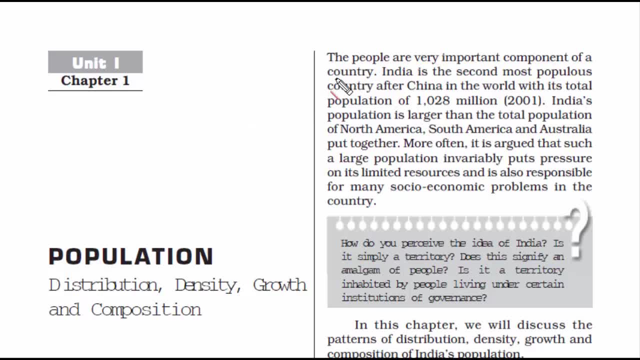 That's what happened in earlier times. So this is how the people are considered: as an important component of a country. Now, when you understand this, you also have to look at the other side. A large population puts pressure on its limited resources. 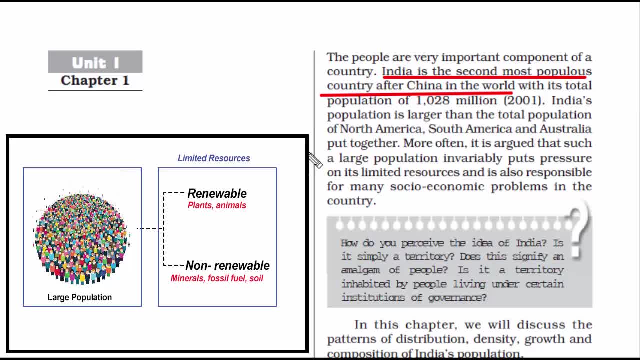 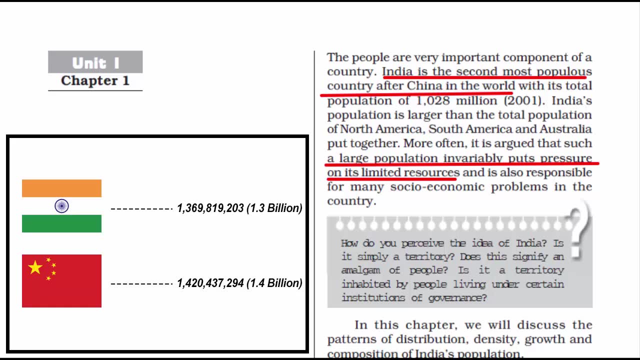 Because we know that natural resources are limited And human beings have unlimited desires. Hence it becomes very difficult to reconcile human beings' unlimited desires with limited resources. If you look at India and China, their populations are 1.3 billion and 1.4 billion respectively. 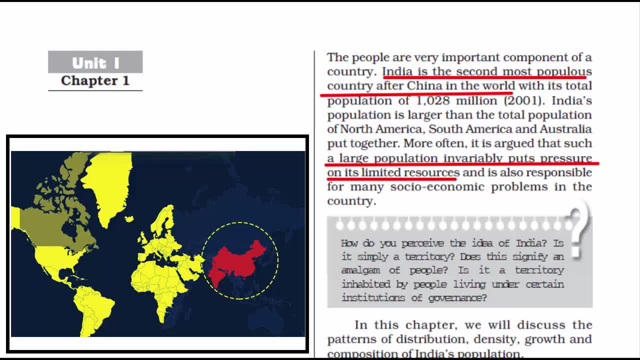 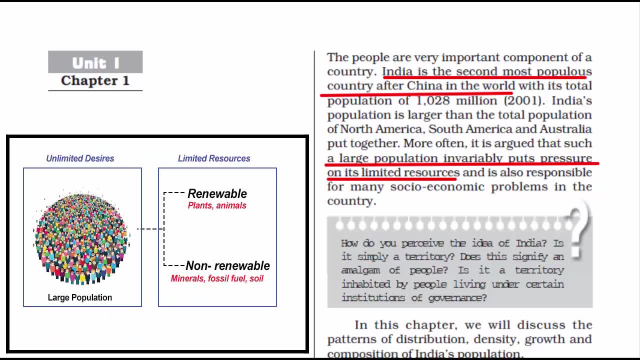 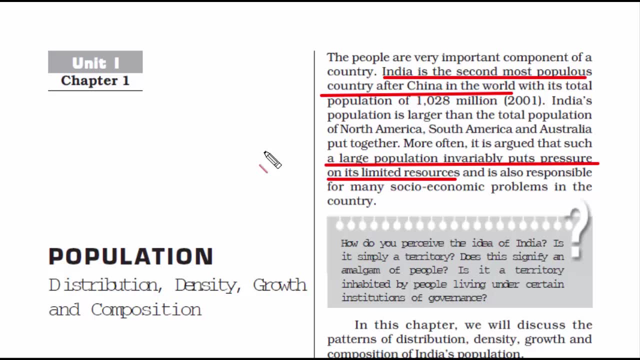 Now, basically, majority of the human beings on earth live in these two countries, So just imagine the needs of these two countries' population. As human population grow, human demands for resources like water, land, trees and energy also grow, And when a country is not able to meet its population's demand, that creates scarcity. 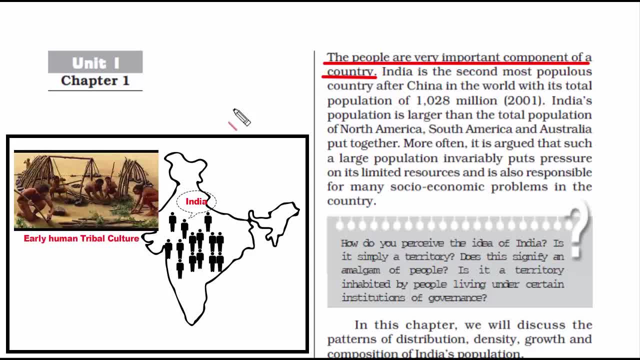 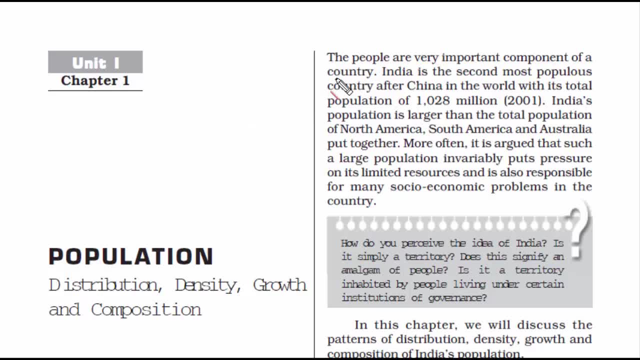 That's what happened in earlier times And it is still relevant today. So that is how the people are considered as an important component of a country. Now, when you understand this, you also have to look at the other side. A large population puts pressure on its limited resources. 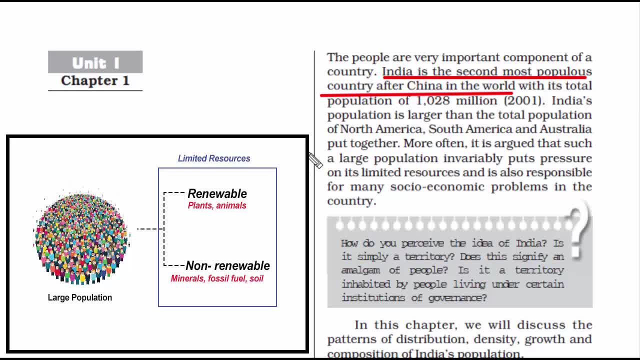 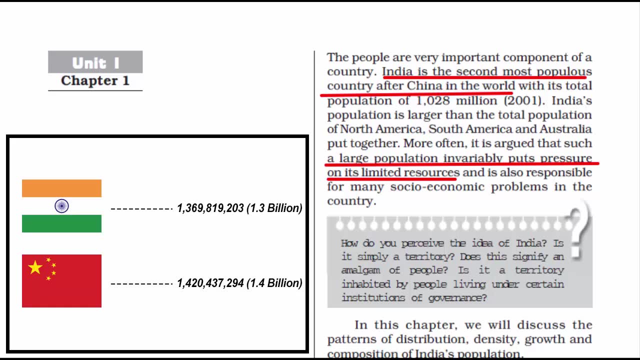 Because we know that natural resources are limited And human beings have unlimited desires. Hence it becomes very difficult to reconcile human beings' unlimited desires with limited resources. If you look at India and China, their populations are 1.3 billion and 1.4 billion respectively. 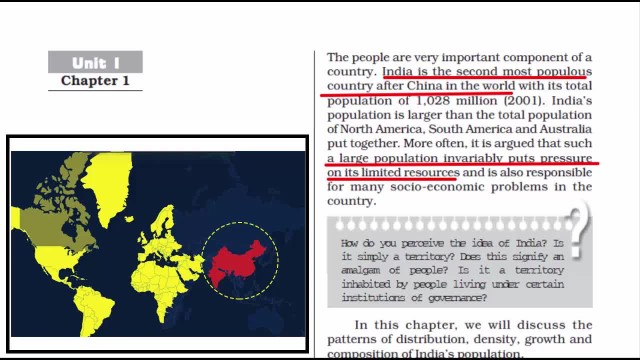 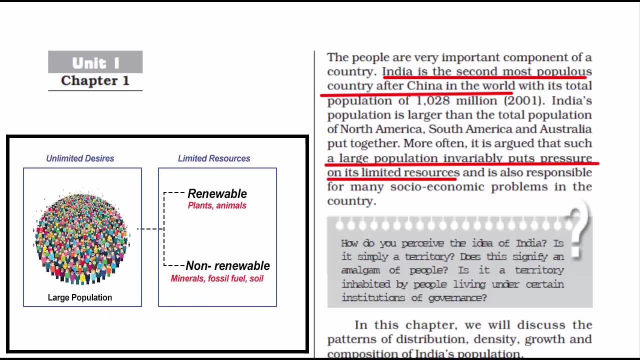 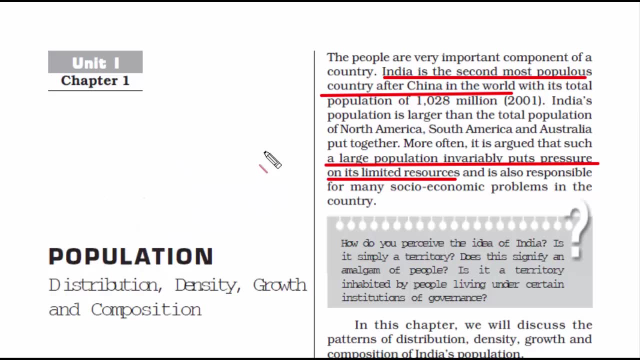 Now, basically, majority of the human beings on earth live in these two countries, So just imagine the needs of these two countries' population. As human population grow, human demands for resources like water, land, trees and energy also grow, And when a country is not able to meet its population's demand, that creates scarcity. 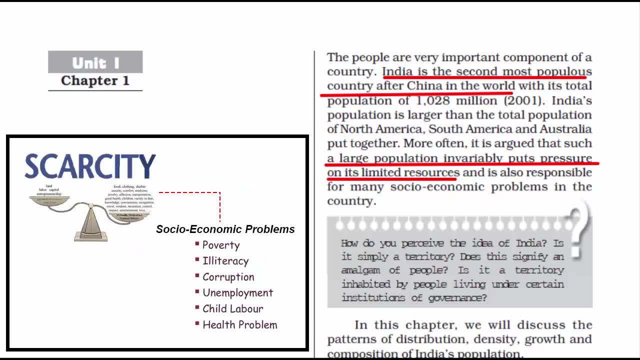 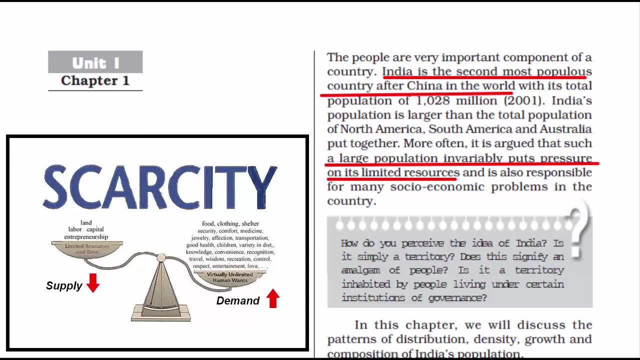 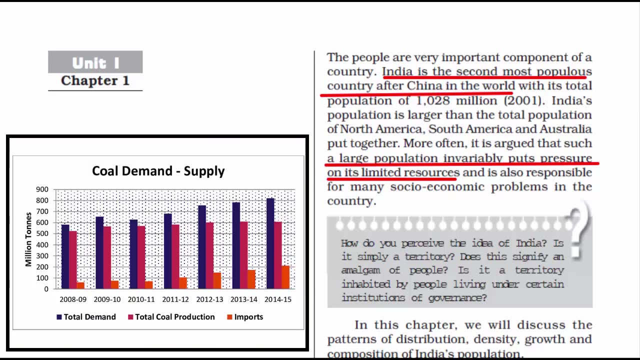 And scarcity gives rise to many socio-economic problems. During scarcity, demand increases and supply is usually low. A good example would be: during summer you need electricity. All of a sudden, the demand for energy increases And you will notice the demand for energies is always greater than the supply. 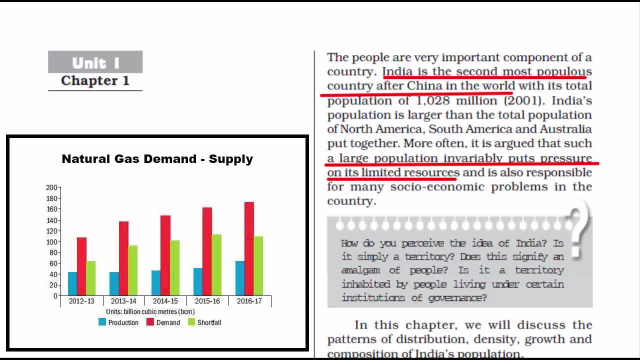 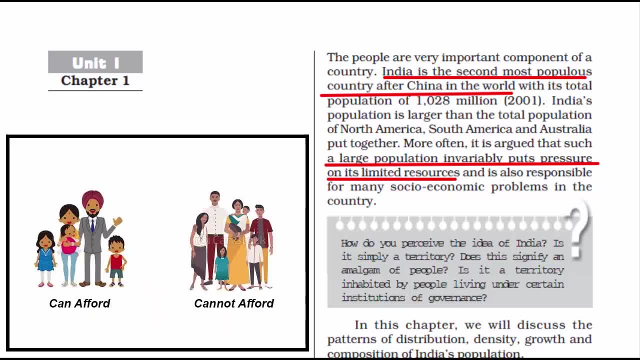 Because it takes a lot of time and effort to produce electricity. That is why the price of electricity also increases during summer. In a society, there will be some who can afford this price-wise, But there will be many who cannot, because it will directly affect their household income. 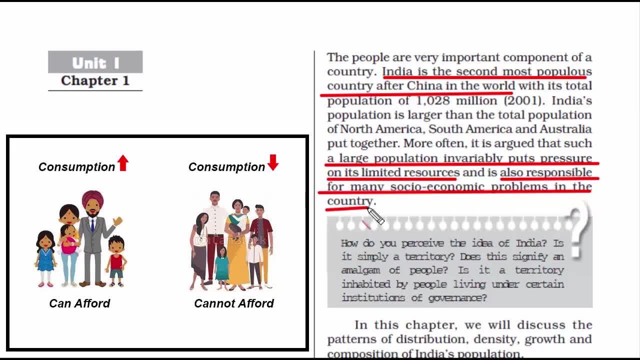 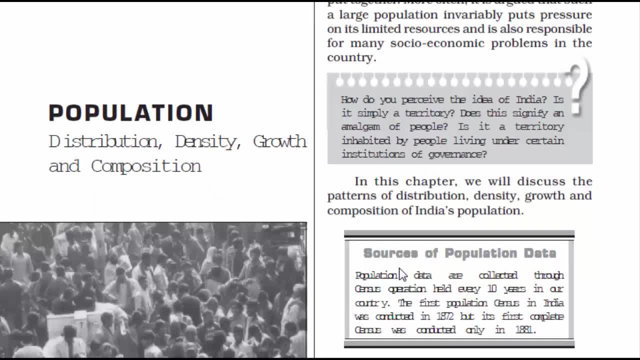 In that case, many have to bear the heat of the summer And some may reap the benefit of an air conditioner, And that's how you will notice a socio-economic divide in the society. So, anyhow, in this chapter we will discuss the patterns of distribution, density, growth and composition of India's population. 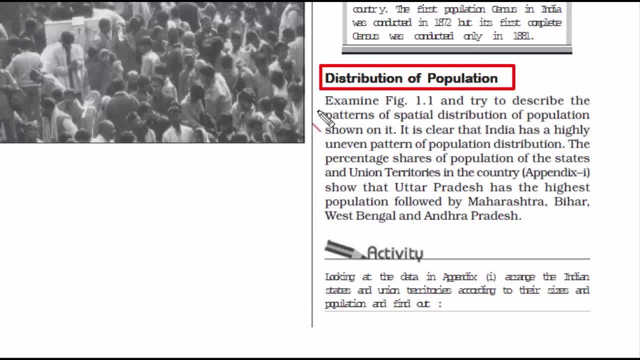 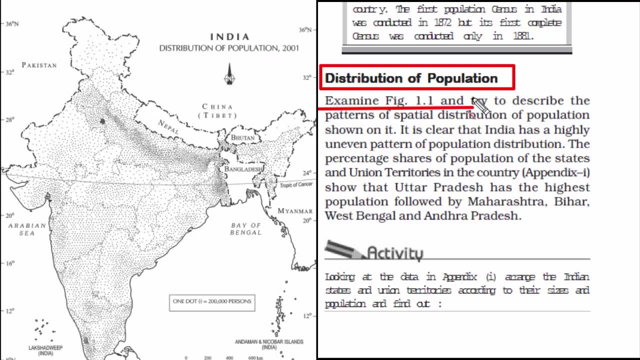 So the first topic is distribution of population. When you look at this figure, you can see how these tiny dots are distributed all across the India map, And here it says 1 dot is equal to 2 lakh persons. You will notice at some places the concentration of dots are more. 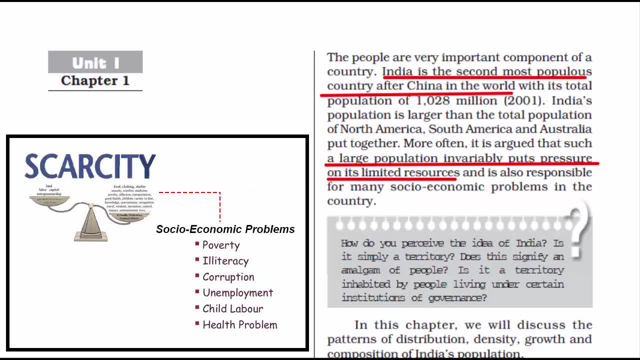 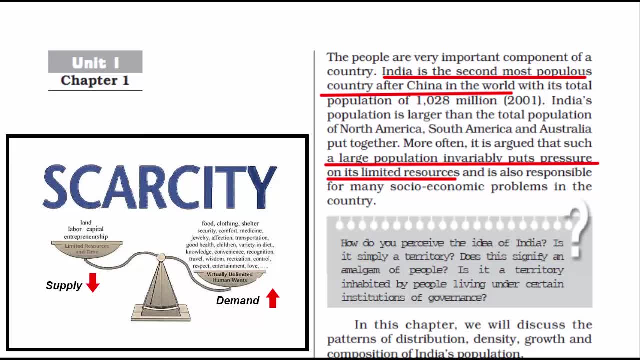 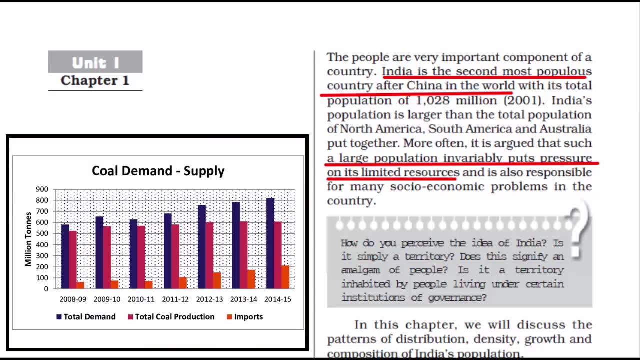 And scarcity gives rise to many socio-economic problems. During scarcity, demand increases and supply is usually low. A good example would be: during summer you need electricity. All of a sudden, the demand for energy increases And you will notice the demand for energies is always greater than the supply. 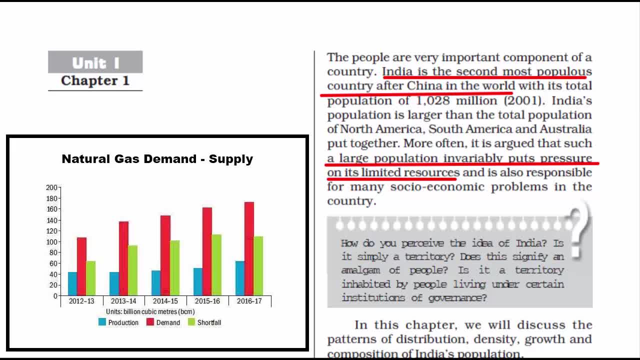 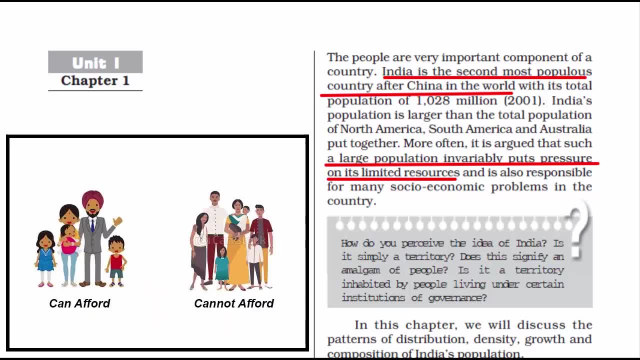 Because it takes a lot of time and effort to produce electricity. That is why the price of electricity also increases during summer. In a society, there will be some Who can afford this price wise, But there will be many who cannot, Because it will directly affect their household income. 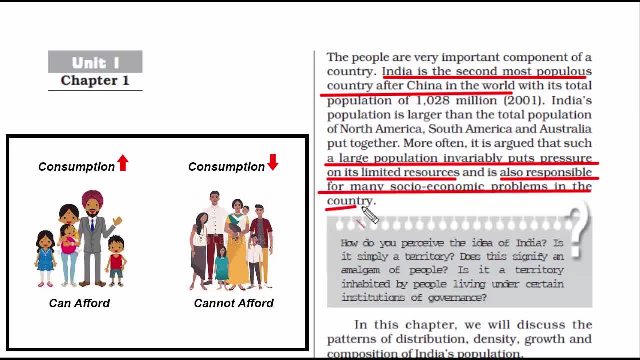 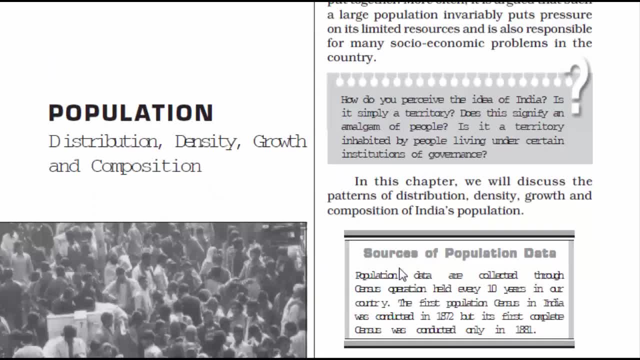 In that case, many have to bear the heat of the summer And some may reap the benefit of an air conditioner, And that's how you will notice a socio-economic divide in the society. So, anyhow, in this chapter we will discuss the patterns of distribution, density, growth and composition of India's population. 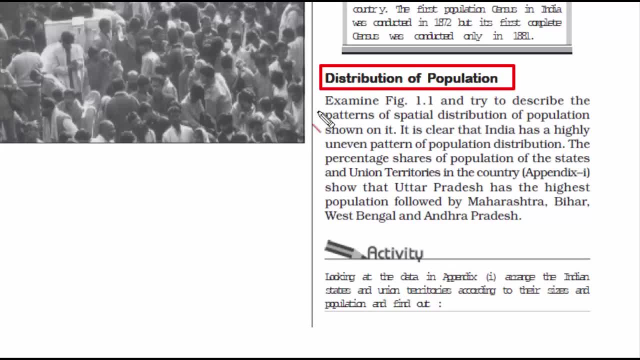 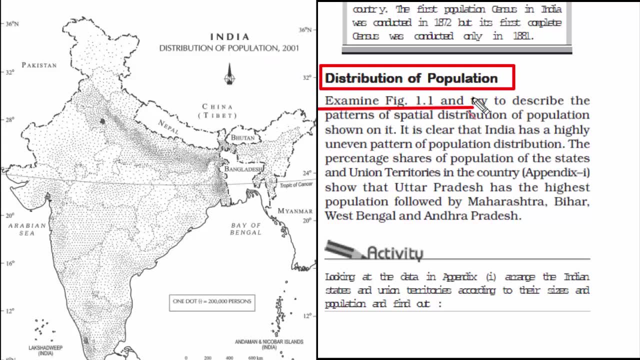 So the first topic is distribution of population. When you look at this figure, you can see how these tiny dots are distributed all across the India map, And here it says one dot is equal to two lakh persons. You will notice at some places the concentration of dots are more. 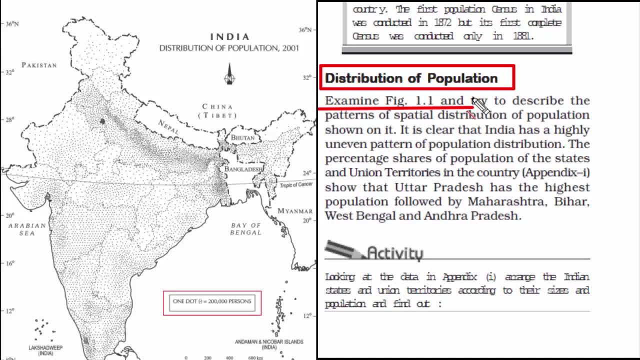 These are places where population is comparatively higher, And then there are places where you will find it less. These are usually rural areas or the geographical or physical landscape is such that it makes human settlement tough. If you look at the states of Maharashtra, Bihar, West Bengal, Telangana, Andhra Pradesh, Tamil Nadu, Madhya Pradesh, Rajasthan, Karnataka and Gujarat, 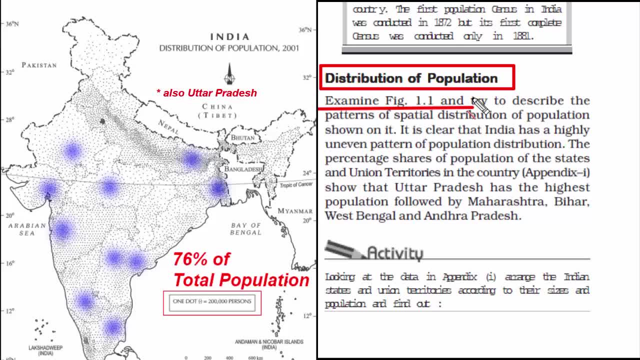 Together they have around 76% of the total population of India. On the other hand, states like Jammu and Kashmir, Himachal Pradesh, Uttarakhand and Arunachal Pradesh. There the population is very small, despite the fact that these states have large geographical area. 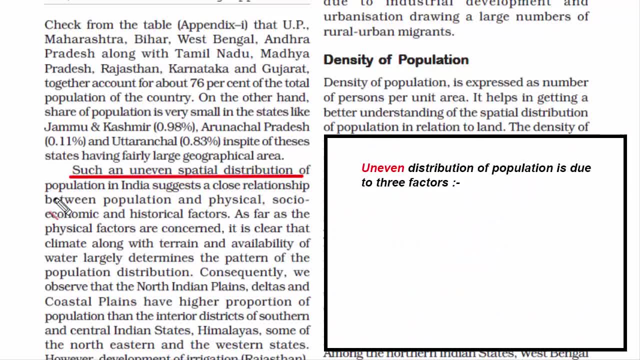 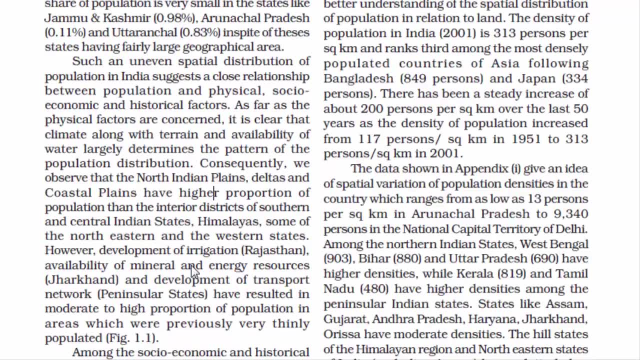 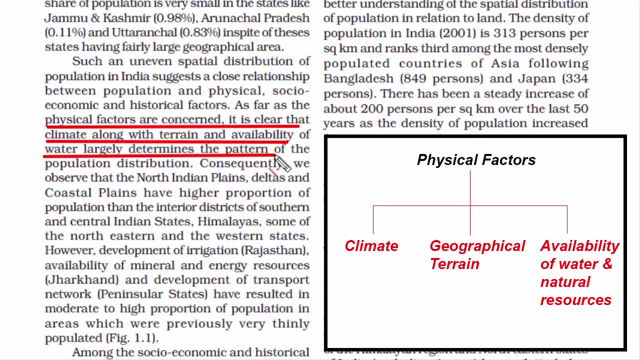 Now, the reason behind this kind of distribution of population Is due to three factors: Physical factor, socio-economic factors and historical factors. When we say physical factors, we are talking about the climate of that particular place And availability of water and other natural resources. 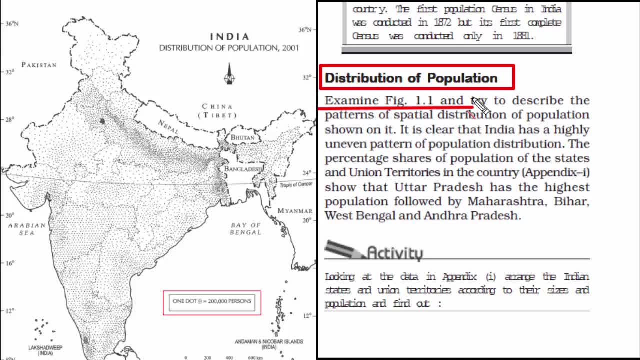 These are places where population is comparatively higher, And then there are places where you will find it less. These are usually rural areas or the geographical or physical landscape is such that it makes human settlement less. If you look at the states of Maharashtra, Bihar, West Bengal, Telangana, Andhra Pradesh, Tamil Nadu, Madhya Pradesh, Rajasthan, Karnataka and Gujarat, 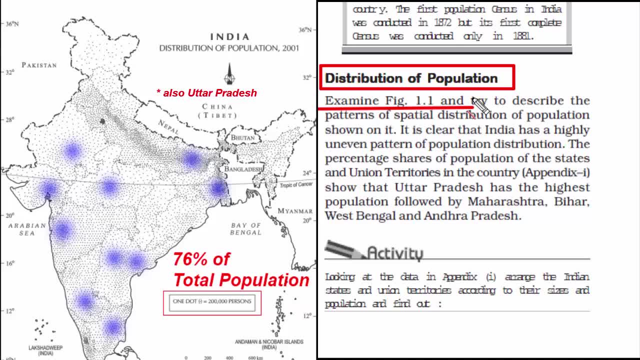 together they have around 76% of the total population of India. On the other hand, states like Jammu and Kashmir, Himachal Pradesh, Uttarakhand and Arunachal Pradesh. there the population is very small, despite the fact that these states have large geographical area. 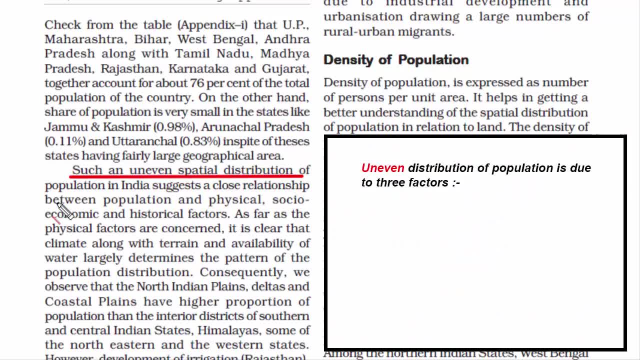 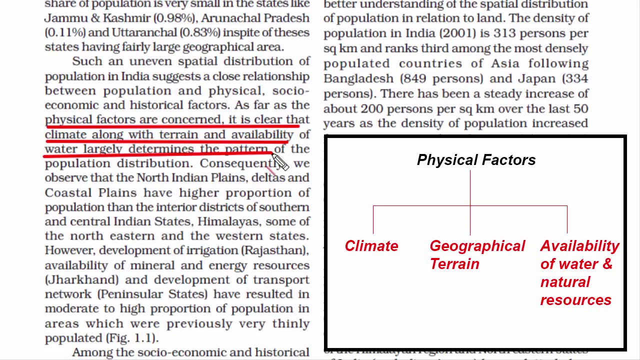 Now, the reason behind this kind of distribution of population is due to three factors: Physical factor, socio-economic factors and historical factors. When we say physical factors, we are talking about the climate of that particular place And availability of water and other natural resources. 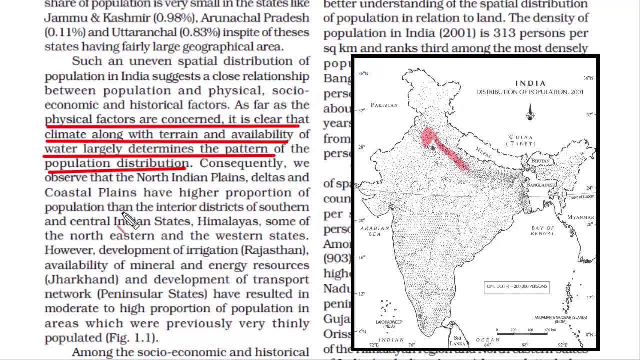 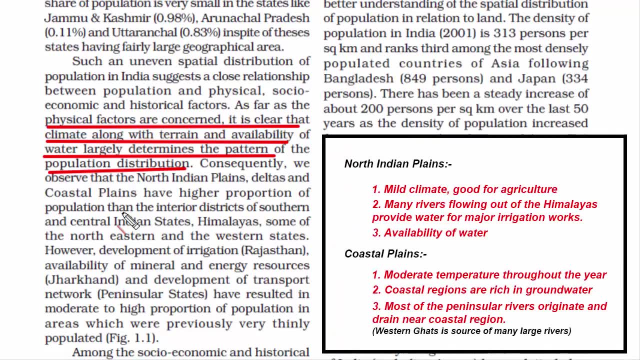 If you look at the map, you can clearly see that regions like the North Indian Plain and the coastal regions have higher population, And the reason is clearly because of the climate And the availability of water. Similarly, if you look at the interior regions of some southern and central states, 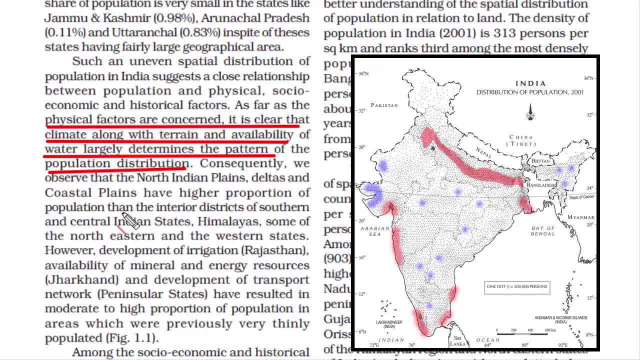 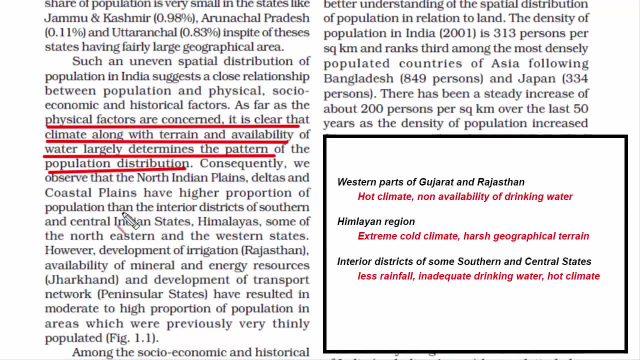 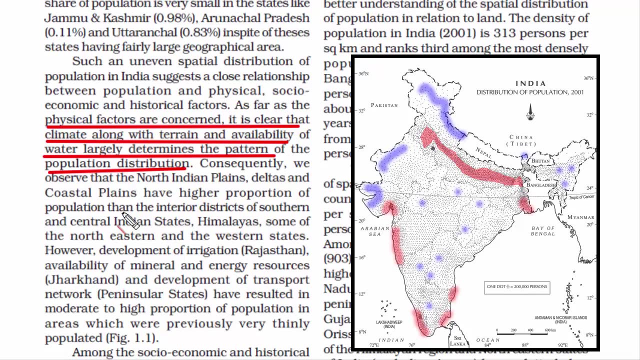 then the north eastern states, then western part of Gujarat and Rajasthan, places near the Himalayas. here the population is less due to extreme climate, harsh terrain and availability of drinking water. However, today, in modern India, these places are attracting quite a lot of human settlements. 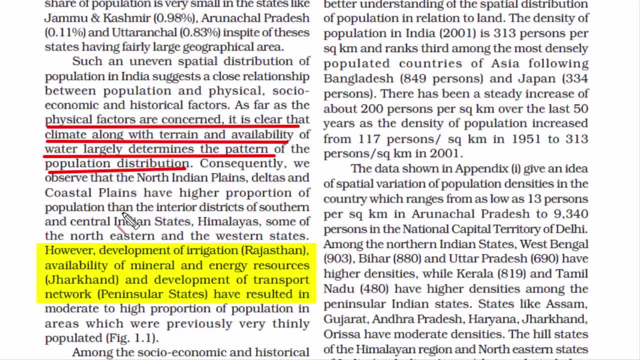 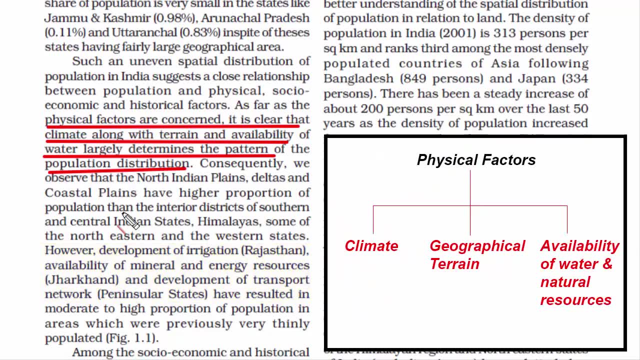 because of agricultural development, availability and extraction of mineral and energy resources, and also development of transport network. So this is what we mean when we say physical factor being one of the reason behind the distribution of population. The second one is the socio-economic factors. 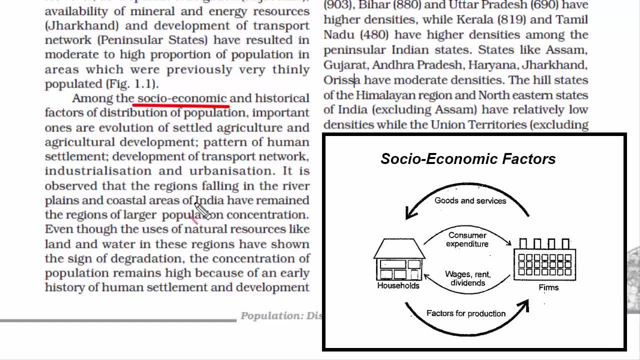 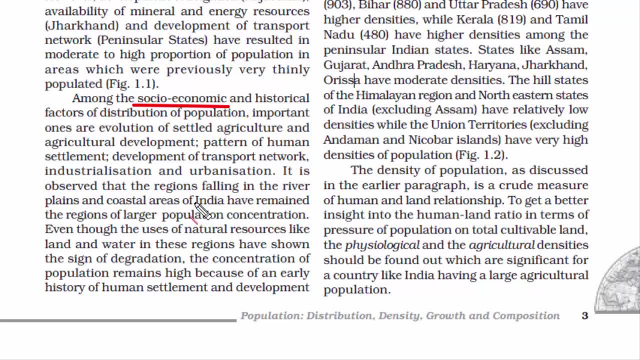 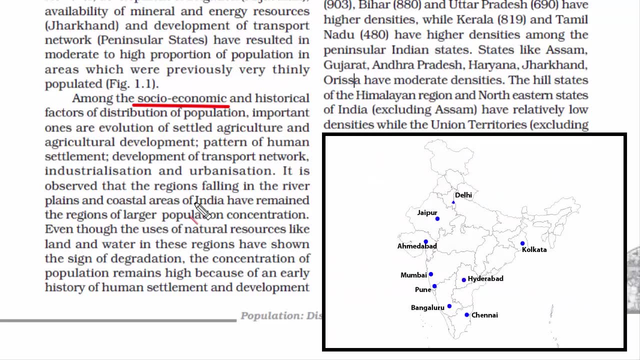 When we say socio-economic factors, we basically mean how economic activities affect the society. In other words, we analyze how societies progress and regress because of their local or regional economy, or sometimes global economy. When you look at the urban regions of Delhi, Mumbai, Kolkata, Bangalore, Pune, Hyderabad, Ahmedabad, Chennai and Jaipur, 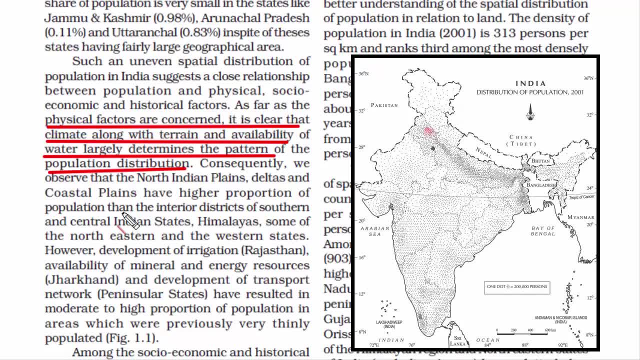 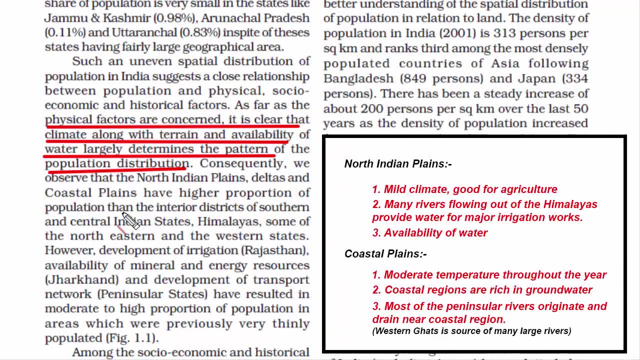 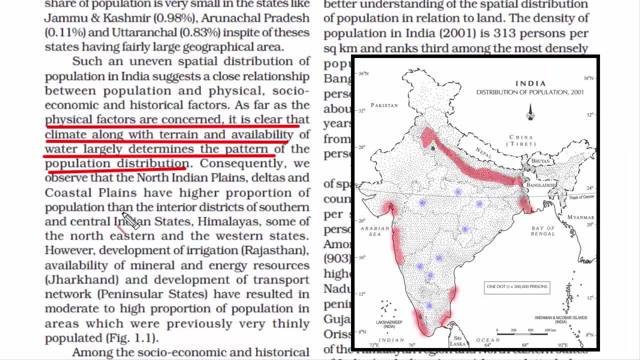 If you look at the map, you can clearly see that regions like the North Indian plain and the coastal regions have higher population, And the reason is clearly because of the climate and the availability of water. The interior regions of some southern and central states, then the northeastern states, then western part of Gujarat and Rajasthan, places near the Himalayas- here the population is less due to extreme climate, harsh terrain and availability of drinking water. 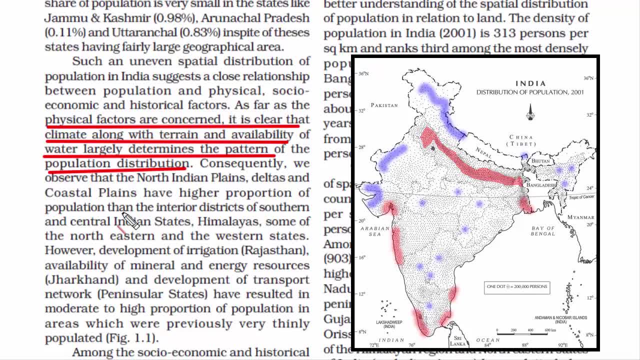 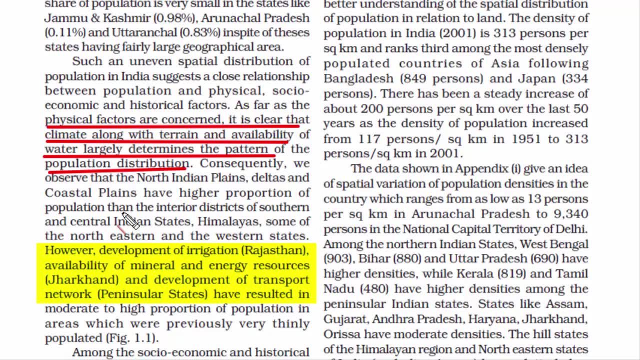 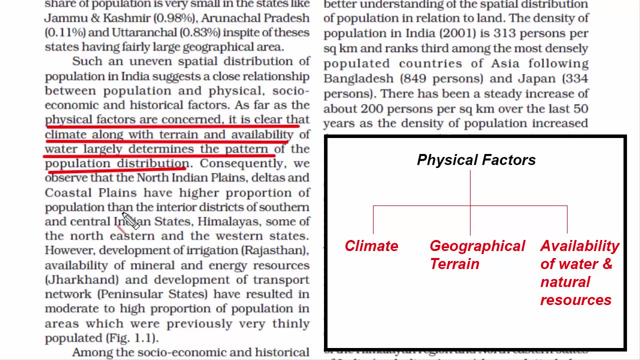 However, today in modern India, these places are attracting quite a lot of human settlements because of agricultural development, availability and extraction of mineral and energy resources, and also development of transport network. So this is what we mean when we say physical factor being one of the reason behind the distribution of population. 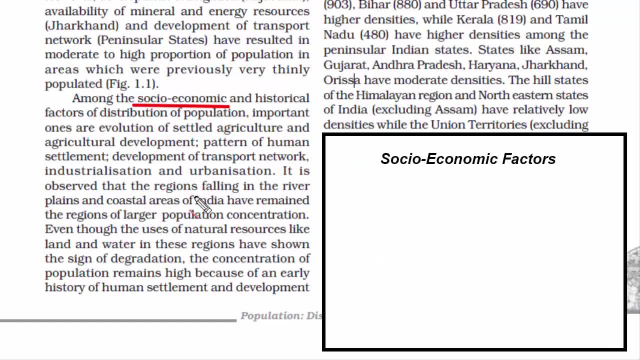 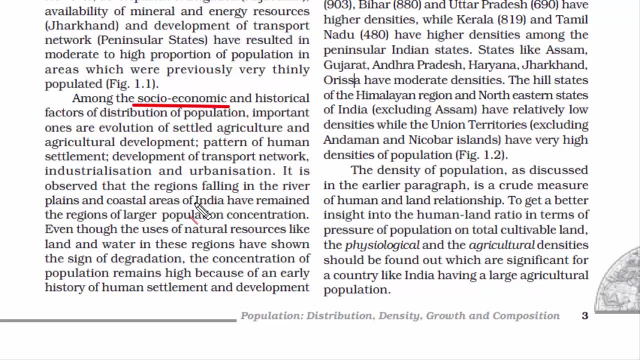 The second one is the socio-economic factors. When we say socio-economic factors, we basically mean how economic activities affect the society. In other words, we analyze how societies progress and regress because of their local or regional economy, or sometimes global economy. When you look at the urban regions of Delhi, Mumbai, Kolkata, Bangladesh, India and India, 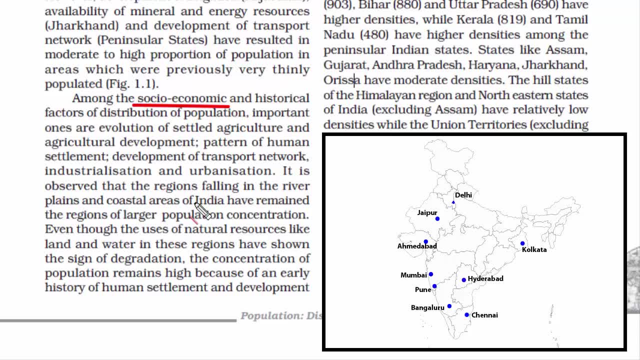 When you look at the urban regions of Delhi, Mumbai, Kolkata, Bangladesh, India and India. when you look at the urban regions of Delhi, Mumbai, Kolkata, Bangladesh, India and India, Bangalore, Pune, Hyderabad, Ahmedabad, Chennai and Jaipur, In these places you will find high 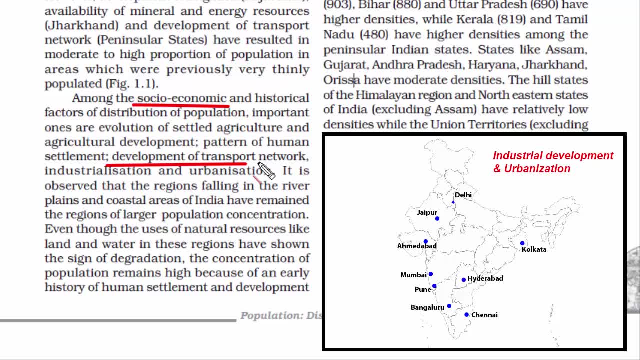 concentration of population, and it is due to industrial development and urbanization. You will also notice that these are the cities that generate a lot of revenue and contributes heavily to India's GDP Plus. today, everyone needs employment. In theory, we know that employment happens where there is development. If the big developments are happening in these major 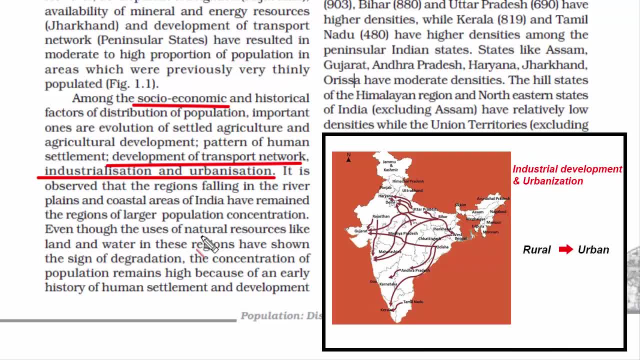 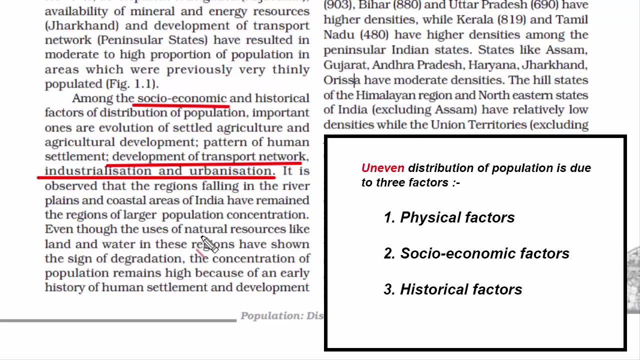 cities, don't you think it is obvious that it will attract a lot of people from rural areas? Of course, right. In other words, we call it rural to urban migration or urbanization. So this is how socio-economic factors make the distribution of population of a country uneven. 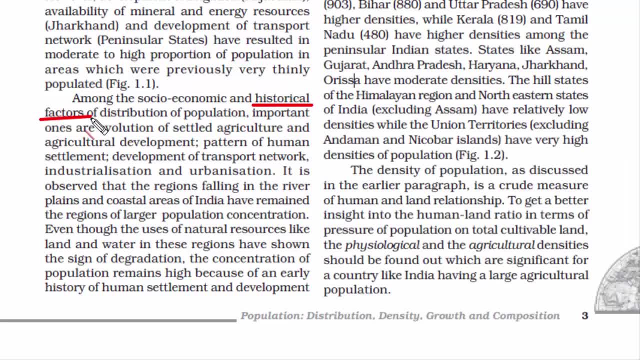 And the third factor is historical factors. By this we mean that the reason behind uneven population distribution has to be based on the historical facts. or it is based on the historical facts. or it is based on the historical facts, Because historical processes should also be taken into account. 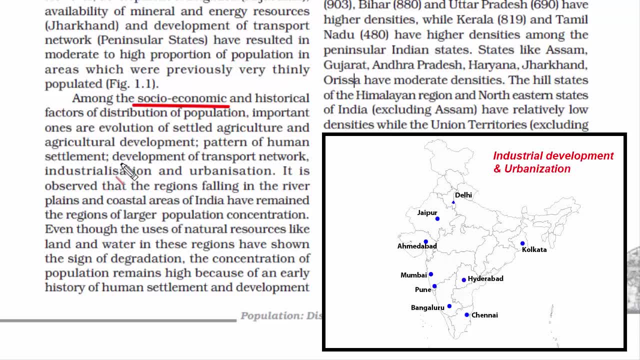 in these places you will find high concentration of population, and it is due to industrial development and urbanization. You will also notice that these are the cities that generate a lot of revenue and contributes heavily to India's GDP Plus. today, everyone needs employment. In theory, we know that employment happens where there is development. 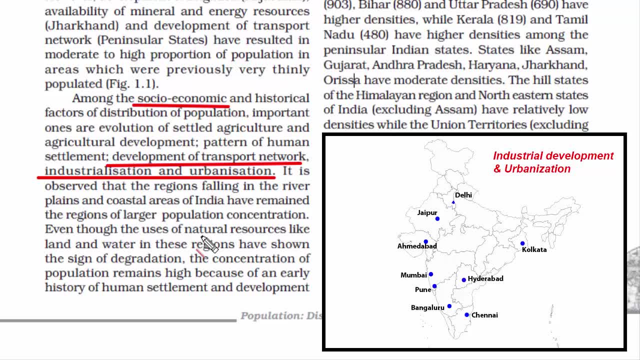 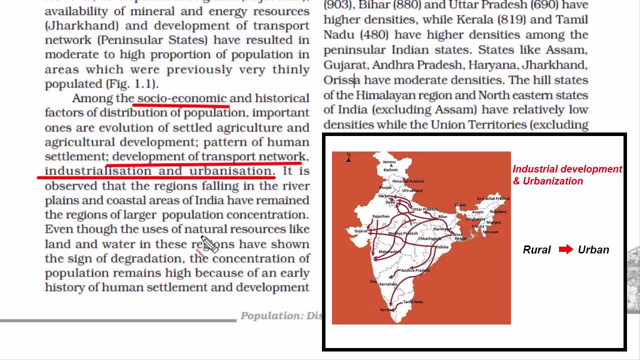 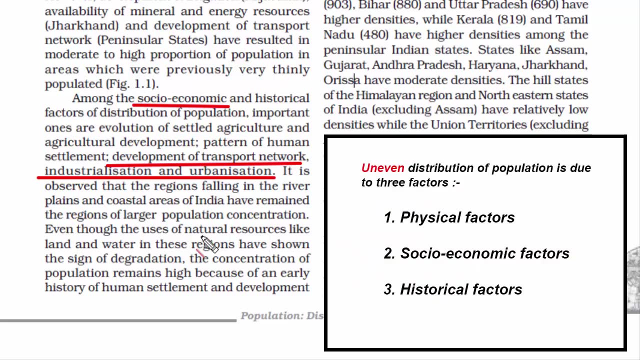 Big developments are happening in these major cities, Don't you think it is obvious that it will attract a lot of people from rural areas? Of course, right. In other words, we call it rural to urban migration or urbanization. So this is how socio-economic factors make the distribution of population of a country uneven. 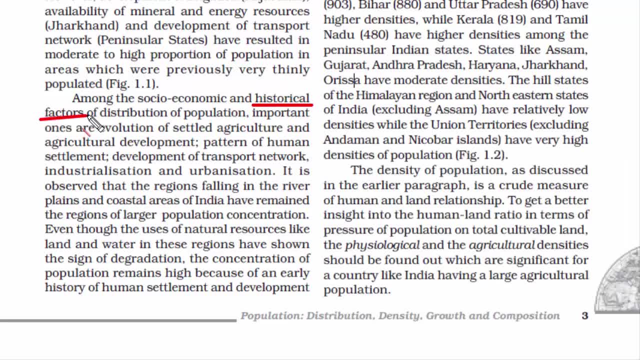 And the third factor is historical factors. By this we mean that the reason behind uneven population distribution has to be based on the historical facts, or it is based on people and event of the past, Because historical processes should also be taken into account while explaining the patterns of population distribution. 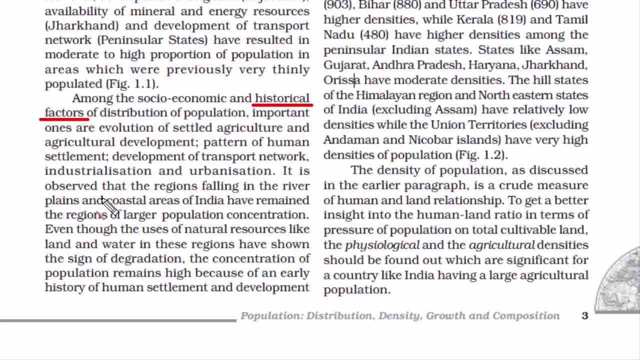 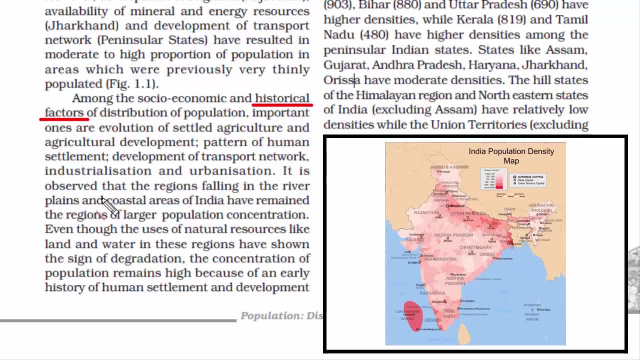 If you look at the duration of the human settlement at a particular place, it will tell you why the population is so much concentrated at that area. If you look at the most densely populated areas in India, they have a very long history of human habitation. 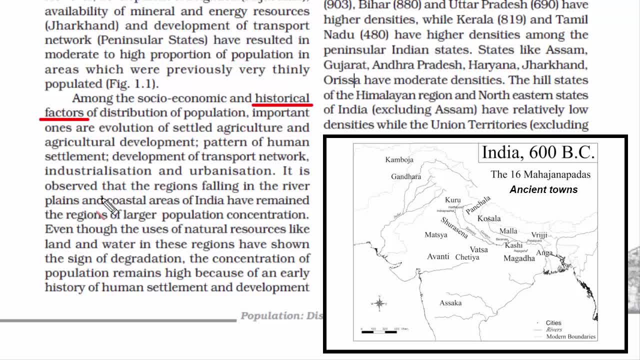 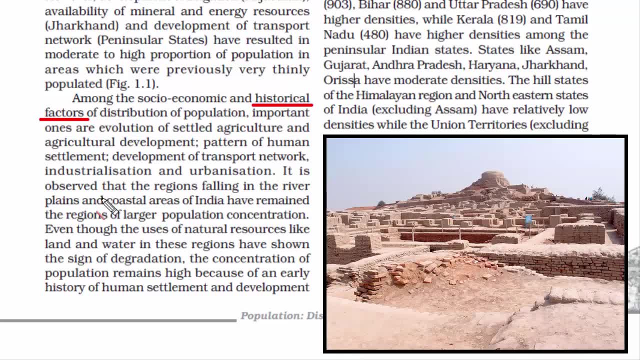 Some of the early trading towns and markets were set up in these places. Then if you go back to the time of Indus Valley Civilization or the Harappan Civilization, which is also called as the earliest known urban culture of the Indian subcontinent, 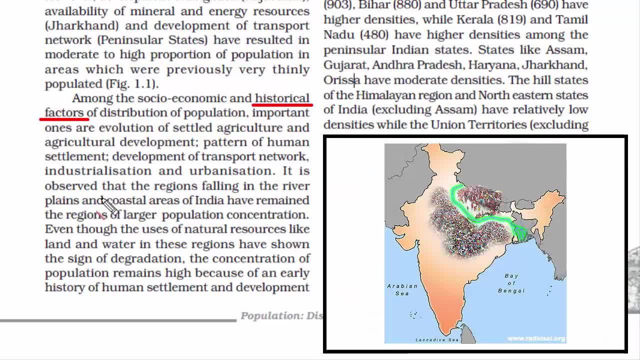 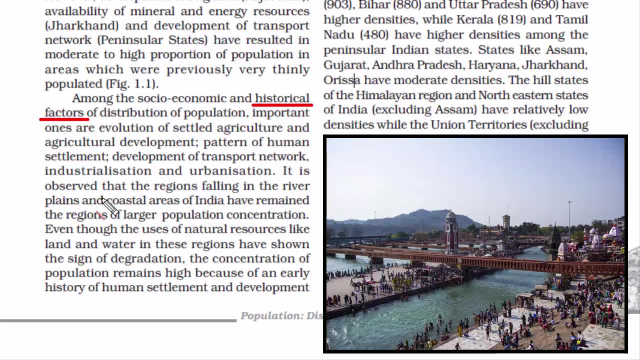 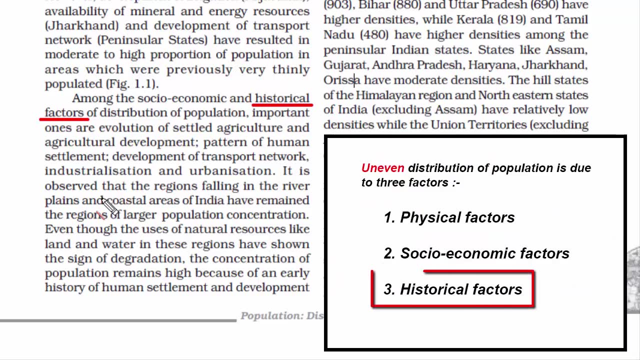 it provides a strong evidence that the Indian civilization had begun in and around the Ganges Valley, And that's how, with time, not only these places evolved, the population also grew, as generation after generation people continued to live in these places, And that is what we mean when we say how historical factors are the reason behind the distribution of population in India. 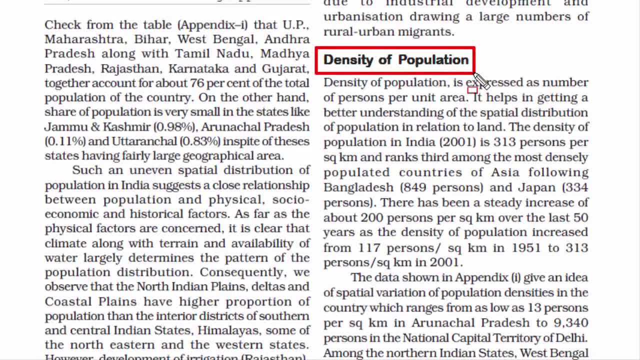 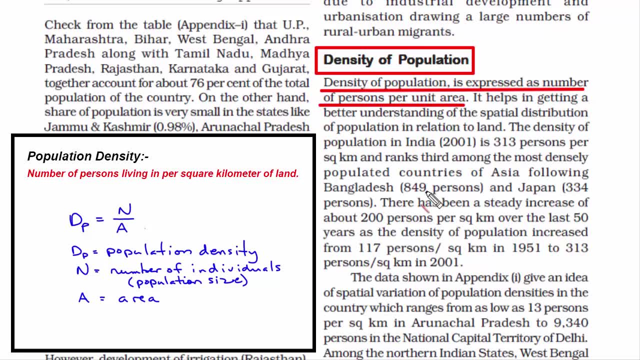 Now let's go to the next topic: density of population. It is defined as the number of persons living in per square kilometer of land. It helps in getting a better understanding of the spatial distribution of population in relation to land. It is also used to measure the intensity of land use by people. 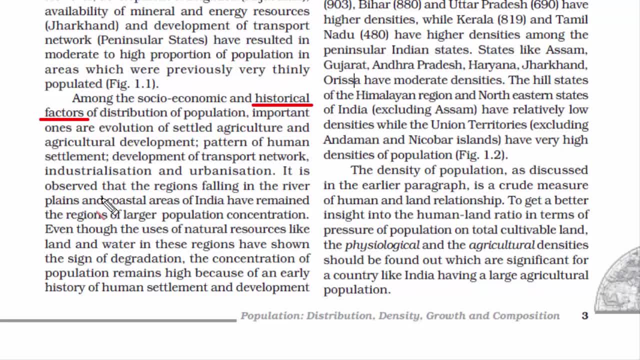 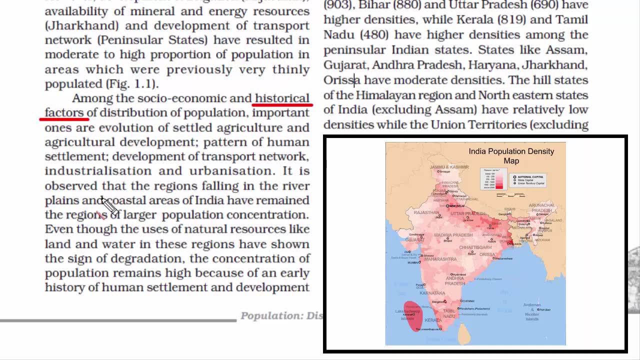 while explaining the patterns of population distribution. If you look at the duration of the human settlement at a particular place, it will tell you why the population is so much concentrated at that area. If you look at the most densely populated areas in India, they have a very long history. 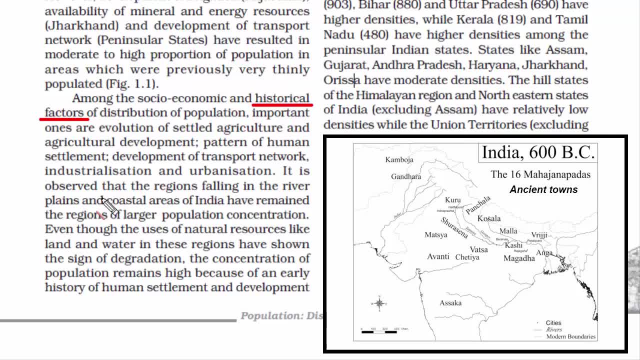 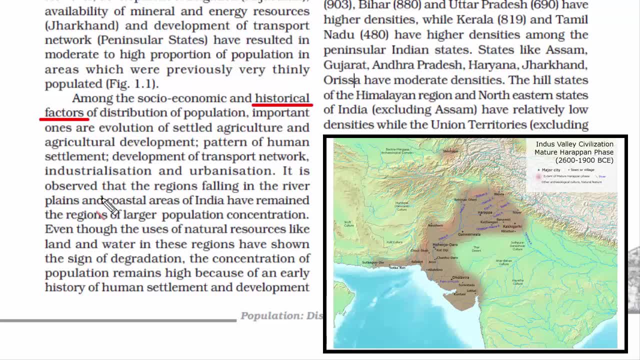 of human habitation. Some of the early trading towns and markets were set up in these places. Then if you go back to the time of Indus Valley civilization or the Harappan civilization, which is also called as the earliest known urban culture of the Indian subcontinent, 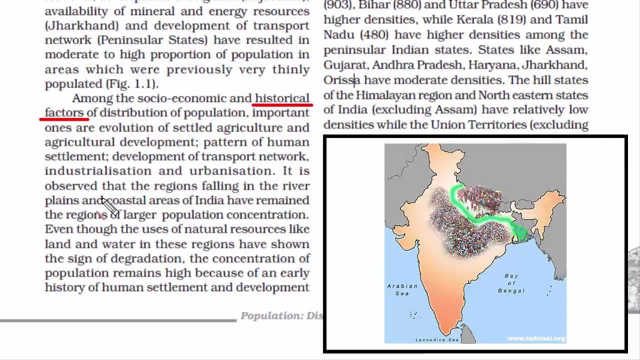 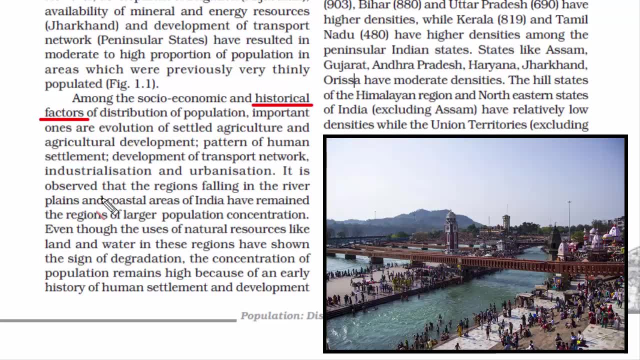 it provides a strong evidence that the Indian civilization had begun in and around the Ganges valley, And that's how, with time, not only these places evolved, the population also grew, as generation after generation people continued to live in these places, And that is what we mean. 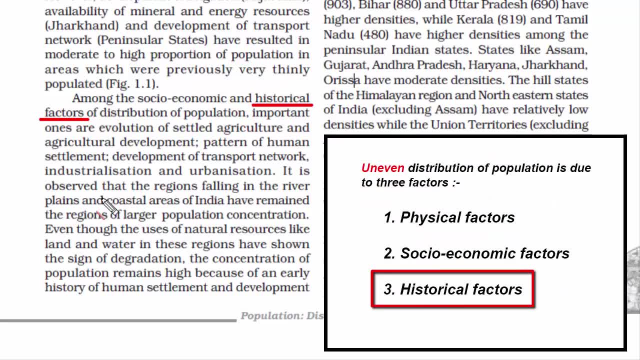 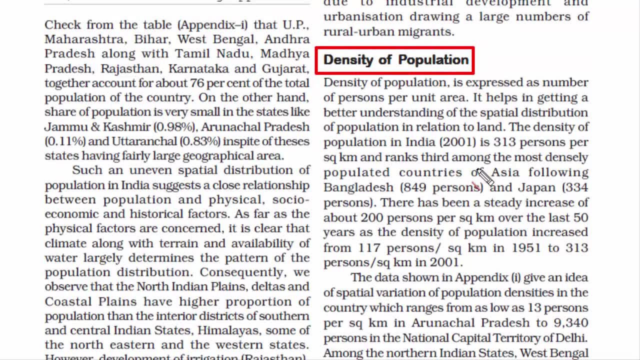 when we say how historical factors affect the civilization of the Indian subcontinent. Now let's go to the next topic: Density of Population. It is defined as the number of persons living in per square kilometer of land. It helps in getting a better understanding of the spatial distribution of population. 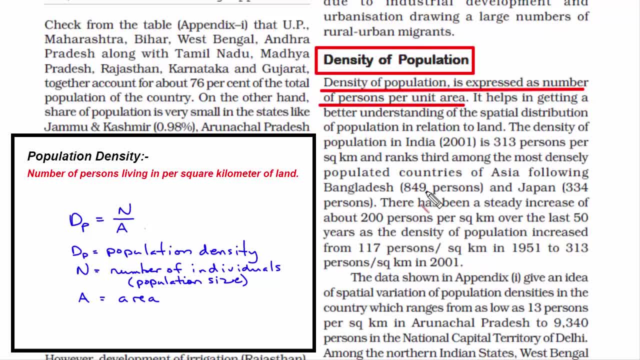 in relation to land. It is also used to measure the intensity of land used by people. To calculate the population density, you will have to divide the population by the size of the area. The population density is calculated by the number of people living in the area. 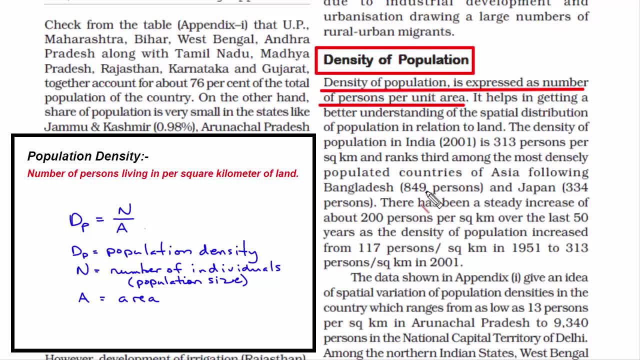 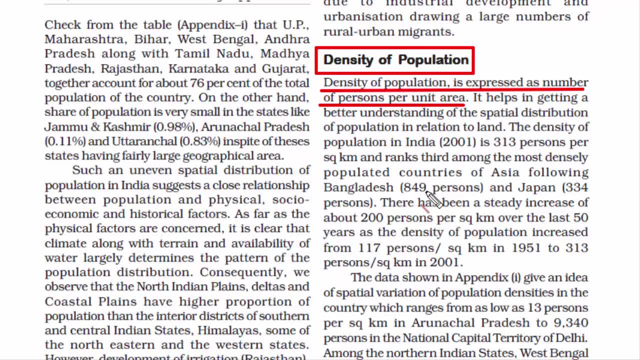 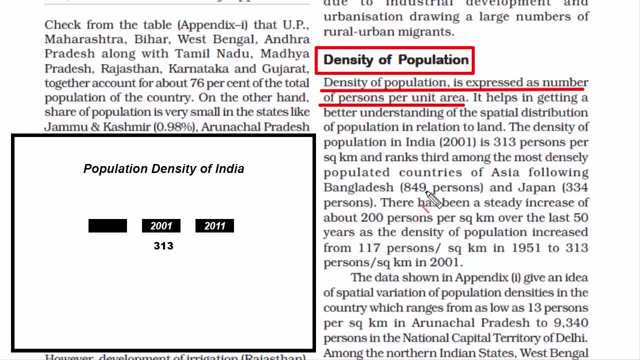 The population density is calculated by the number of people living in the area. Population density is equal to number of people divided by land area. In India, the population density is on the rise. The density of population in India, according to 2001 census, was at 313 persons per square kilometer. In 1951, it was 117 persons per. 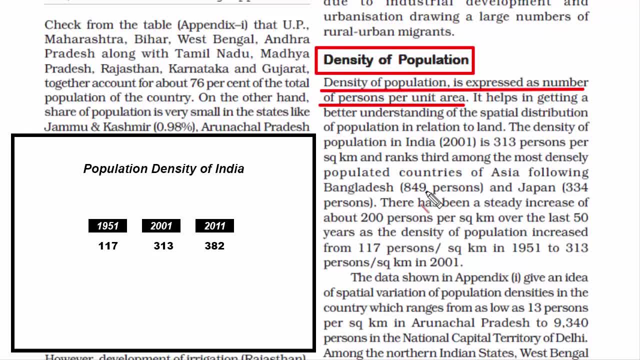 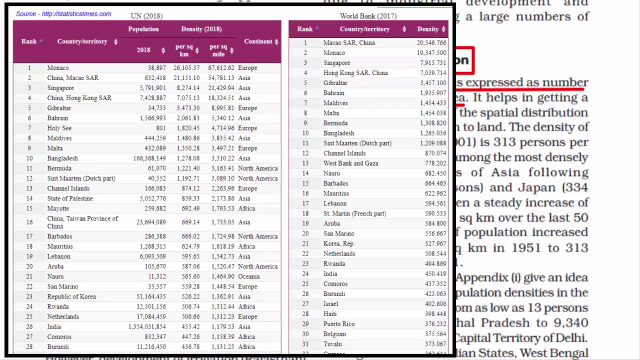 square kilometer. As per 2011 census, it has gone up to 382 persons per square kilometer. That means now 69 more people live in a square kilometer area in the country than the number that lived 10 years ago. Here is a list of countries ranked in order of their population density. 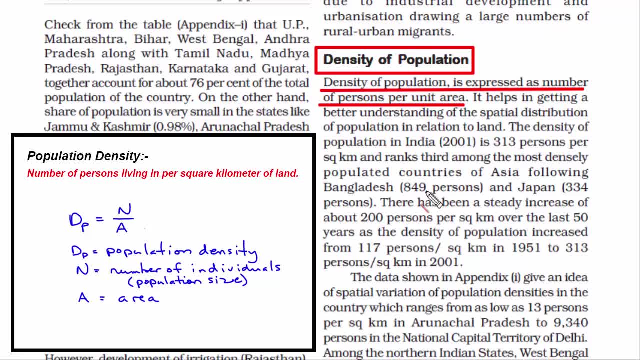 To calculate the population density, you will have to divide the population by the size of the area. Population density is equal to number of people divided by land area. In India, the population density is on the rise. The density of population in India, according to 2001 census, was at 313 persons per square kilometer. 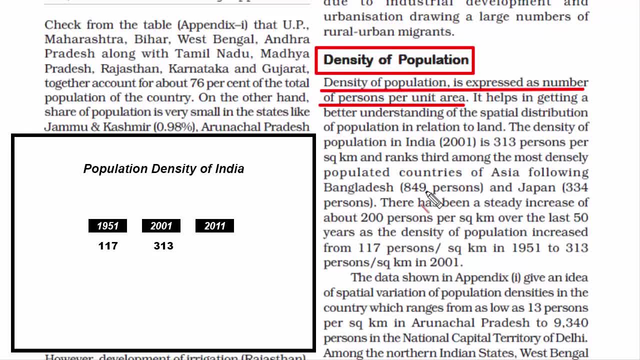 In 1951, it was 117 persons per square kilometer. As per 2011 census, it has gone up to 382 persons per square kilometer. That means now 69 more people live in a square kilometer area in the country than the number that lived 10 years ago. 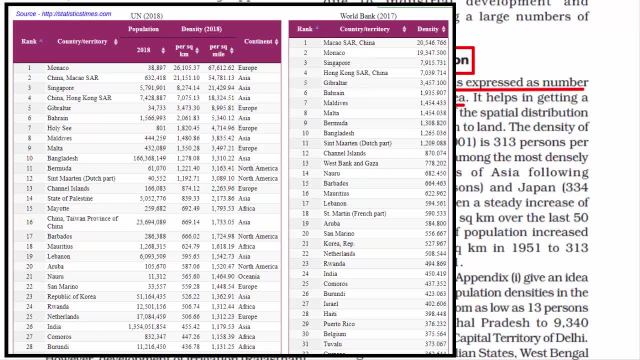 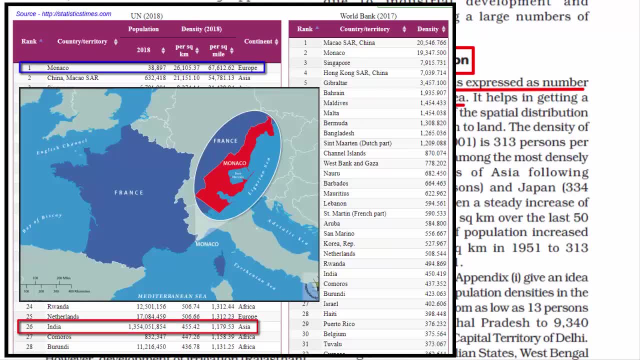 Here is a list of countries ranked in order of their population density. India is the 26th rank. If you look at Monaco, it is a tiny independent city-state on France's Mediterranean coastline. An average person can walk across the width of the country in about an hour. 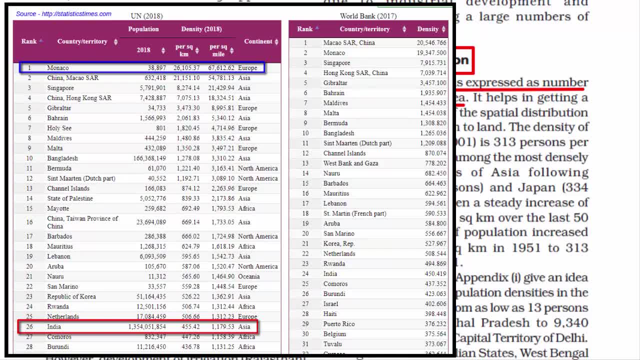 But look at its population density when compared to India. Therefore, it totally depends on number of persons living in per square kilometer of land. By the way, Monaco is densely populated because people are attracted to Monaco by its weather and casino and its glamorous reputation. 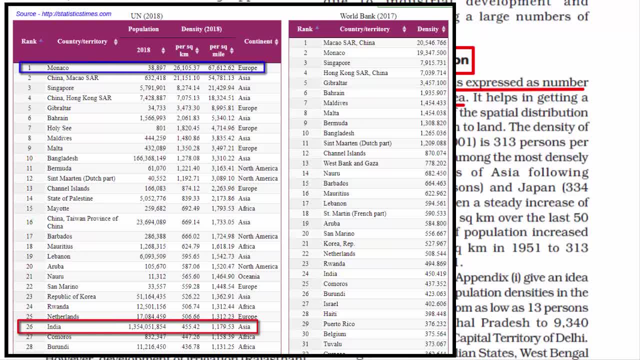 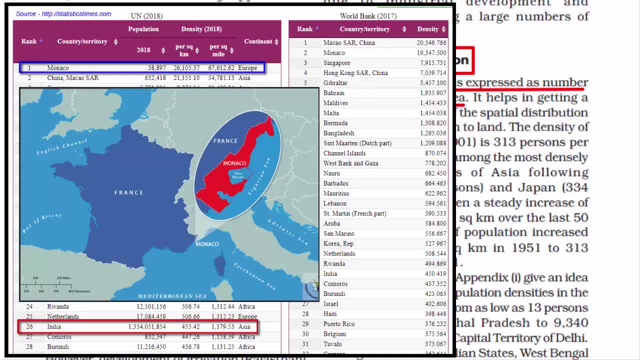 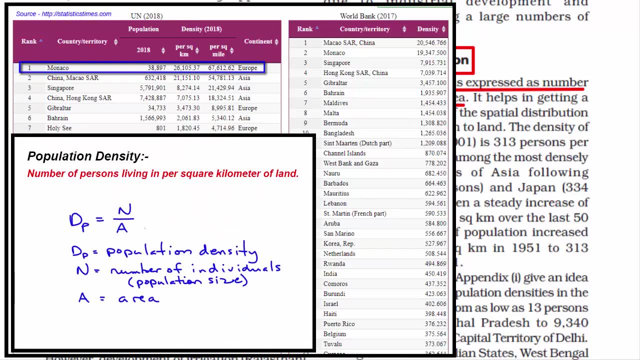 India is the 26th rank. If you look at Monaco, it is a tiny independent city-state on France's Mediterranean coastline. An average person can walk across the width of the country in about an hour, But look at its population density when compared to India. Therefore it 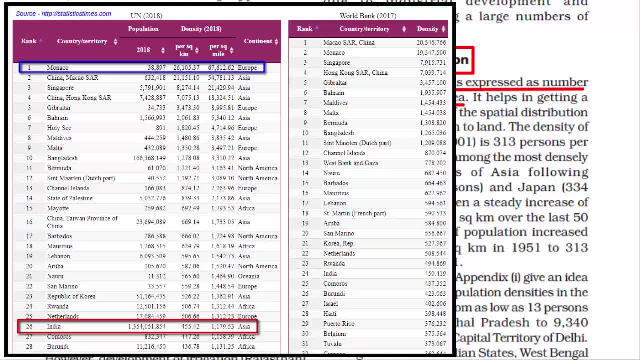 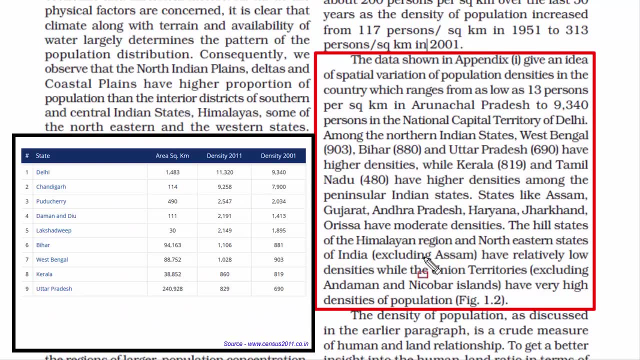 is a noظard, Even 3o-rese ona number of persons living in per square kilometer of land. By the way, Monaco is densely populated because people are attracted to Monaco by its weather, casino and glamorous reputation. Similarly, if you look at the states and union territories in 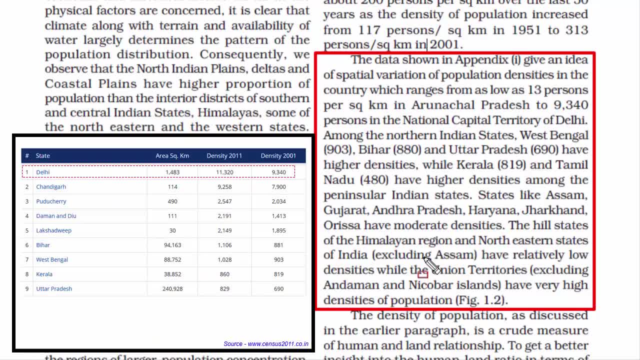 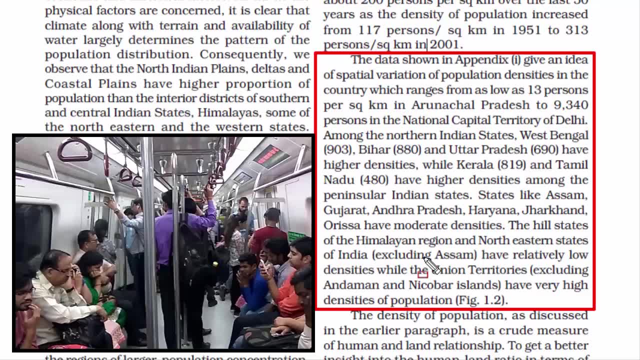 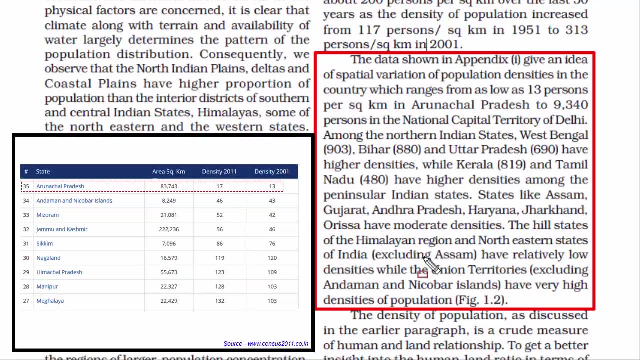 India. Delhi is the most densely populated place in India. Delhi has nothing of its own. People came here and settled. Since it's the capital, people come here for better work. Now, if you look at Arunachal Pradesh, it is the lowest population density state in India. 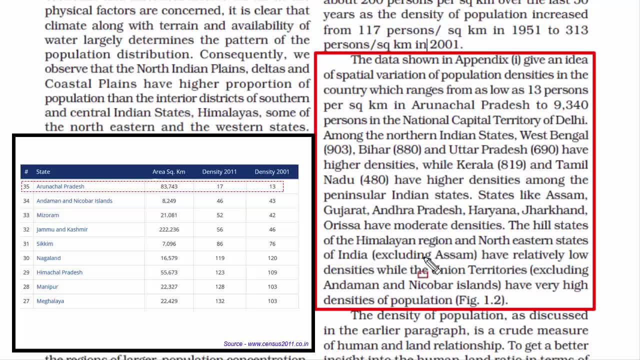 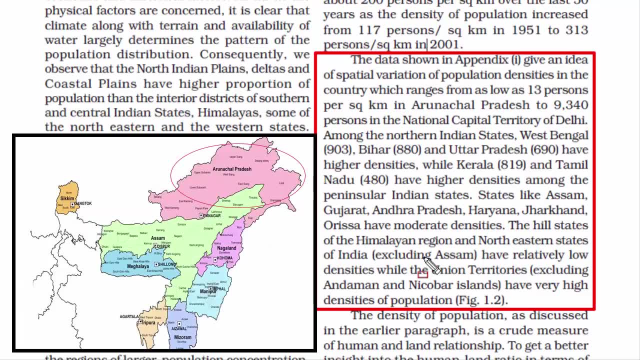 It is around 17% per square kilometer, And the reason behind this is lack of facilities or food, as agriculture is rarely followed there by the people. The geographical terrain is hilly, the weather is cold and rainy, and most of the state is 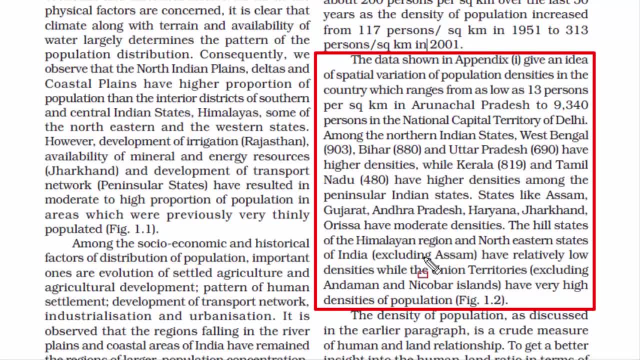 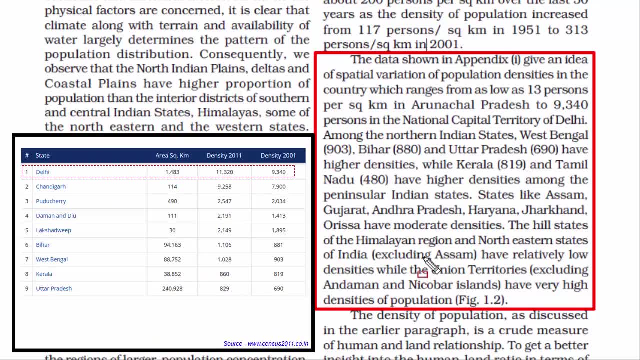 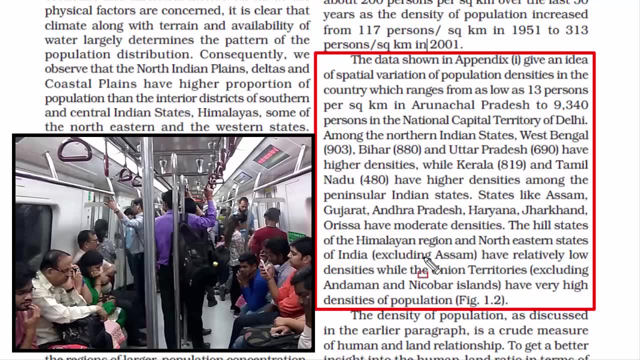 Similarly, if you look at the states and union territories in India, Delhi is the most densely populated place in India. Delhi has nothing of its own. People came here and settled. Since it's the capital. people come here for better work, education and life opportunities. 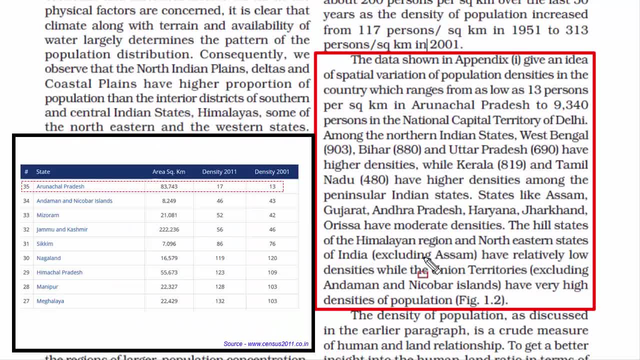 Now, if you look at Arunachal Pradesh, it is the lowest population density state in India- It is around 17 persons per square kilometer- And the reason behind this is lack of facilities or food, as agriculture is rarely followed there by the people. 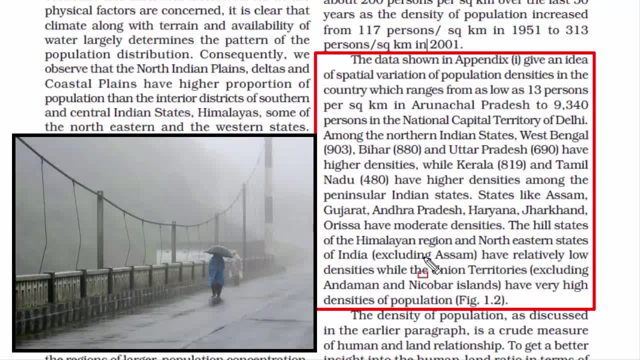 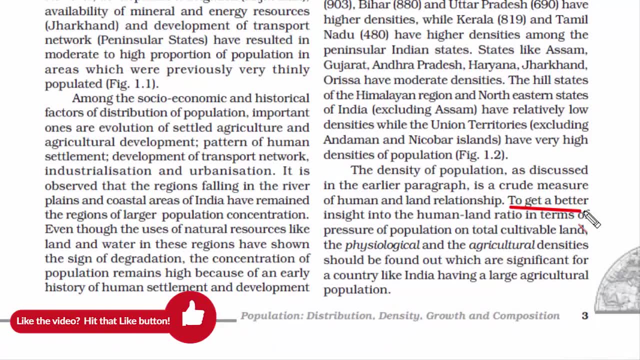 The geographical terrain is hilly, the weather is cold and rainy, and most of the state is covered with thick forests. Now that you know what is population density and how it is calculated, in the similar way we can find out physiological densities and agricultural densities. 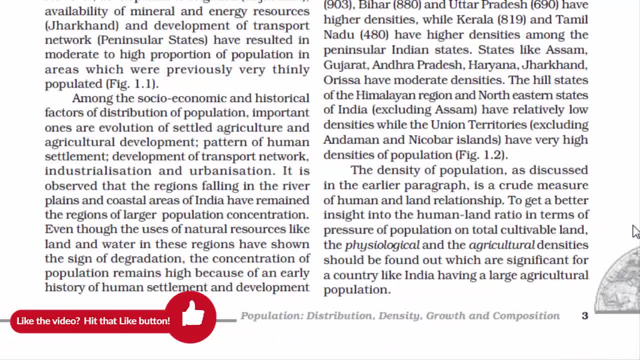 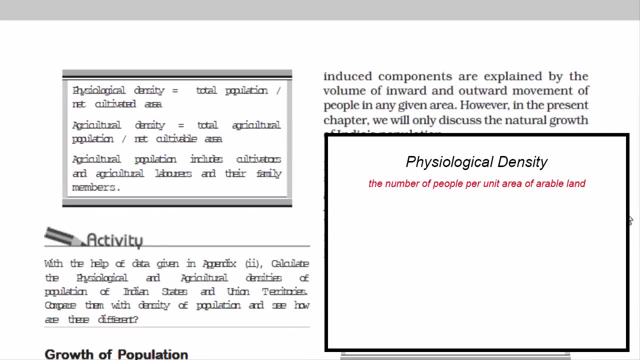 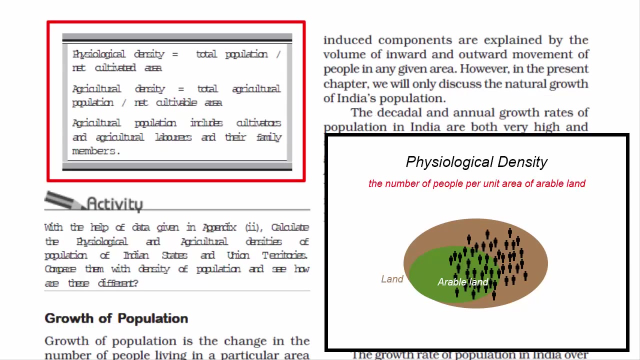 covered with thick forests. Now that you know what is population density and how it is calculated, in the similar way we can find out physiological densities and agricultural densities. So physiological density means the number of people per unit area of arable land. In other words, how many people can be supported through per unit area of agricultural land. 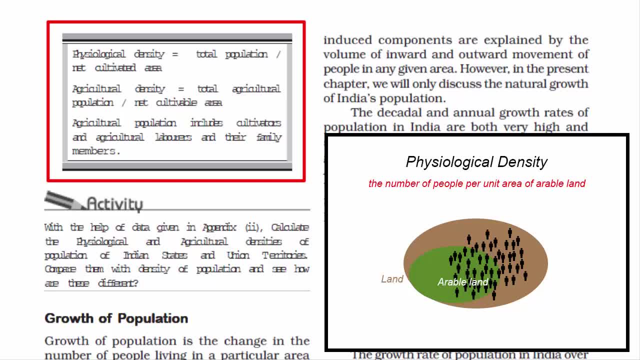 Arable land means the land which is capable of being plowed and used to grow crops, In other words, agricultural land. Now, finding the physiological density is an important data. It can actually show us how many people are being supported by each unit of farmland, and 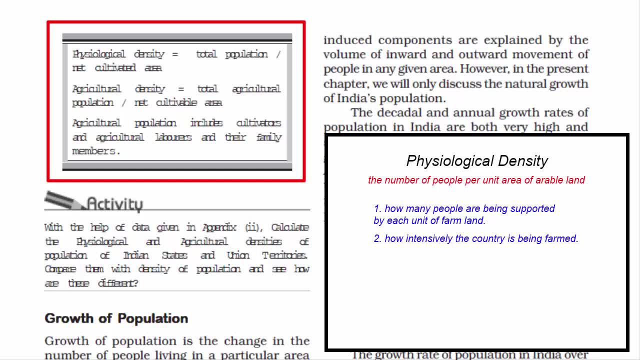 can tell us something about how intensively the country is being farmed and the nation's food producing capability. A higher physiological density suggests that the available agricultural land is being used more and may reach its output limit sooner than a country that has a lower physiological 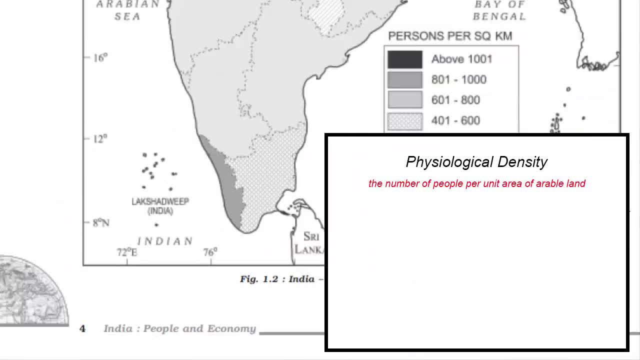 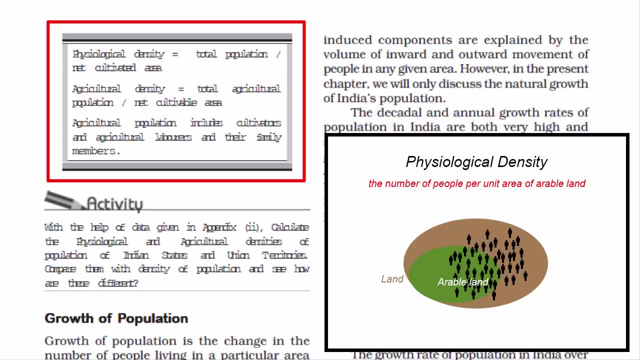 So physiological density means the number of people per unit area of arable land. In other words, how many people can be supported through per unit area of agricultural land. Arable land means the land which is capable of being plowed and used to grow crops. 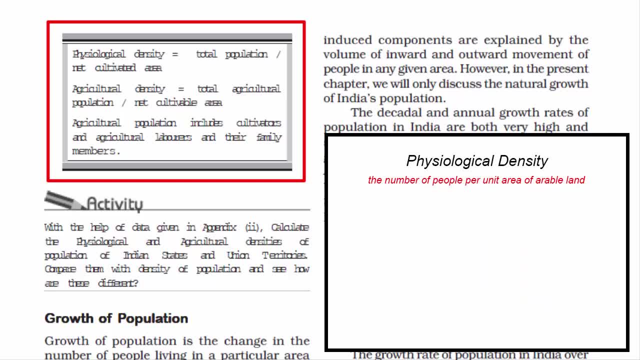 In other words, agricultural land. Now, finding the physiological density is an important data. It can actually show us how many people are being supported by each unit of farmland and can tell us something about how intensively the country is being farmed and the nation's food producing capability. 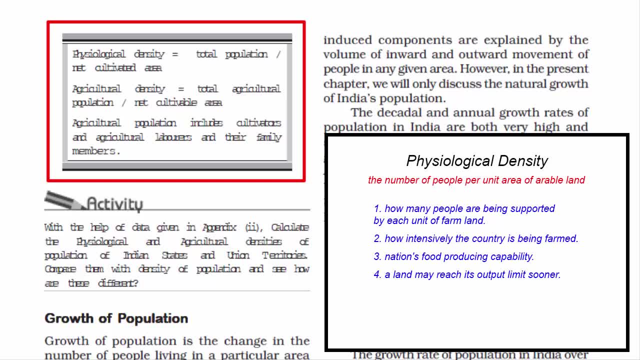 A higher physiological density suggests that the available agricultural land is being used more and may reach its output limit sooner than a country that has a lower physiological density. It can also show us how much of food we can produce in a homeland and how much do we need to import or export. 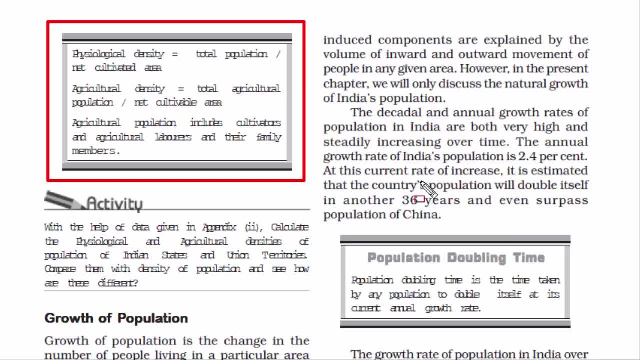 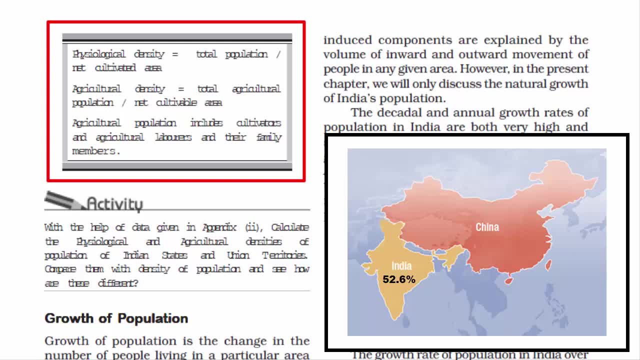 I want you to understand that this is very important. I'll explain with an example. Let's take China and India. India is an agrarian land. Almost half the total land area of India is a good arable land, Whereas that number is only 15% for China. 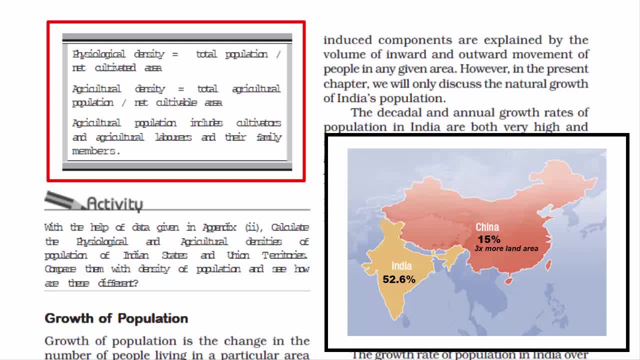 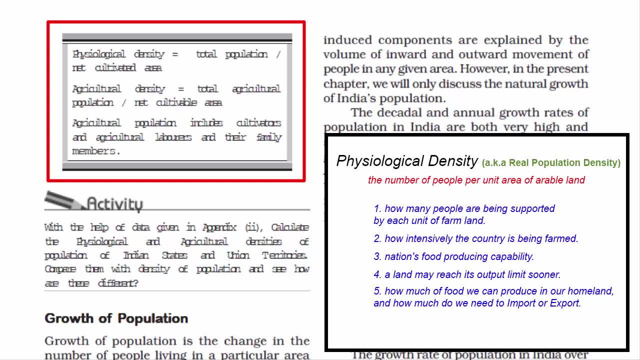 But then if you see China, it is three times larger than India in terms of area, Although China looks bigger on the map. their population density is low, But China's food growing capability is less for its people compared to India. By the way, physiological density is also called as real population density. 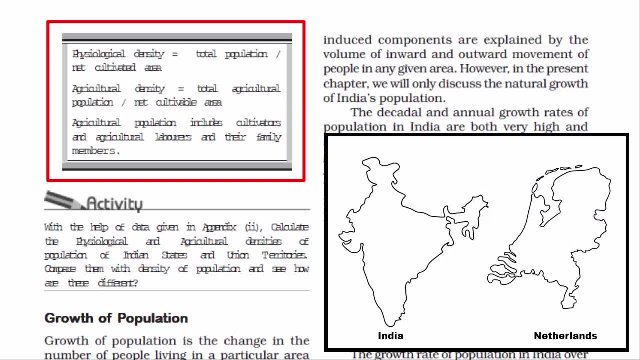 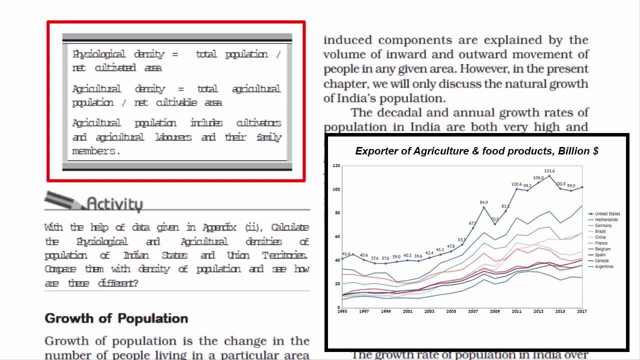 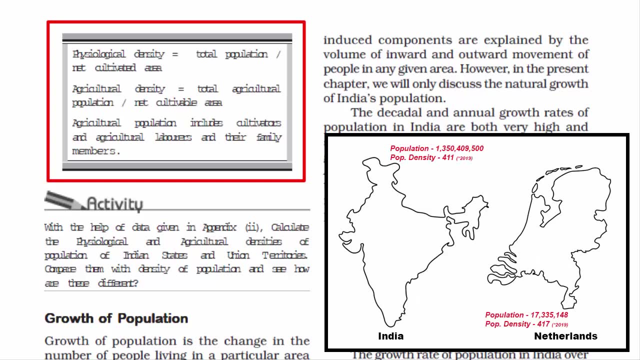 We'll take another example. Let's look at Netherlands and India. Netherlands is second or third biggest agricultural exporter in the world, And have you seen the area size of Netherlands? Netherlands is about 79 times smaller than India, But the population density is almost similar to India. 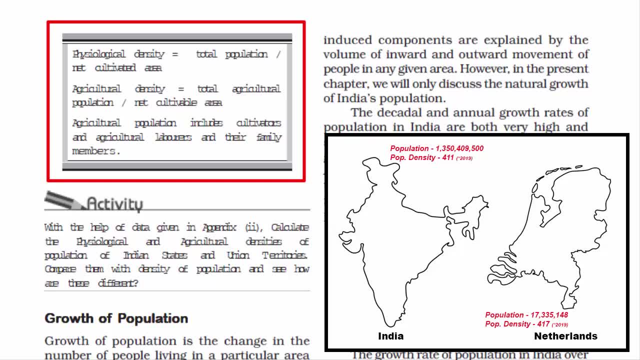 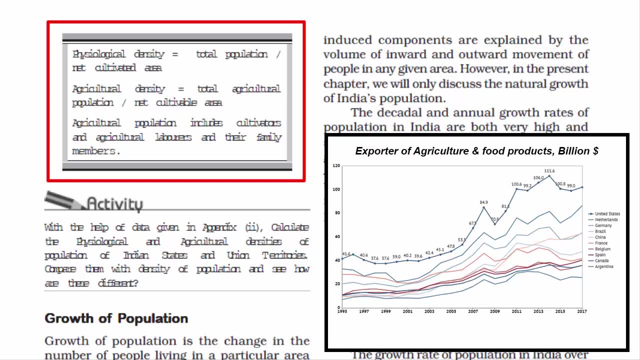 That means it is one of the crowded places on earth, just like India. Now the question is: how is it that a country like Netherlands, which is equally overpopulated like India, has succeeded much better economically and socially, And they are also the second or third biggest agricultural exporter in the world? 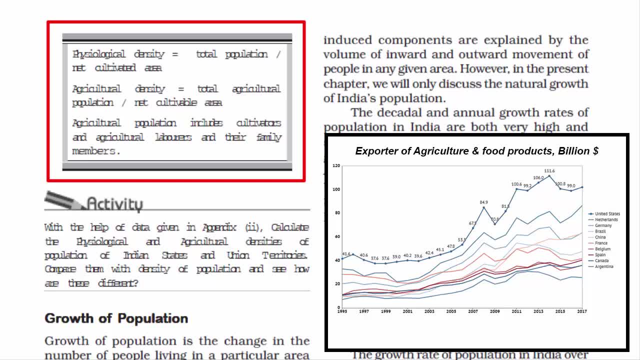 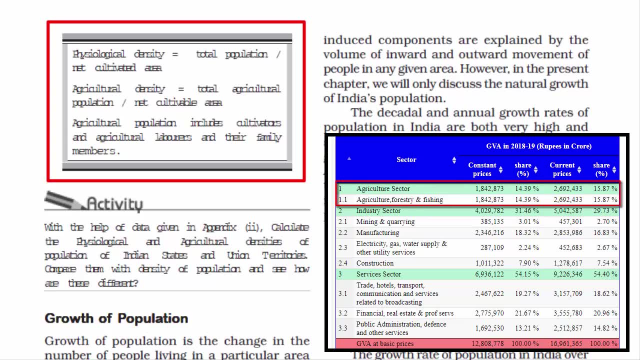 That means they are not just meeting the food demands of their own people, but they are also able to export the excess. On the other hand, India's agricultural condition is in a poor state And, if you see, we have been always told that it is because of the overpopulation. 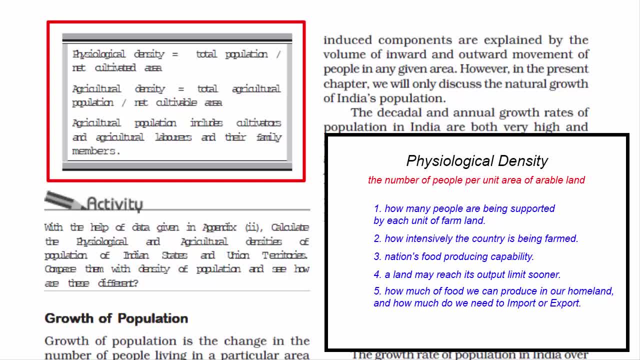 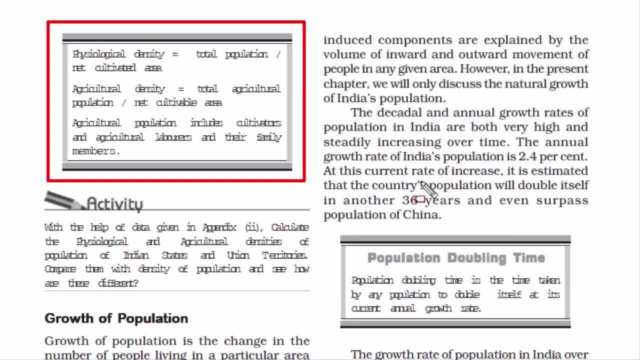 density. It can also show us How much of food we can produce in a homeland, and how much do we need to import or export. I want you to understand that this is very important. I'll explain with an example. Let's take China and India. 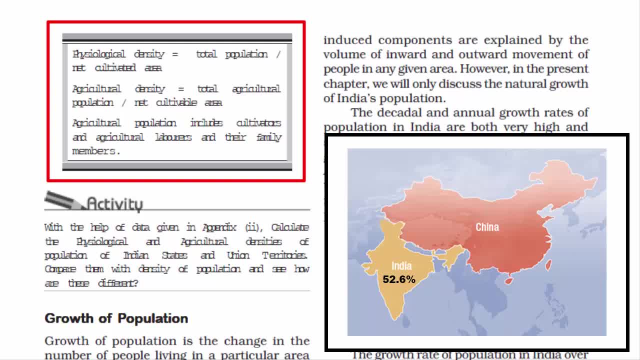 Now India is an agrarian land. Almost half the total land area of India is a good arable land, whereas that number is only 15% for China. But then if you see China, it is 3 times larger than India in terms of area. 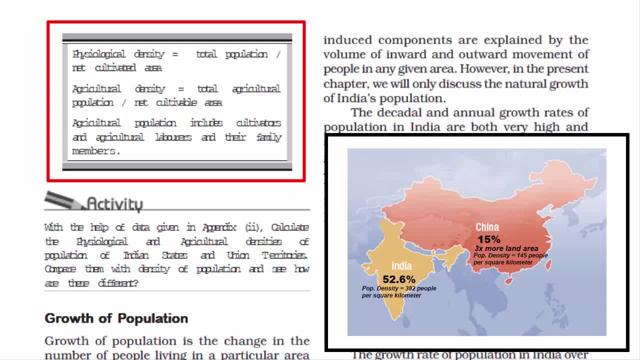 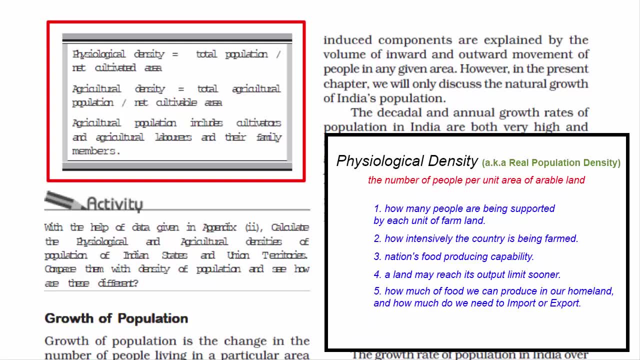 Although China looks bigger on the map, Their population density is low. But China's food growing capability is less for its people compared to India. By the way, physiological density is also called as real population density. We'll take another example. Let's look at Netherlands and India. 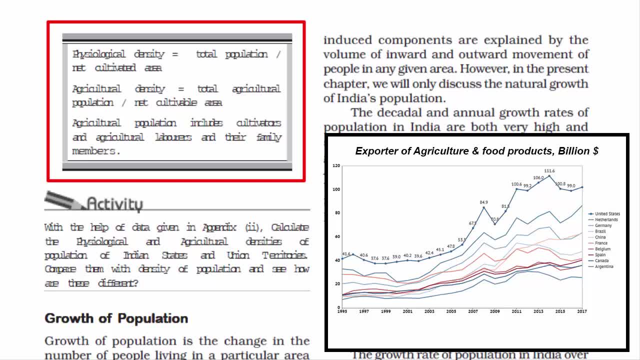 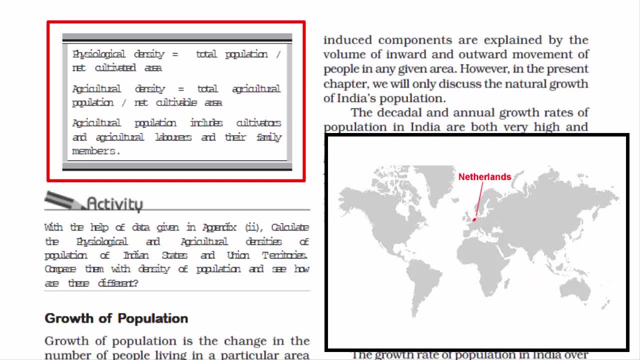 Netherlands is second or third biggest agricultural exporter in the world. And have you seen the area size of Netherlands? Netherlands is about 79 times smaller than India, But the population density is almost similar to India. That means it is one of the crowded places on earth, just like India. 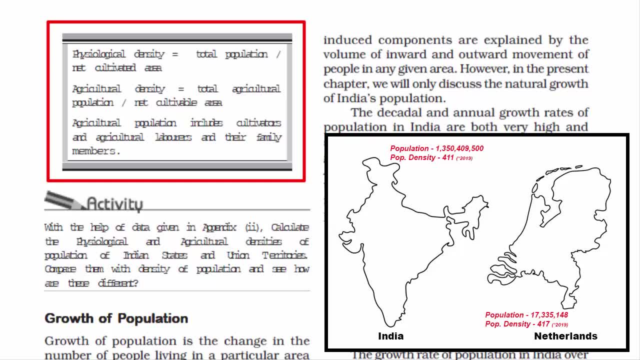 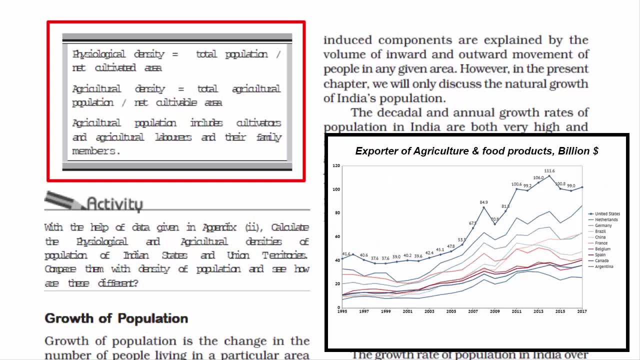 Now the question is: how is it that a country like Netherlands, which is equally overpopulated like India, has succeeded much better economically and socially? And they are also the second or third biggest agricultural exporter in the world. That means they are not just meeting the food demands of their own people, but they are 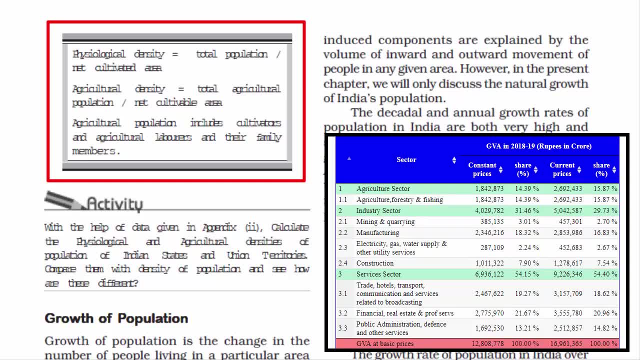 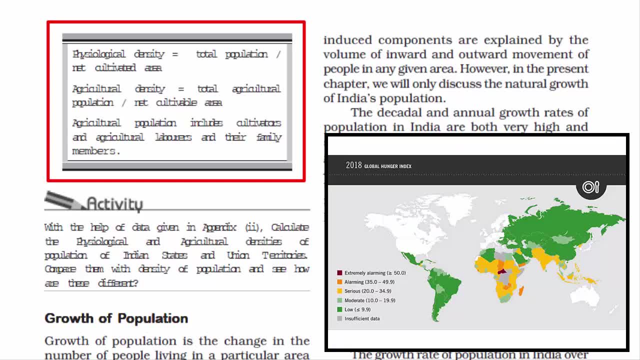 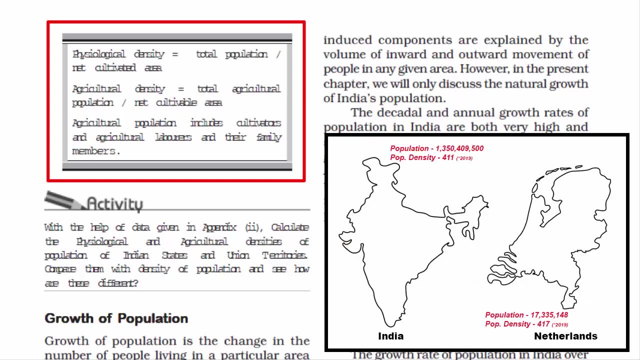 also able to export the excess. On the other hand, India's agricultural condition is in a poor state And, if you see, we have been always told that it is because of the overpopulation. India is facing food shortage. Now, looking at both the examples, we can clearly stop blaming the population. 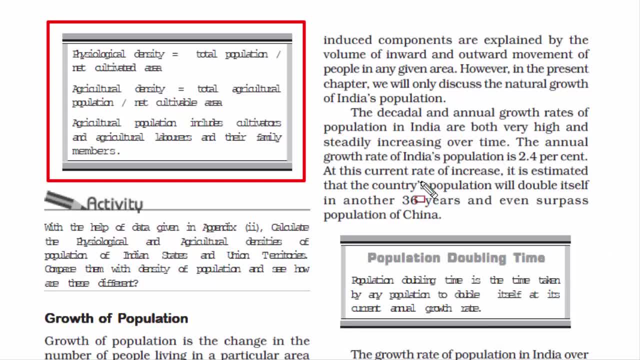 There are many countries which have less agricultural land area than India, and they are also equally crowded like India, But they have a better standard of living than India. So clearly, population cannot be blamed for it. Rather, it has everything to do with our misplaced economic policies and poor governance. 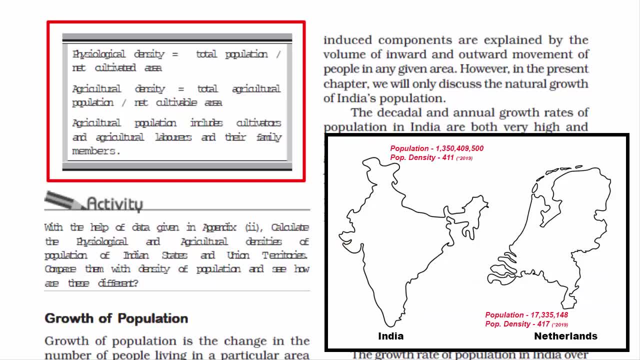 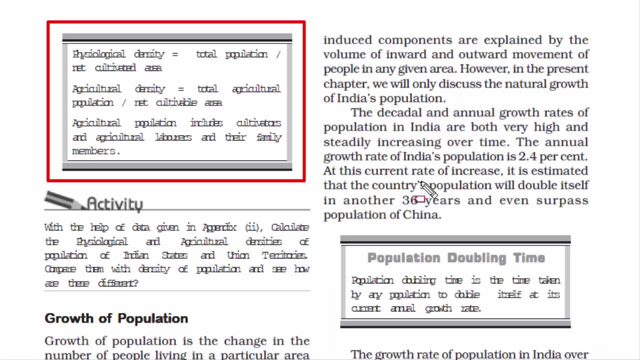 India is facing food shortage. Now, looking at both the examples, we can clearly stop blaming the population. There are many countries which have less agricultural land area than India, And they are also equally crowded like India, But they have a better standard of living than India. 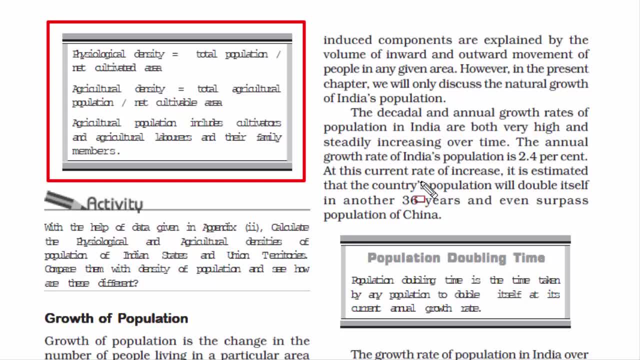 So clearly population cannot be blamed for it. Rather, it has everything to do with our misplaced economic policies and poor governance. So this kind of analysis can be made if we get to know the physiological density of a country. There is another term called agricultural density. 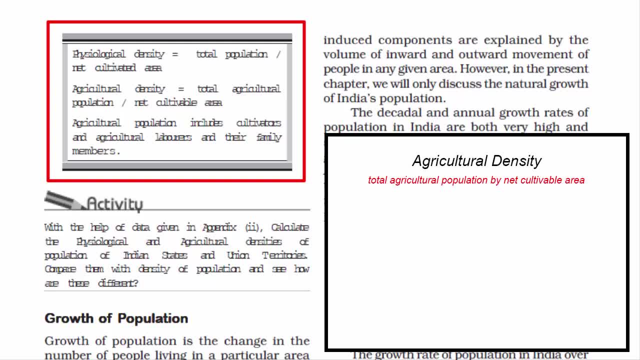 It means total agricultural population by net cultivable area. Now, what do we mean by agricultural population? It includes farmers and their family members. That means number of farmers in a particular region, divided by the area of farmland. Try to understand this carefully. 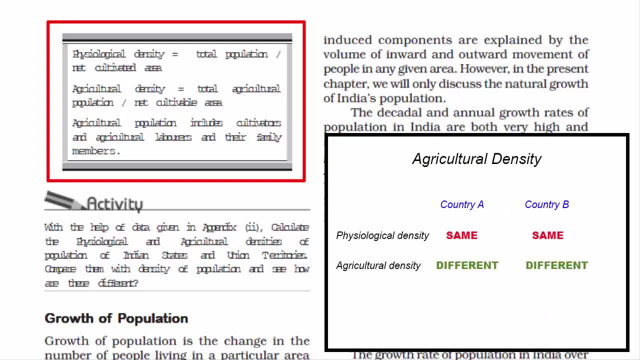 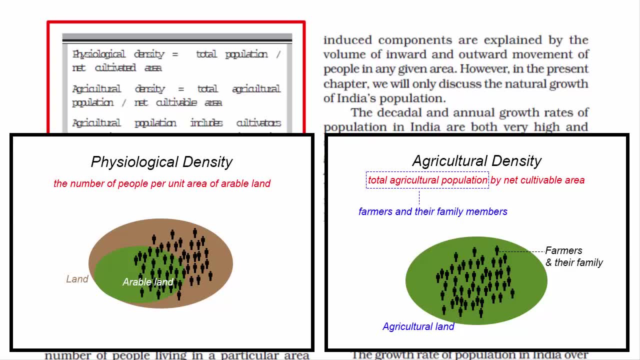 Two countries can have similar physiological densities but different agricultural density. You simply take the physiological and agricultural densities of countries and compare them. It will give you a better insight into the human to land ratio in terms of pressure of population on total cultivable land. 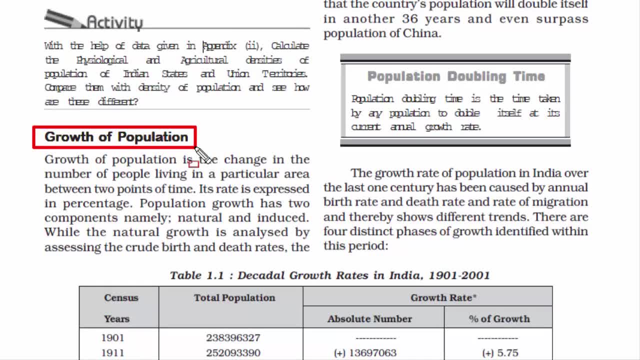 Let's go to the next topic: growth of population. Now, population growth or growth of population is the same, So by looking at the topic's name, you can easily figure out that it's talking about the change in the number of people living in a particular area between two points of time. 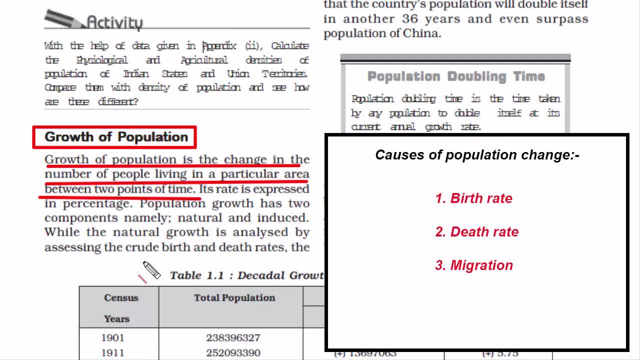 There are three main causes of population change. They are birth, death and migration. Births are usually measured using the birth rate, That is number of births divided by total population multiplied by thousand. Now, deaths are usually measured using the death rate, That is, number of deaths divided by total population multiplied by thousand. 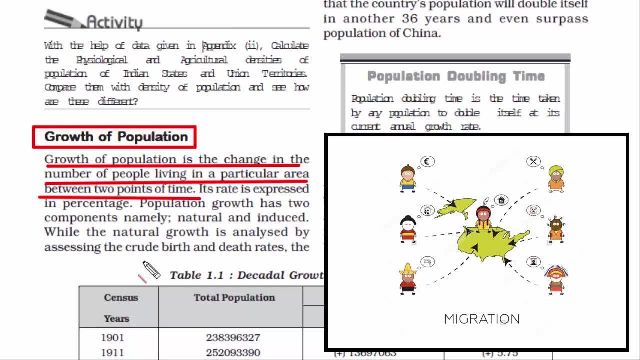 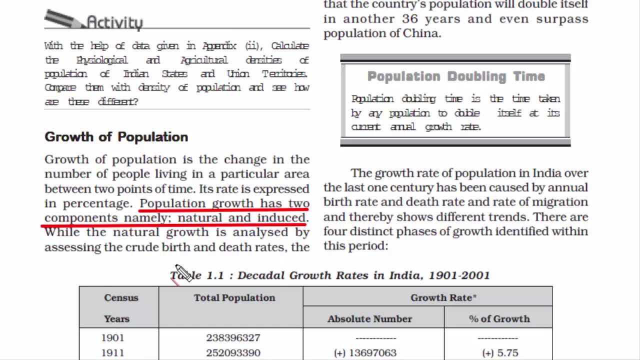 And migration is the movement of people in and out of an area. Now, here it says. population growth has two components: natural and induced. Births and deaths are natural causes of population change. The difference between the birth rate and the death rate of a country or place is called the natural increase. 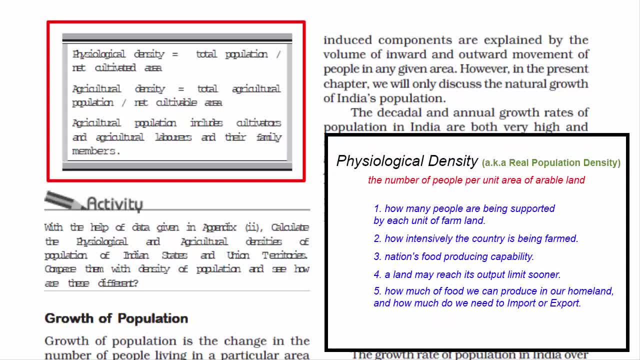 So this kind of analysis can be made if we get to know the physiological density of a country. There is another term called agricultural density. It means total agricultural population by net cultivable area. Now, what do we mean by agricultural population? It includes farmers and their family members. 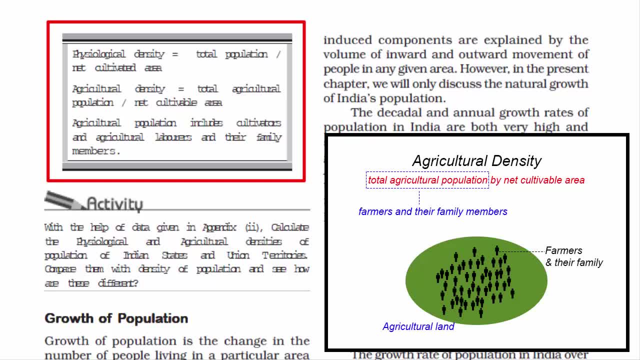 That means number of farmers in a particular region divided by the area of farm area. That means the number of farmers in a particular region divided by the area of farm area. That means the number of farmers in a particular region divided by the area of farm area. 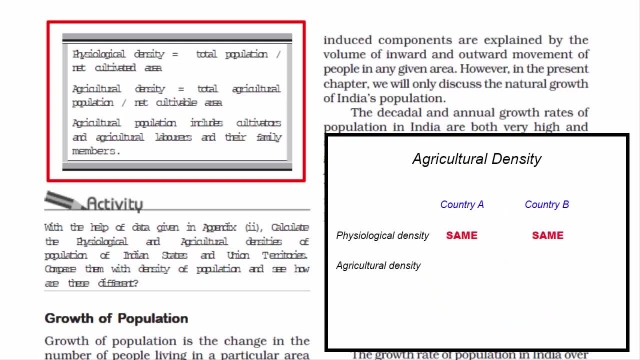 That means the number of farmers in a particular region, divided by the area of farm land. Try to understand this carefully. Two countries can have similar physiological densities but different agricultural density. Try to understand this carefully. Two countries can have similar physiological densities but different agricultural density. 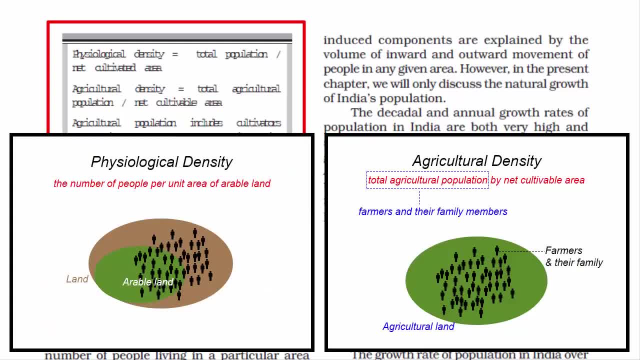 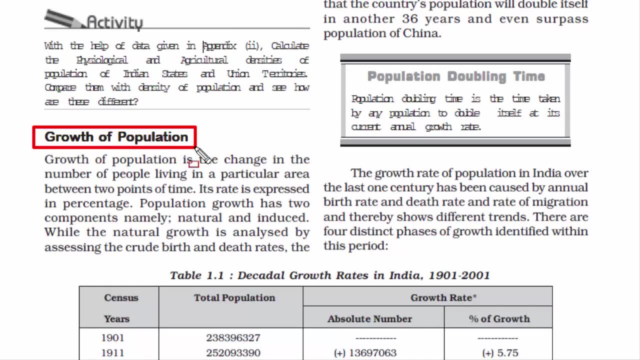 You simply take the physiological and agricultural densities of countries and compare them. It will give you a better insight into the human to land ratio in terms of pressure of population on total cultivable land. Lets go to the next topic: growth of population. Now, population growth or growth of population is the same type of population as the growth of the population, But only if the population was more or less than the soil size. So the next topic is a chemical advantage. where land is sandwiched between the land, land and land, The man or woman needs to plant, plant land on farms and the man yields the land. 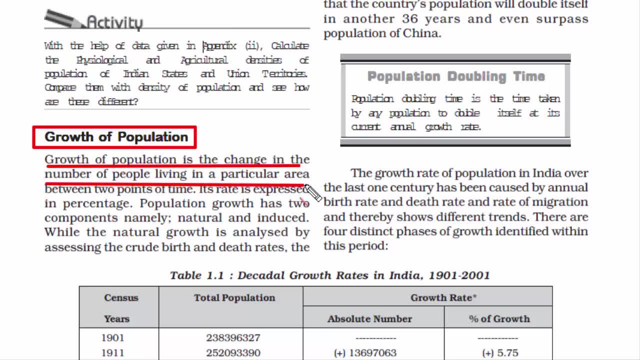 The man or woman needs to own the land, it's the same. So by looking at the topic's name, you can easily figure out that it's talking about the change in the number of people living in a particular area between two points of time. There are three main causes of population change. They are birth, death. 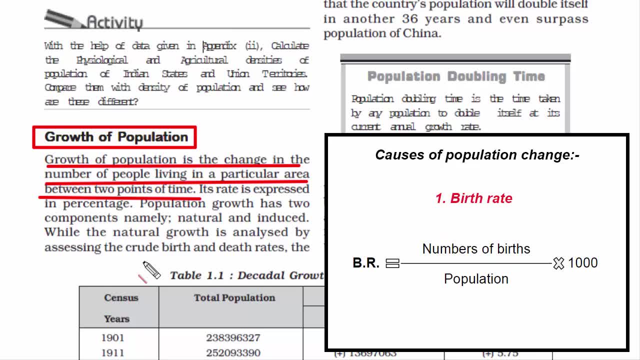 and migration. Births are usually measured using the birth rate, that is, number of births divided by total population multiplied by 1000.. Now, deaths are usually measured using the death rate, that is, number of deaths divided by total population multiplied by 1000.. And 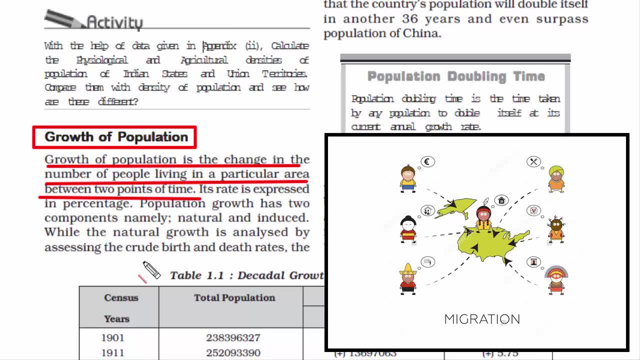 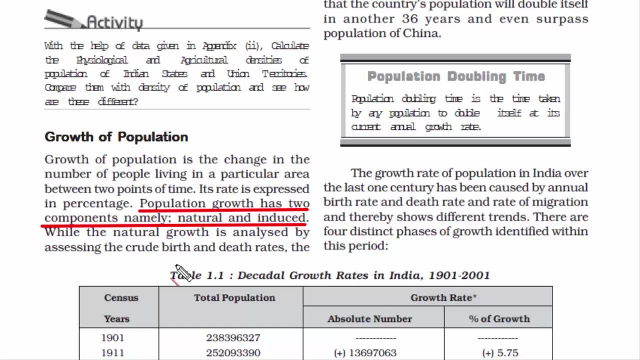 migration is the movement of people in and out of an area. Now here it says. population growth has two components: natural and induced. Births and deaths are natural causes of population change. The difference between the birth rate and the death rate of a country or place is 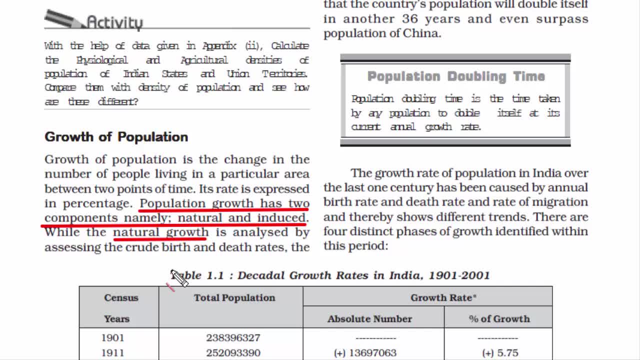 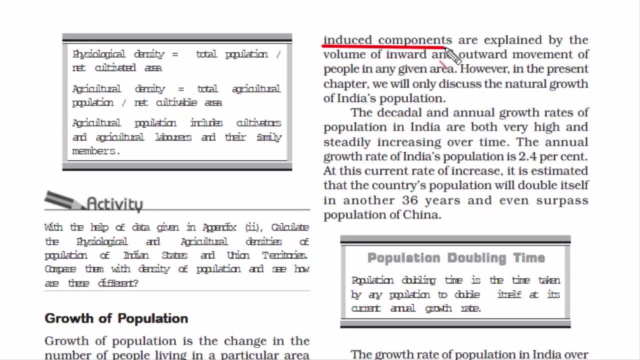 called the natural increase. The natural increase is calculated by subtracting the death rate from the birth rate. Now, if you look at induced component, it is explained by the volume of inward and outward movement of people in any given area, meaning how many people have moved in and out of a 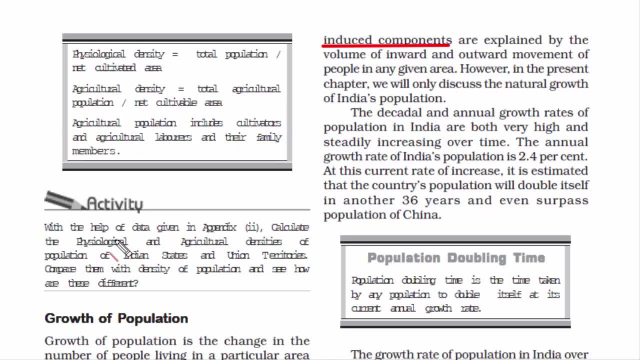 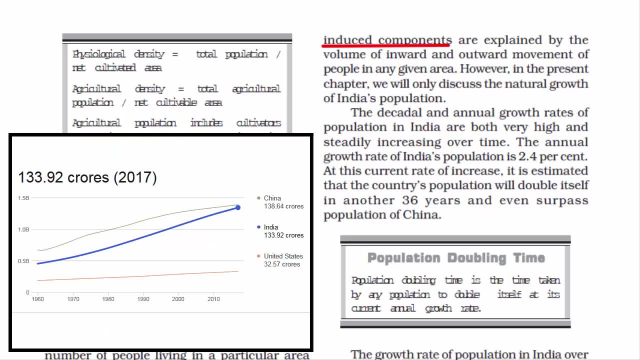 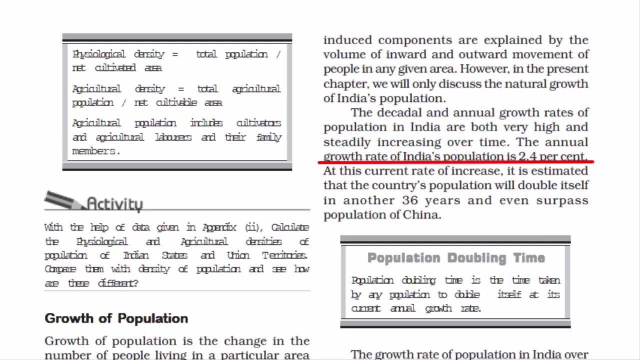 particular place, But in this chapter we will discuss only about natural growth of India's population. We all know that the population of India is very high. The country has doubled in size in just 40 years. Here it says the annual growth rate of India's population is 2.4%. 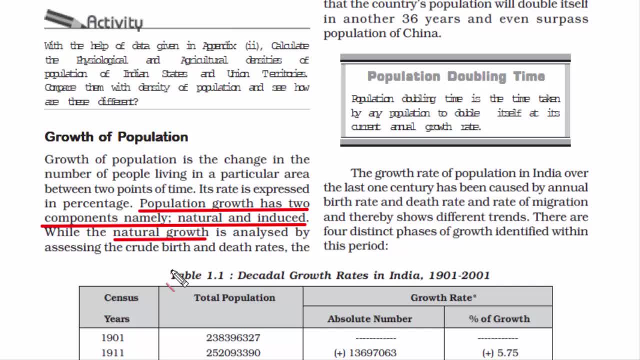 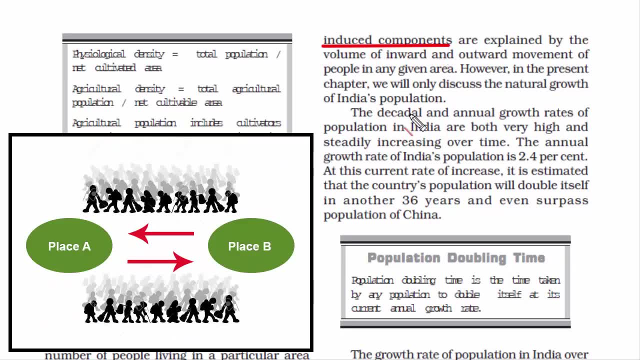 The natural increase is calculated by subtracting the death rate from the birth rate. Now, if you look at induced component, it is explained by the volume of inward and outward movement of people in any given area, Meaning how many people have moved in and out of a particular place. 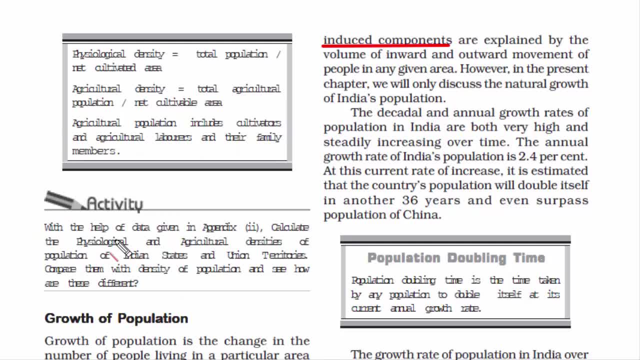 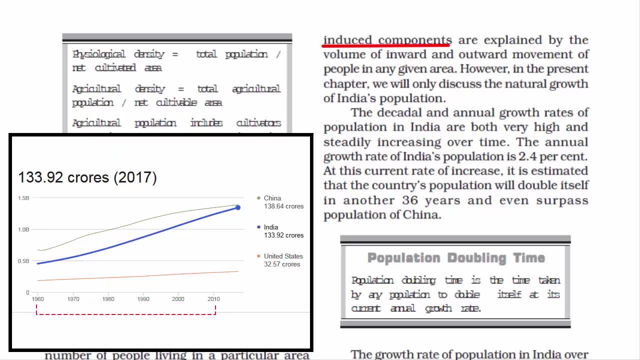 But in this chapter we will discuss only about natural growth of India's population. We all know that the population of India is very high. The country has doubled in size in just 40 years. Here it says the annual growth rate of India's population is 2.4%. 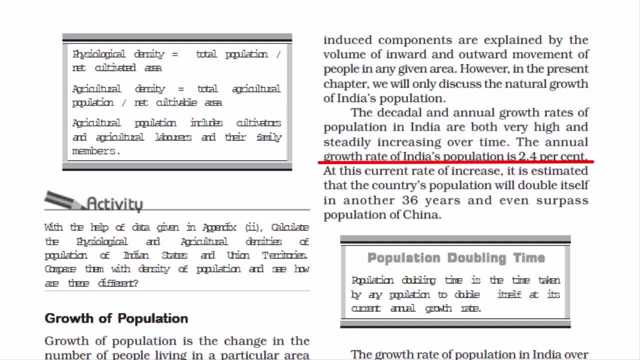 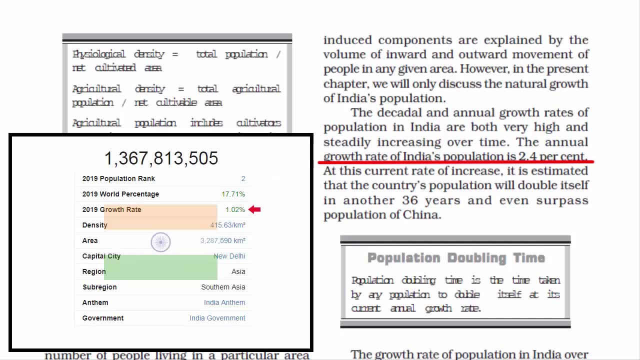 Since this book was published in 2005 or something, so the present count is around 1.02%. This count is between 2010 and 2019.. If you see China's annual population growth, it is around 0.6%. 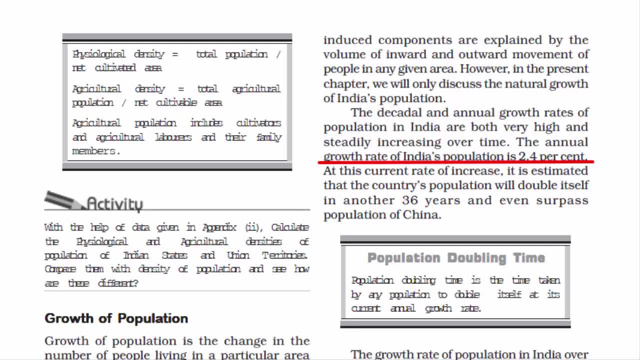 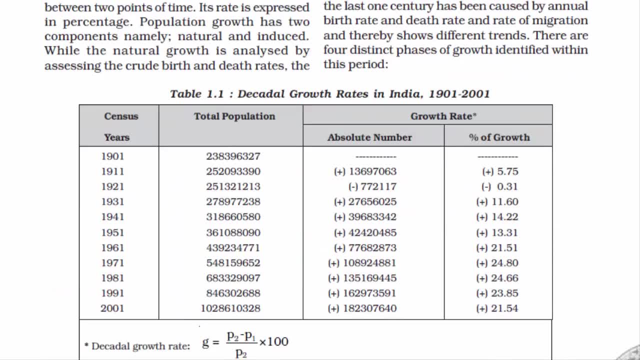 By looking at our population growth rate. it is estimated that India will surpass China as the world's most populated country in the next couple of decades. Now have a look at this table. It shows the population growth rate of India for every 10 years. 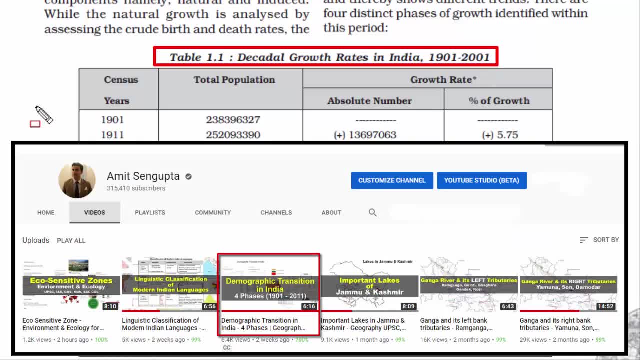 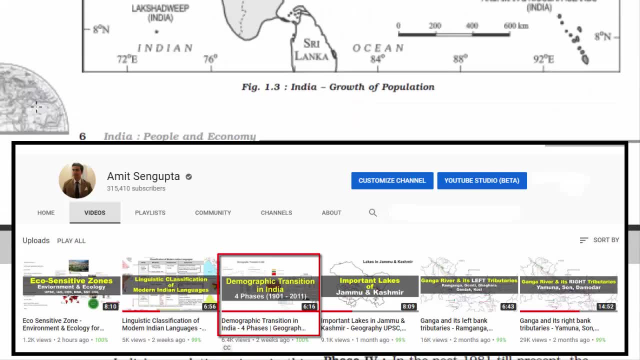 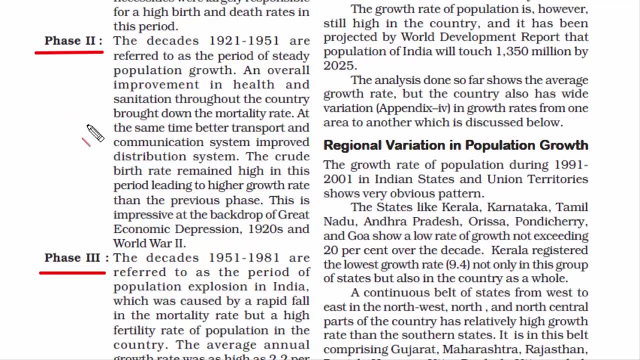 I have made a separate video, especially on this table, explaining different phases of India's population growth. I would recommend you watch that video because this topic requires some time. hence I chose to make a separate video on it. I put the link in the description, or you can simply search for demographic transition in India and you will get it. 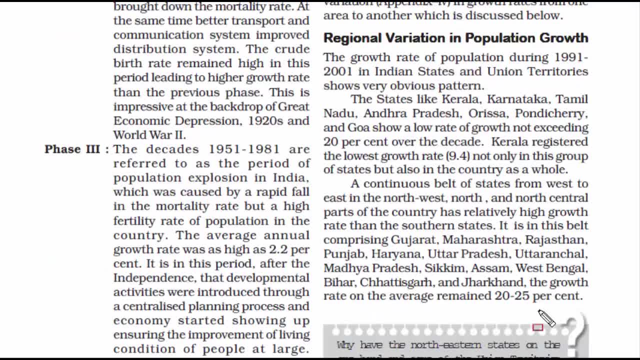 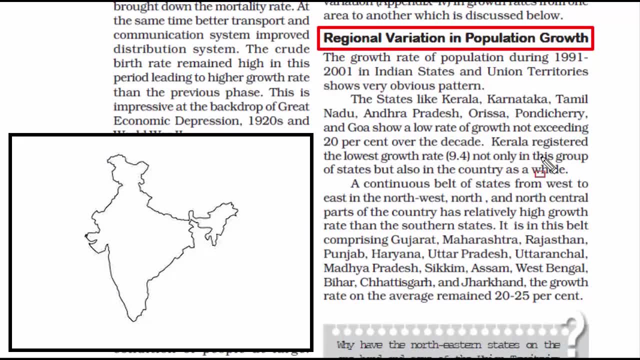 So please watch that video and you will get this topic. The next topic is regional variation in population growth. So far, we have read about the entire country's population growth, But a country comprises of small regions- right That we call as states. 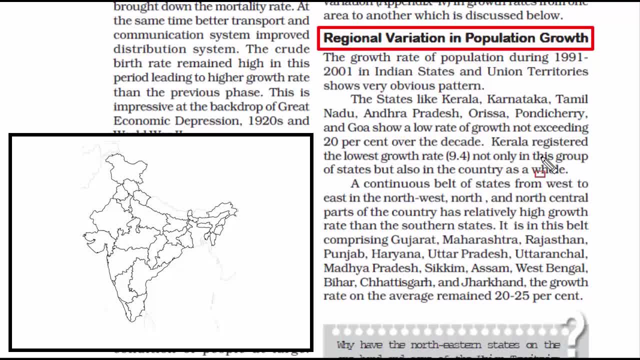 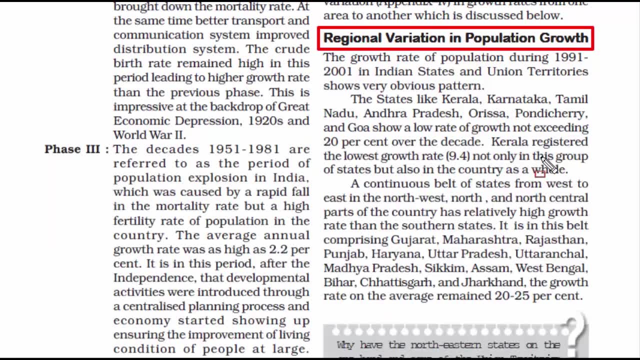 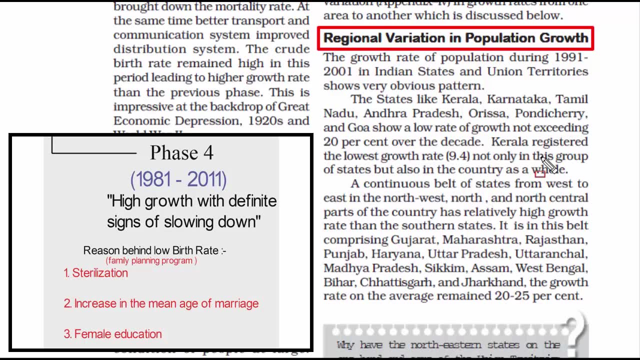 Now we will learn about the population growth within states and see if there is any variation or pattern. So, moments back, I asked you to watch a video that explains different phases of India's population growth, And I hope you have watched that video. So, in that, the final phase, which is from 1981 to 2011, which is also referred to as the period of high growth, with definite signs of slowing down, 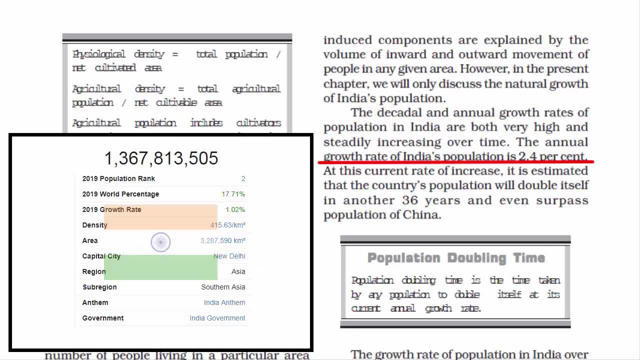 Since this book was published in 2005 or something, so the present count is around 1.02%. This count is between 2010 and 2019.. If you see China's annual population growth, it is around 0.6%. 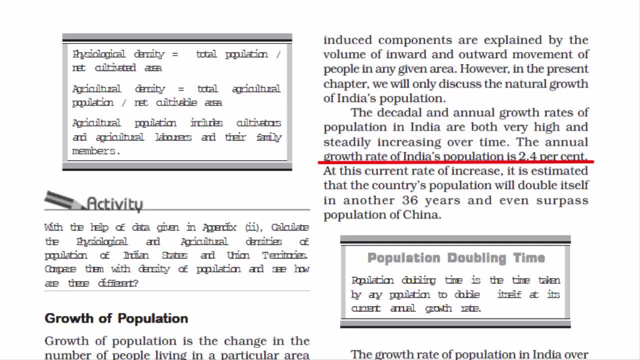 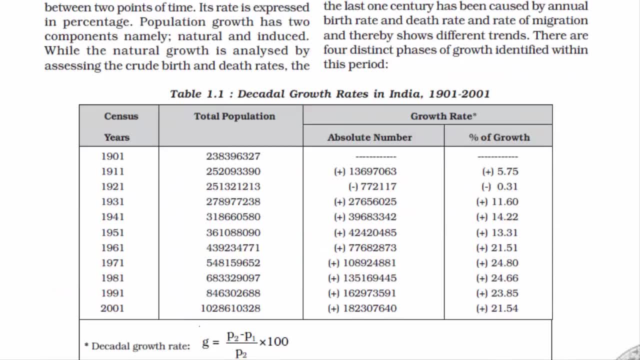 By looking at our population growth rate. it is estimated that India will surpass China as the world's most populated country in the next couple of decades. Now have a look at this table. It shows the population growth rate of India for every 10 years. 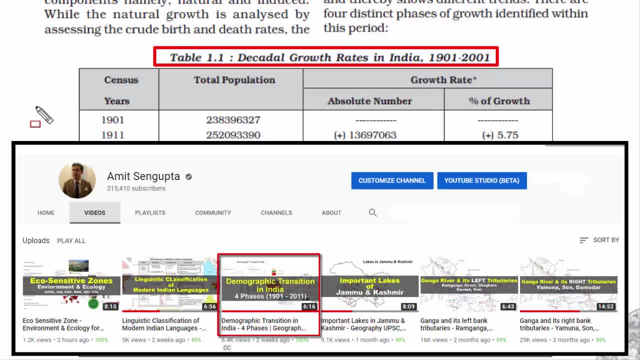 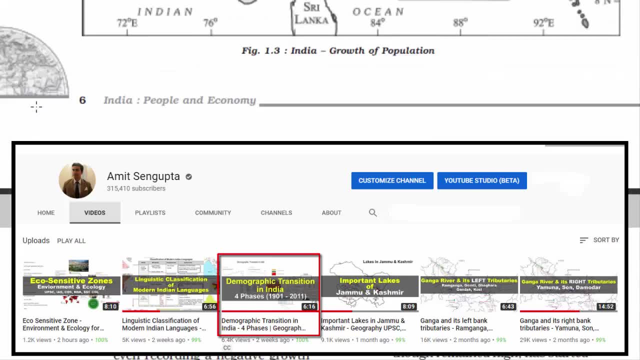 I have made a separate video, especially on this table, explaining different phases of India's population growth. I would recommend you watch that video because this topic requires some time. hence I chose to make a separate video on it. I put the link in the description or you can simply search for demographic transition in. 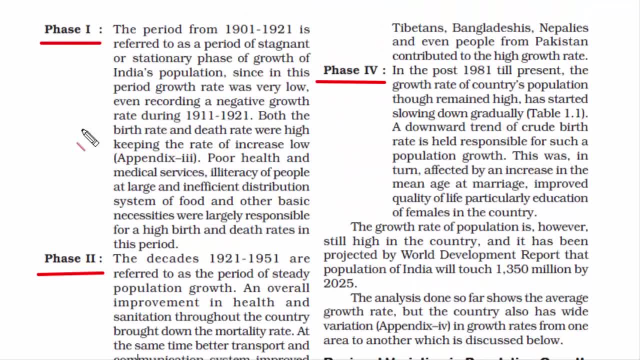 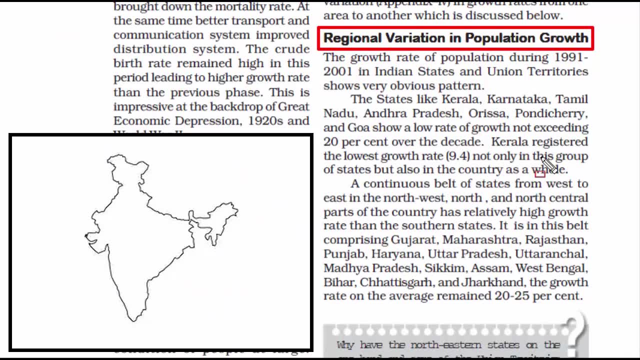 India and you will get it. So please watch that video and you will get this topic. The next topic is regional growth rate. Let's start with the regional growth rate. Regional variation in population growth. So far we have read about the entire country's population growth. 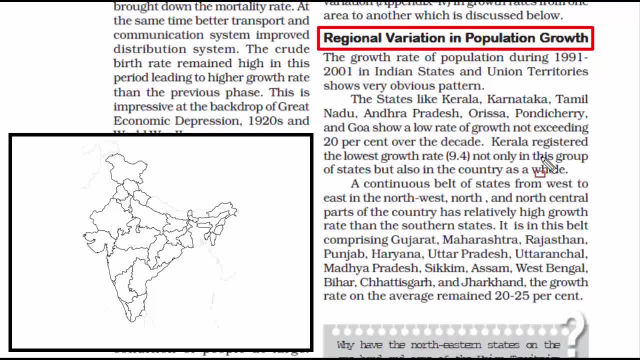 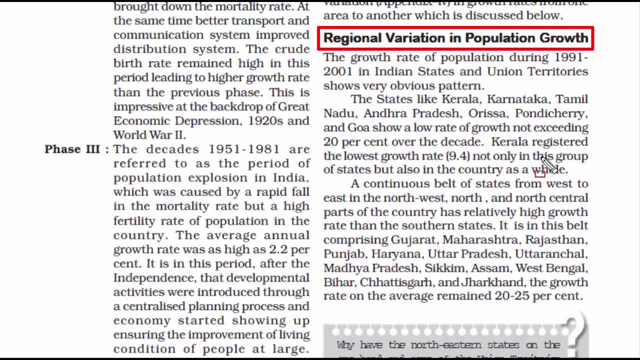 But a country comprises of small regions- right, That we call as states. Now we will learn about the population growth within states and see if there is any variation or pattern. So, moments back, I asked you to watch a video that explains different phases of India's. 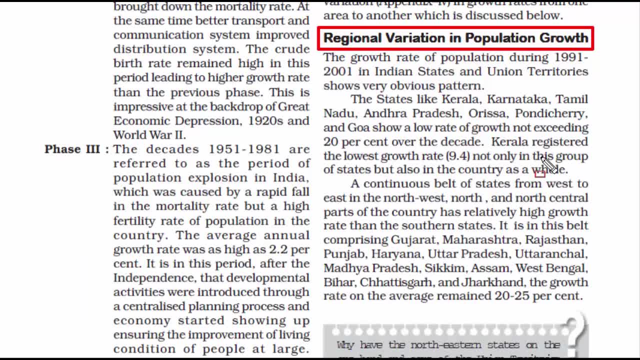 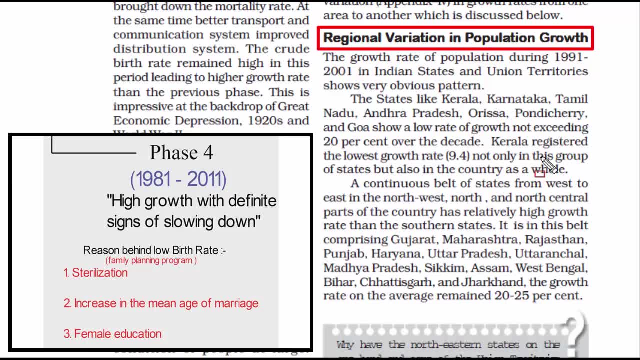 population growth And I hope you have watched that video. So, in that, the final phase, which is from 1981 to 2011.. Which is also referred to as the period of high growth, with definite signs of slowing down, And the reason was because of the decline in birth rate. 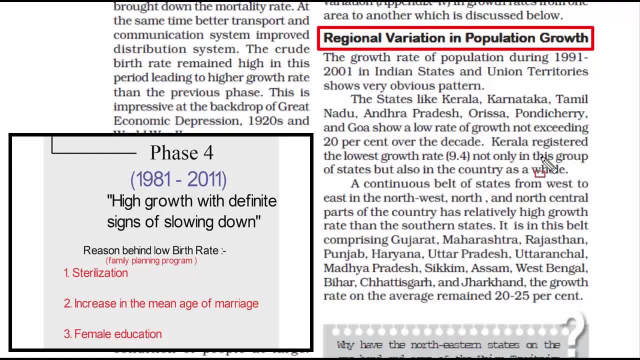 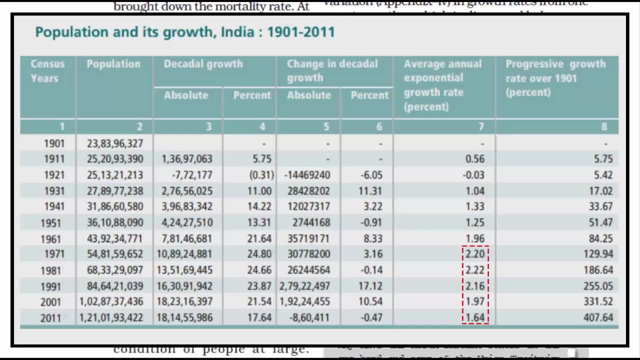 And the reason was because of the decline in birth rate. Plus, I also gave you the statistics: The population growth rate declined from 2.2% in 1971 to 2.14% by 1991.. And further to 1.95% in 2001 and finally to 1.64% in 2011.. 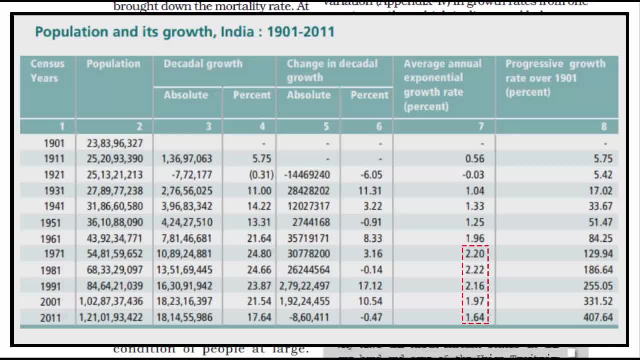 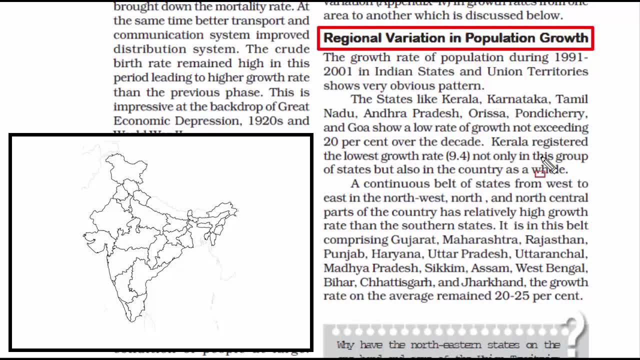 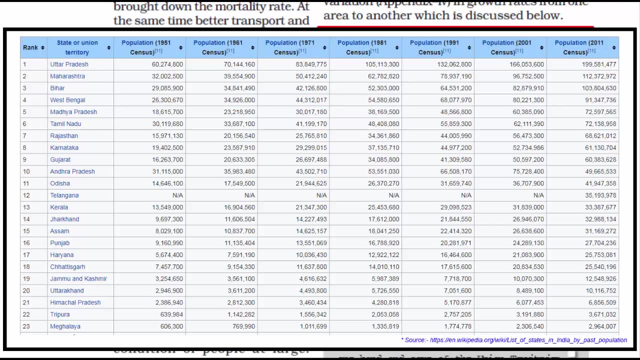 So clearly. you see, it was from 1991 the growth rate started slightly going down. So when we say regional variation, obviously we are talking about the Indian states and the union territories. So what we need to do is we need to look at the growth rate of population of the Indian states and union territories from 1991.. 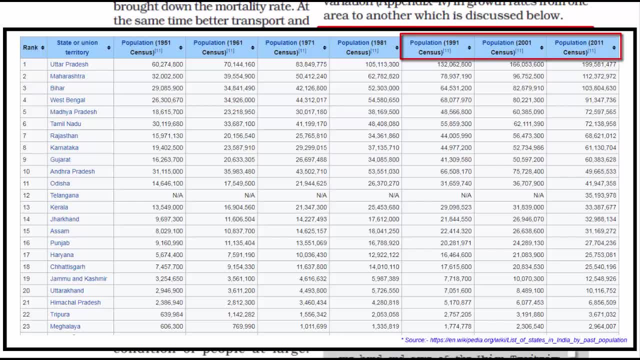 That's how you will notice a pattern as to which states or the regions were having less population or more population. The government does all kinds of investigation because this is how you can find out whether or not there is any correlation between a region and the population growth. 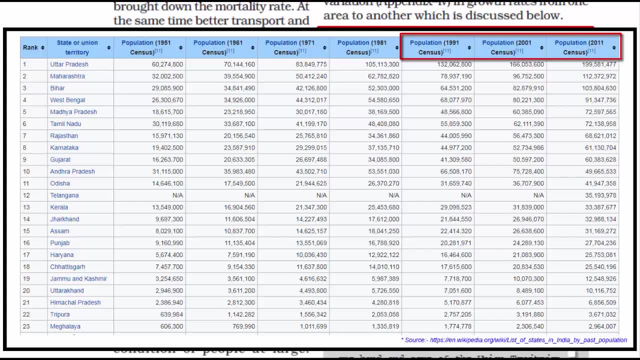 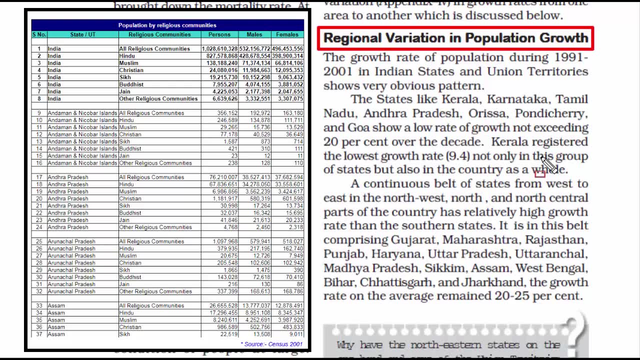 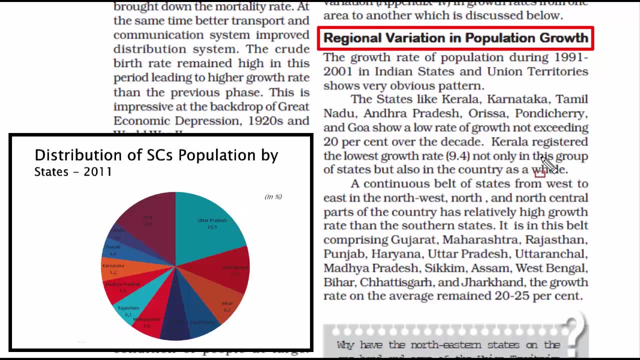 Because over the years we know the distribution pattern of our country's population, Like in a particular state, where the so and so communities live. which region is dominated by which community? Similarly, where do minorities reside? where do tribal communities live? So all kinds of information is available with the government regarding our population. 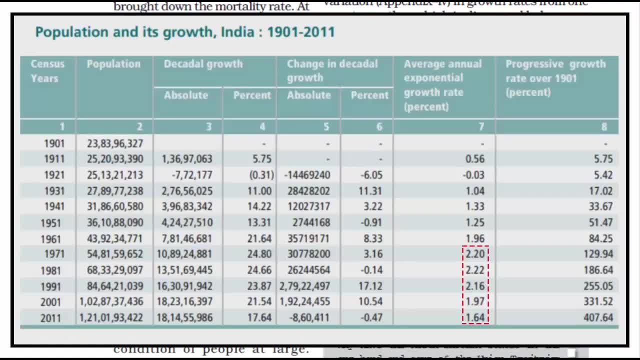 Plus, I also gave you the statistics. The population growth rate declined from 2.2% in 1971 to 2.14% by 1991.. And further to 1.95% in 2001 and finally to 1.64% in 2011.. 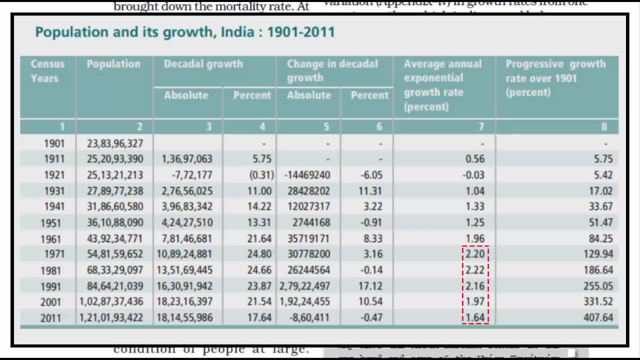 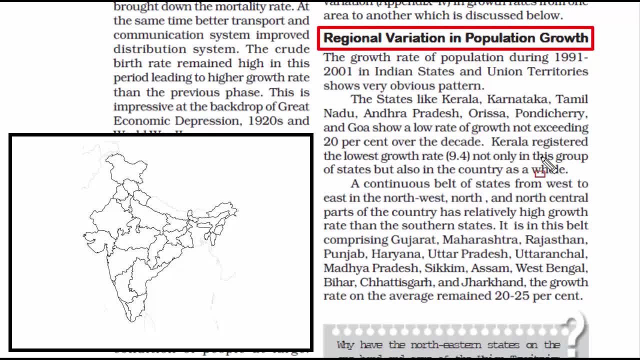 So clearly. you see it was from 1991.. The growth rate started slightly going down. So when we say regional variation, obviously we are talking about the Indian states and the union territories. So what we need to do is we need to look at the growth rate of population of the Indian. 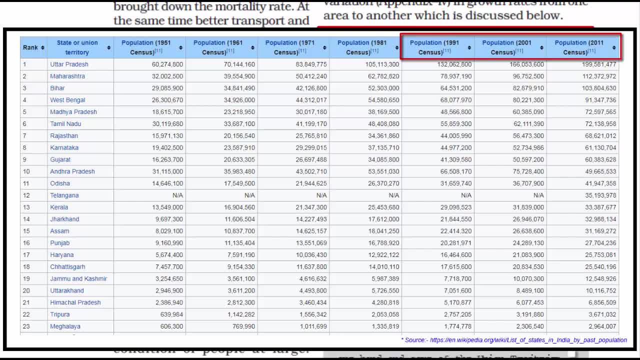 states and union territories from 1991.. That's how you will notice a pattern as to which states or the regions were having less population or more population. The government does all kinds of investigation because this is how you can find out whether or not there is any correlation between a region and the population growth. 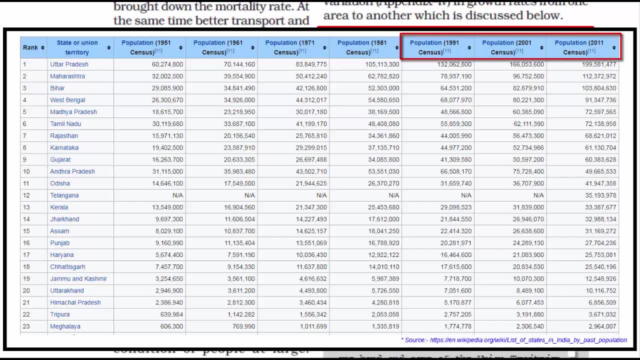 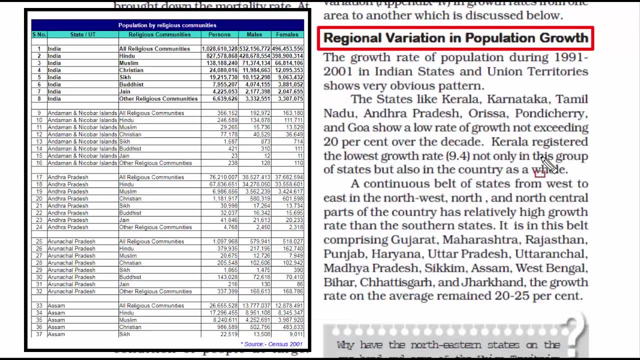 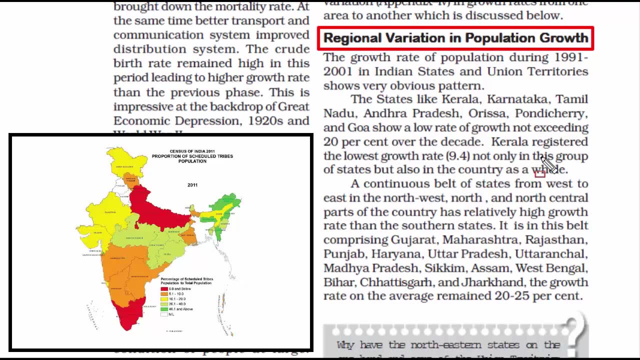 So let's start with the population growth, Because over the years we know the distribution pattern of our country's population, Like in a particular state, where the so and so communities live, which region is dominated by which community? Similarly, where do minorities reside? where do tribal communities live? 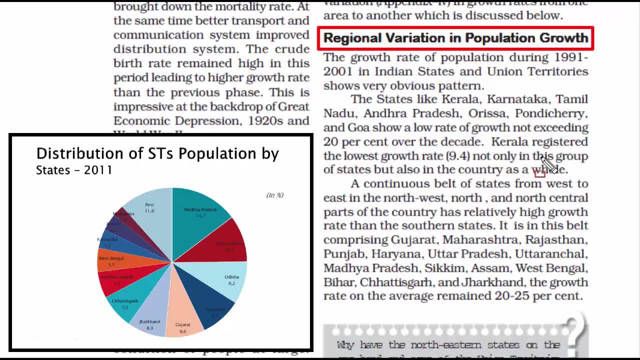 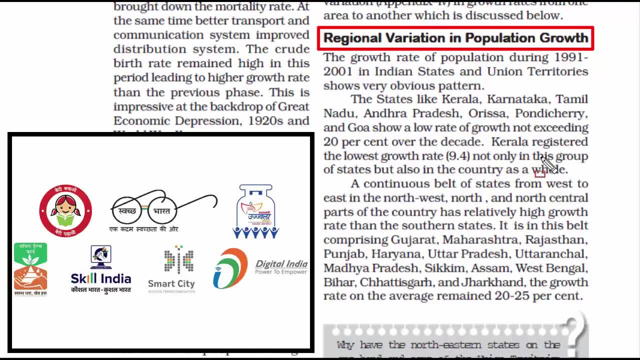 So all kinds of information is available with the government regarding our population And, if you think about it, this kind of information is necessary. Plus, it makes it easy for the government to implement schemes, welfare, etc. So let's start with the population growth. 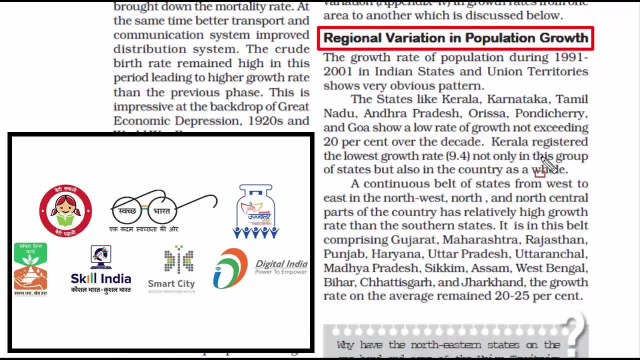 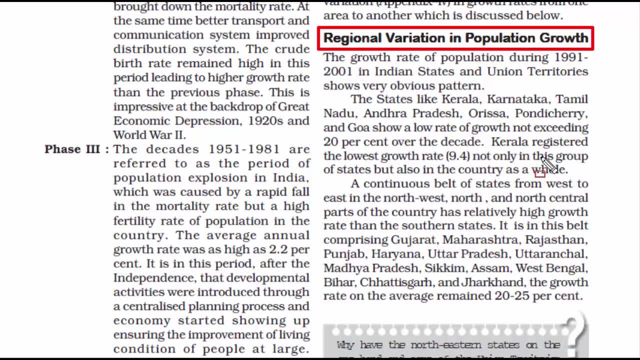 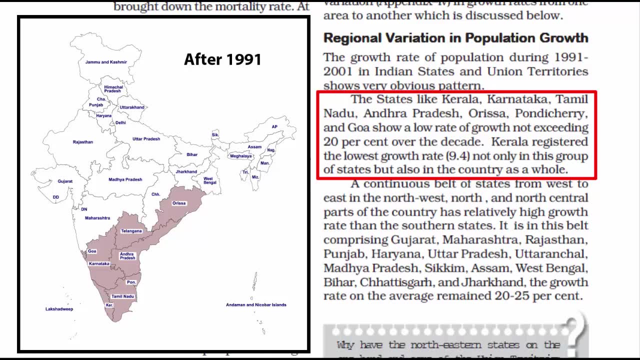 That's a different point whether or not people benefit from it, but you get the point right. That's the kind of information we get when we dig deep into the regional variation in population growth. Anyhow, after 1991, states like Kerala, Karnataka, Tamil Nadu, Andhra Pradesh, Odisha, Pondicherry, 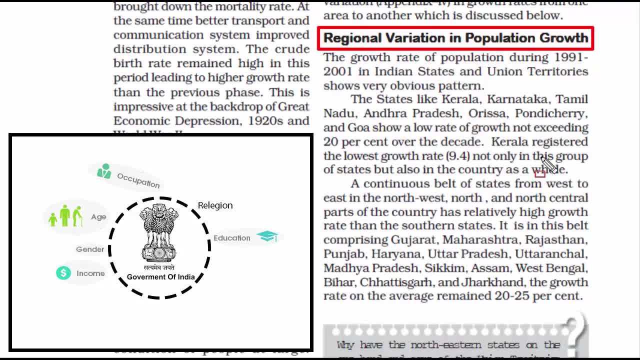 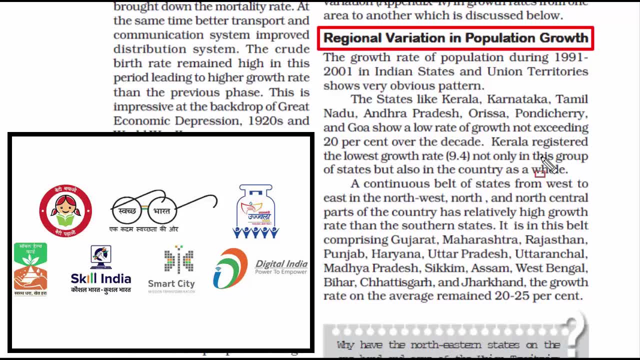 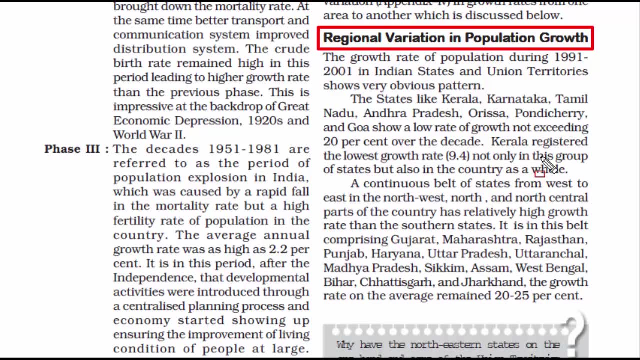 And, if you think about it, this kind of information is necessary. Plus, it makes it easy for the government to implement schemes, welfare etc for the people. That's a different point whether or not people benefit from it, But you get the point right. That's the kind of information we get when we dig deep into the regional variation in population growth. 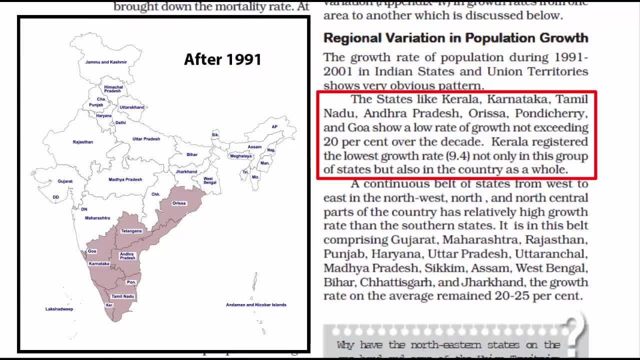 Anyhow, after 1991, states like Kerala, Karnataka, Tamil Nadu, Andhra Pradesh, Odisha, Pondicherry and Goa showed a low rate of growth, not exceeding 20%. over the decade, Kerala registered the lowest growth rate, 9.4%, not only in this group of states but also in the country as a whole. 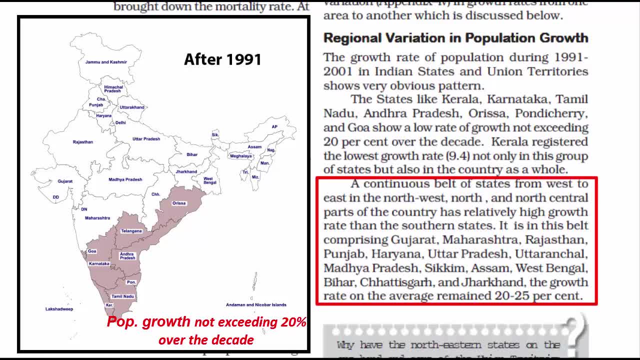 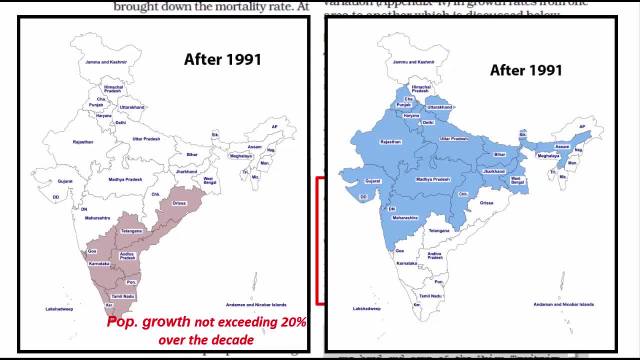 Notice. these are South Indian states. On the other hand, states like Gujarat, Maharashtra, Rajasthan, Punjab, Haryana, Uttar Pradesh, Uttaranchal, Madhya Pradesh, Sikkim, Assam, West Bengal, Bihar, Chhattisgarh and Jharkhand. the growth rate on the average remained 20-25%. 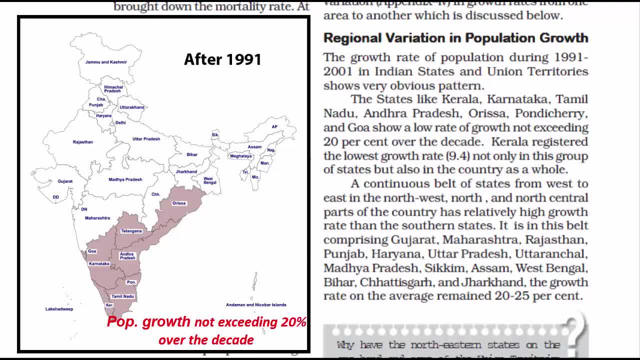 and Goa showed a low rate of growth, not exceeding 20% over the decade. Kerala registered the lowest growth rate, 9.4%, Not only in this group of states, but also in the country as a whole. Notice, these are South Indian states. 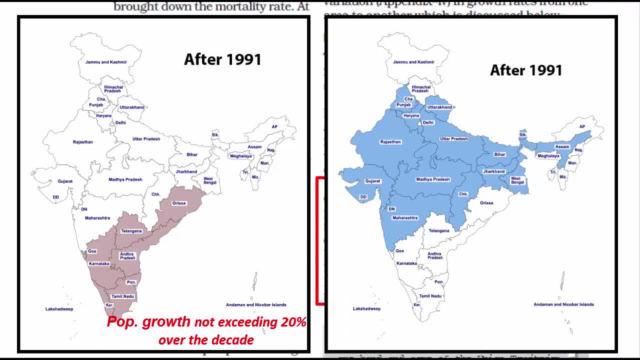 On the other hand, states like Gujarat, Maharashtra, Rajasthan, Punjab, Haryana, Uttar Pradesh, Uttaranchal, Madhya Pradesh, Sikkim, Assam, West Bengal, Bihar, Chhattisgarh and Jharkhand. 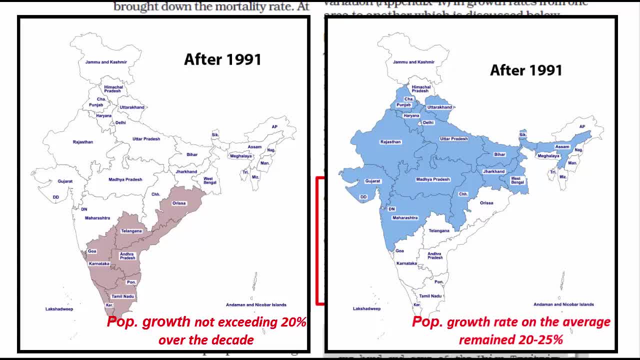 the growth rate on the average remained 20-25%, Meaning these western, central, northern and eastern parts of the country has relatively higher growth rate than the southern states. So clearly there is a difference between South India and North India when it comes to population. 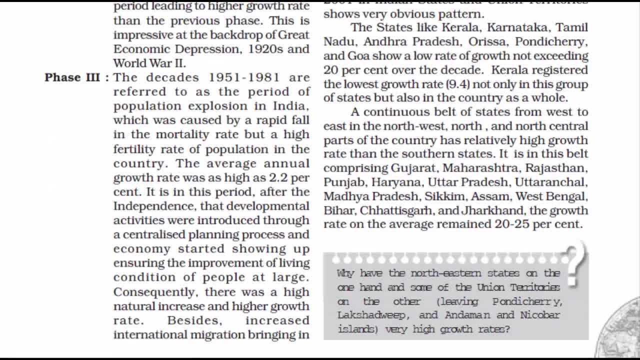 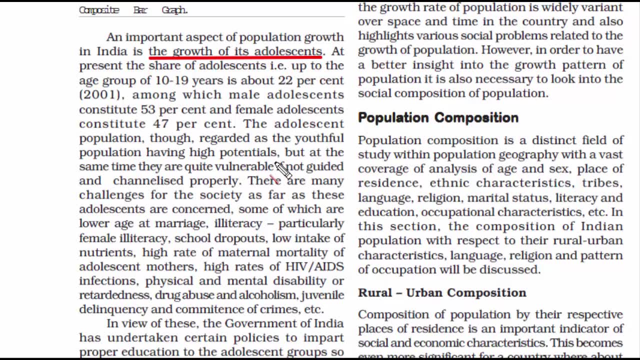 meaning few babies are being born in South. Another important aspect of population growth in India is the growth of its adolescence. When we say the word adolescent, we refer to the period where a young person develops from a child into an adult, And that age group is from 10 to 19 years. 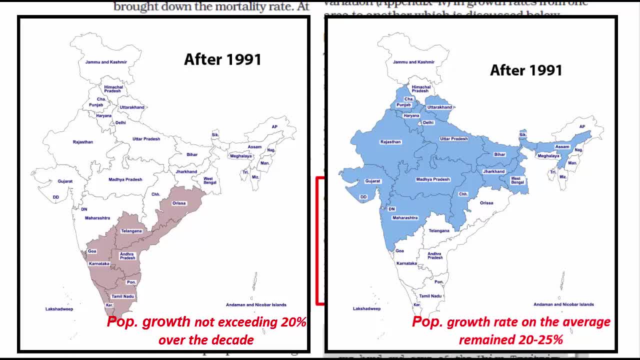 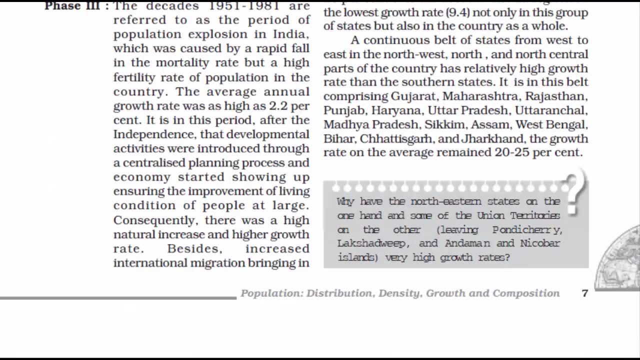 Meaning these western, central, northern and eastern parts of the country, has relatively higher growth rate than the southern states. So clearly there is a difference between South India and North India when it comes to population, meaning few babies are being born in South. Another important aspect of population growth in India is the growth of its population. 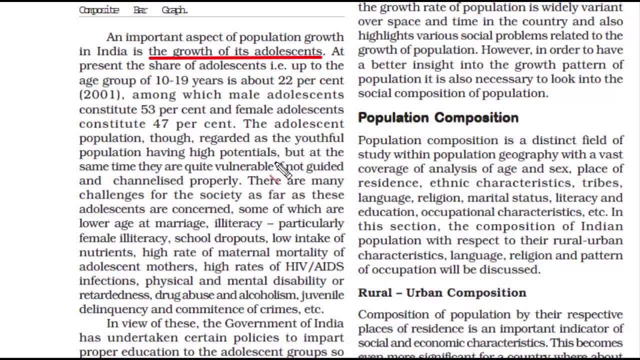 Adolescence. When we say the word Adolescent, we refer to the period where a young person develops from a child into an adult, And that age group is from 10 to 19 years. Here it says: as per the 2001 census, that count is around 22%. 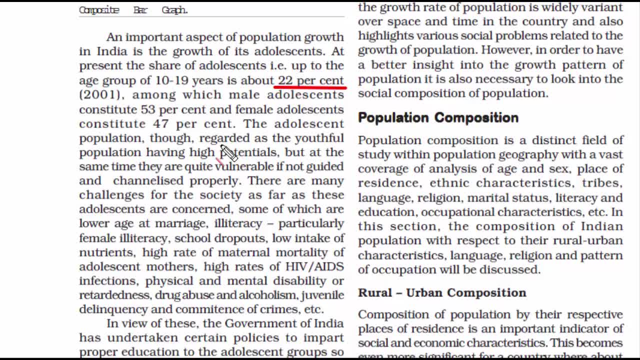 But currently, as per 2011 census, it is around 21.8%. In other words, every 5th person in India is an Adolescent, And you must have heard this many times that they are the bloodline of a nation, they are the change makers, they will define economic prosperity of a nation, etc. etc. 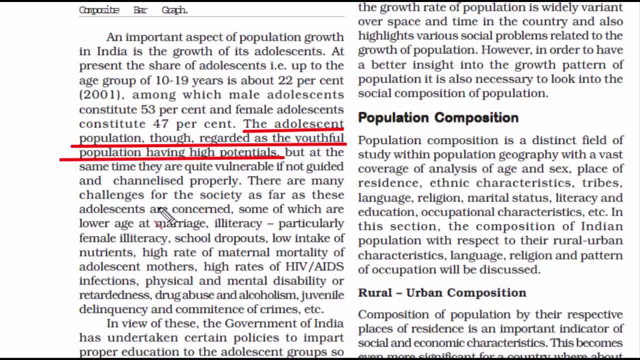 So there is a reason why these statements are being told about the youth, especially the age group of 10 to 19 years. I'll tell you about this in an informal sense so that you get an idea. So puberty can also be an exciting time, as children develop new emotions and feelings. 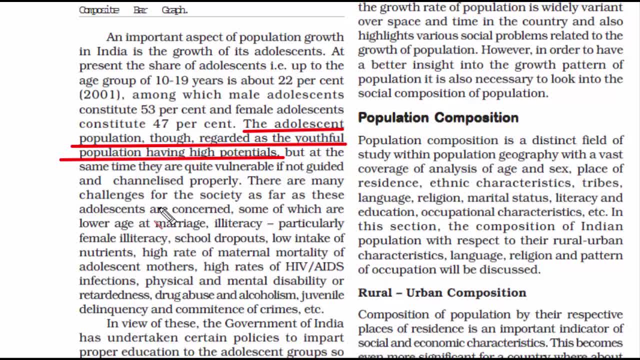 It can also have some psychological and emotional effects, such as unexplained mood swings, low self-esteem, etc. And puberty roughly occurs in between the ages of 10 to 16 years. This is also the time when students are in high school, You have your 10th and 12th board exams. 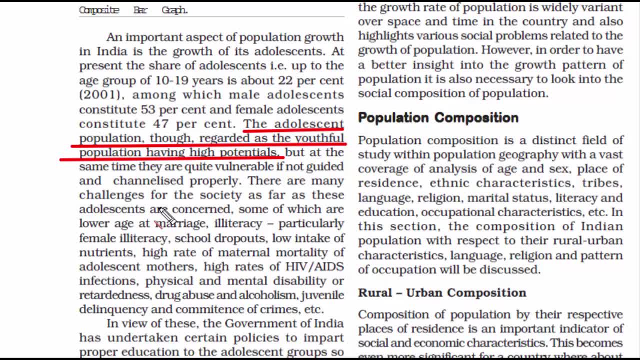 So all sorts of parental expectations and exam fear sets in. Apart from academics, students also have a social pressure, where they have this strong urge to discover their own drives, desires, passions and interests. Basically, they want to build their own identity or they are in self-exploration mode. 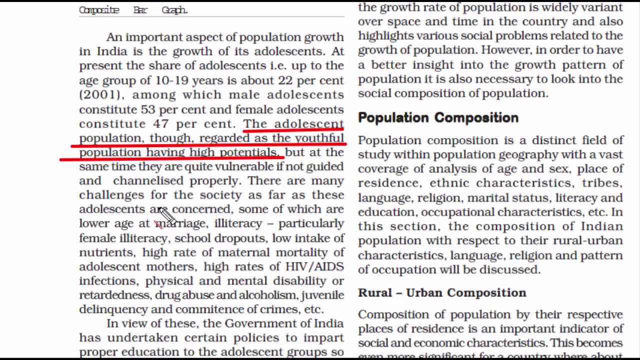 So they try out different roles and personalities and test them socially, emotionally and physically, And one of the ways students do this is by finding role models: You know, a person who they can look up to or someone they want to be like. For majority of the students, that role model is usually someone outside their family. 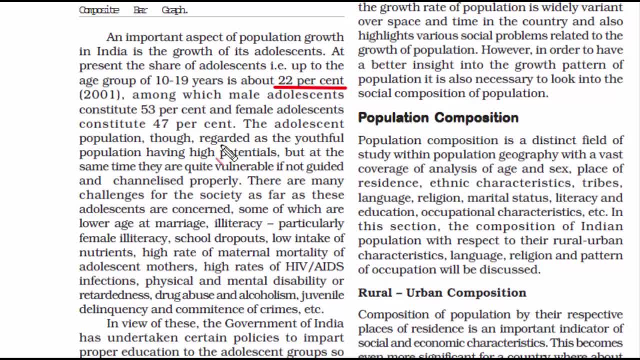 Here it says: As per the 2.5% growth rate in South India, the growth rate in South India is approximately 21.8%. compared to the 2001 census, that count is around 22%, But currently, as per 2011 census, it is around 21.8%. 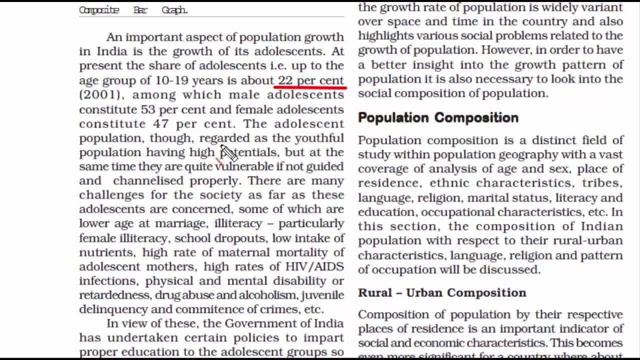 In other words, every 5th person in India is an adolescent, And you must have heard this many times that young people are the bloodline of a nation. they are the change makers, they will define economic prosperity of a nation, etc. etc. 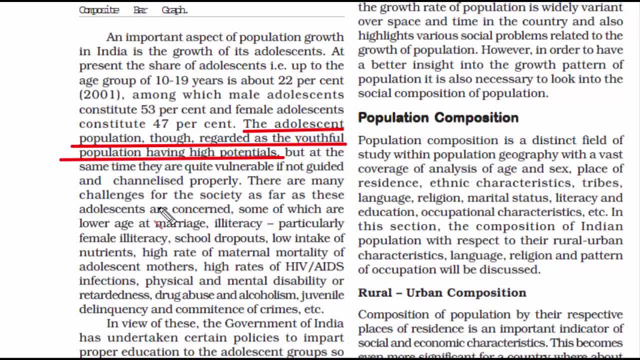 So there is a reason why these statements are being told about the youth, especially the age group of 10 to 19 years. I will tell you about this in an informal sense so that you get an idea. So puberty can also be an exciting time, as children develop new emotions and feelings. 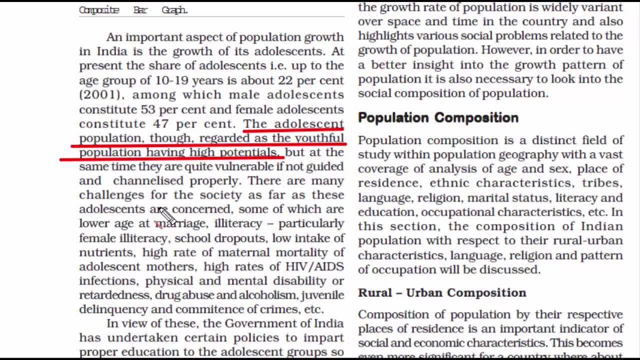 It can also have some psychological and emotional effects, such as unexplained mood swings, low self-esteem, etc. And puberty roughly occurs in between the ages of 10 to 16 years. This is also the time when students are in high school, You have your 10th and 12th board exams. 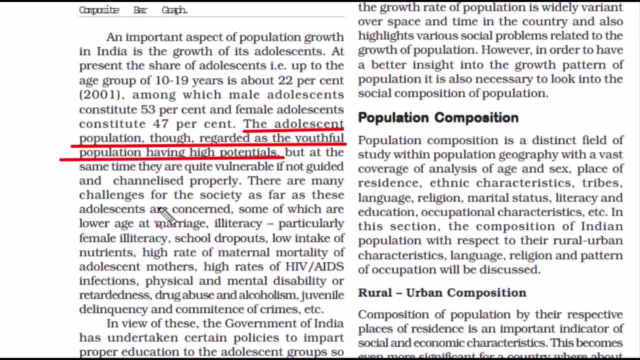 So all sorts of parental expectations And exam fear sets in. Apart from academics, students also have a social pressure, where they have this strong urge to discover their own drives, desires, passions and interests. Basically, they want to build their own identity. 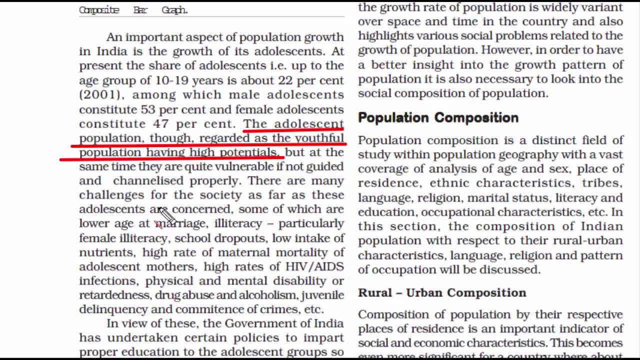 Or they are in self-exploration mode. So they try out different roles and personalities and test them socially, emotionally and physically. And one of the ways students do this is by finding role models: You know, a person who they can look up to or someone they want to be like. 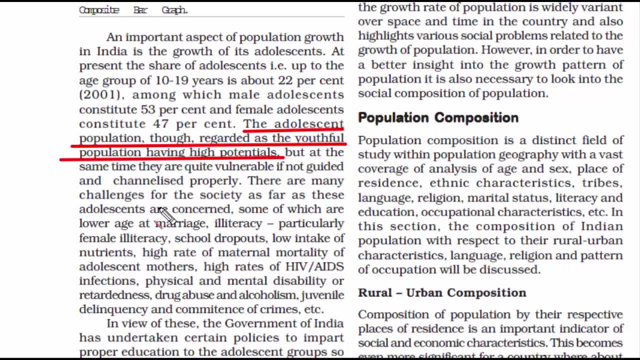 For majority of the students, That role model is usually someone outside their family. Today, with the presence of social media, we now have a global landscape to draw influence or inspiration from People who drink, smoke or do drugs. 8 out of 10 will admit they have discovered all. 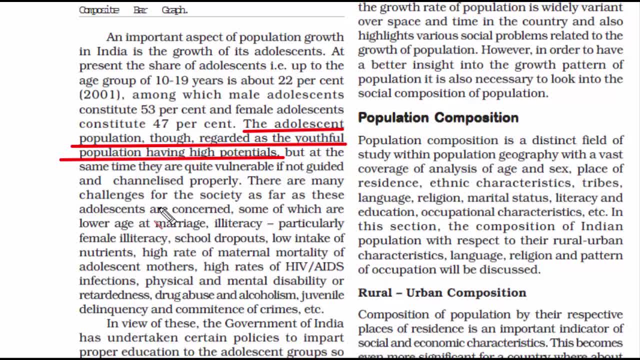 of this during high school. The number of Indian teenagers consuming alcohol is increasing, especially in metro cities, where it has been accepted as a way of socializing, not only among adults, but also among teenagers. That's why this period of time is so important. 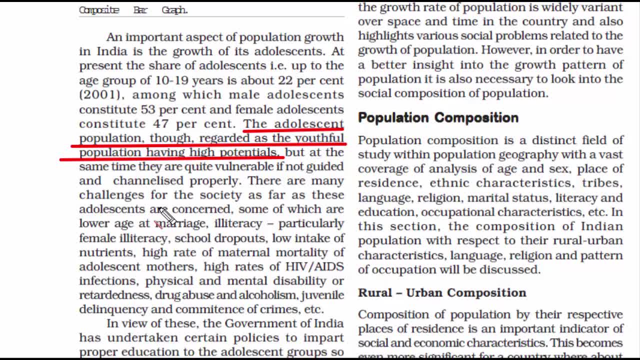 Today, with the presence of social media, we now have a global landscape to draw influence or inspiration from People who drink, smoke or do drugs. 8 out of 10 will admit they have discovered all of this during high school. The number of Indian teenagers consuming alcohol is increasing, especially in metro cities. 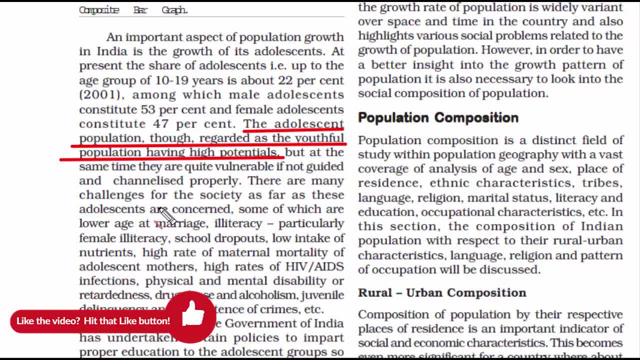 where it has been accepted as a way of socializing, not only among adults, but also among teenagers. That's why this period of adolescence is a vulnerable period of one's life. Here it's written. if not guided and channelized properly, there are many challenges for the society as far as these adolescents are concerned. 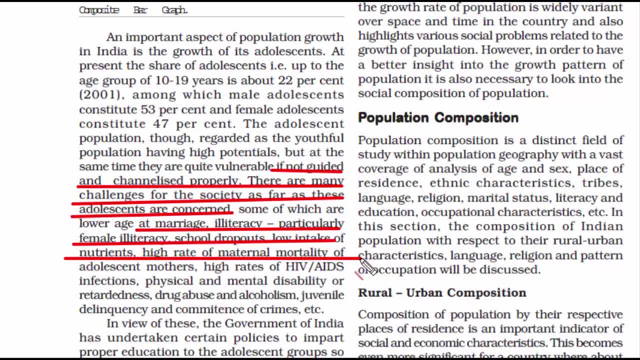 some of which are: lower age of marriage, high literacy, particularly female illiteracy, school dropouts, low intake of nutrients, high rate of maternal mortality of adolescent mothers, high rates of HIV, AIDS infections, physical and mental disability, drug abuse and alcoholism. 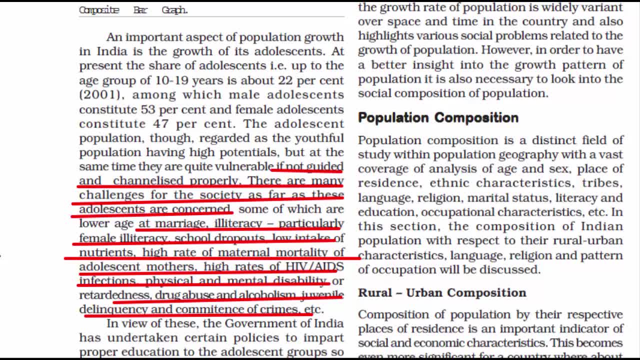 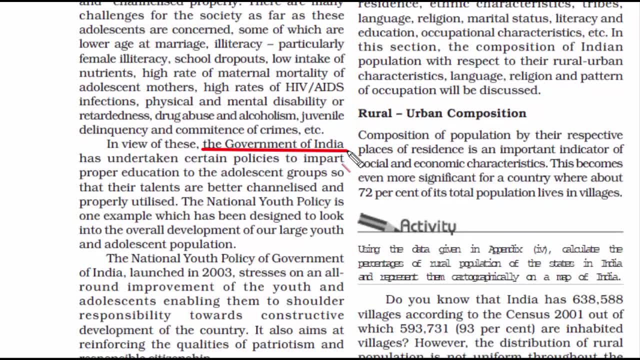 juvenile delinquency and committance of crimes, etc. Yeah, so these are the problems that exist not in India, but everywhere in the world. So naturally, it is the respective government's duty to look into it and do something about it. After all, these young people are going to join the workforce. 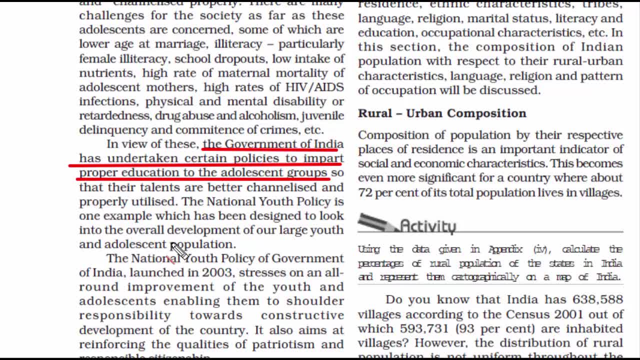 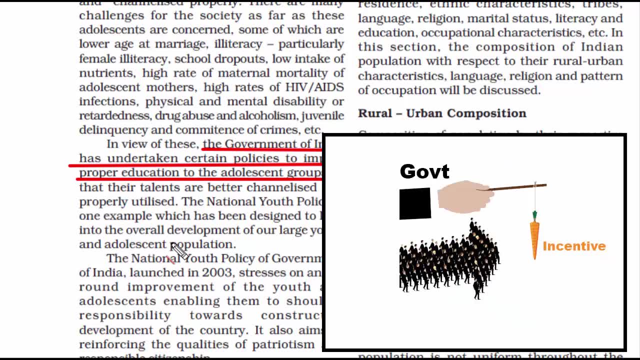 So, be it in economic sense or moral sense, the government has to do something about it. And one more thing you have to understand is that government can do two things: Either it will give incentive to encourage certain behavior, or it will create a law to discourage certain behaviors. 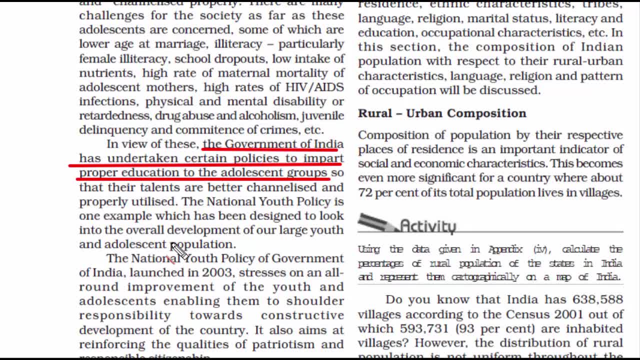 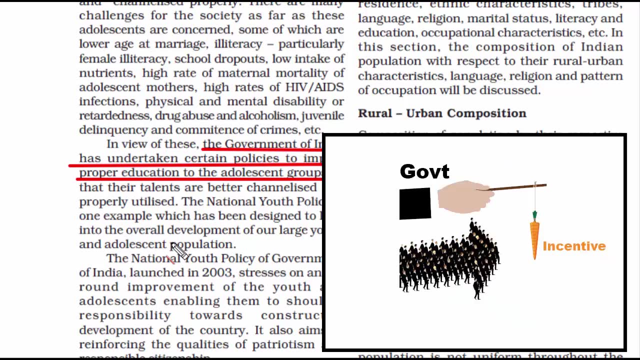 These are two effective ways government controls its citizens. Keeping that in mind, the government of India has undertaken certain policies to impart proper education to the adolescent groups so that their talents are better channelized and properly utilized. You see, the government is talking about incentives to encourage certain behavior. 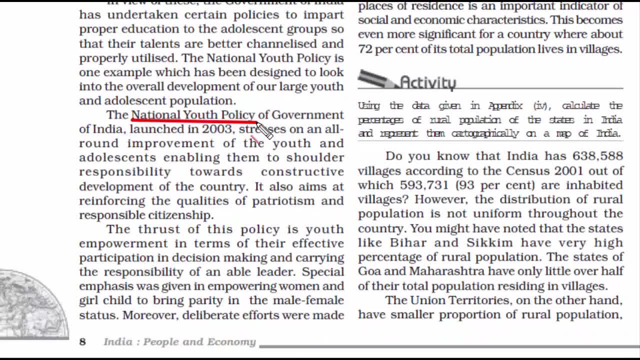 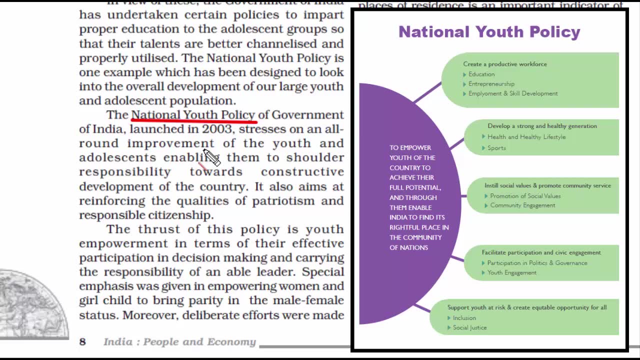 The National Youth Policy is one example, which has been designed to look into the overall development of our large youth and adolescent population. It was formulated in 2003.. The idea of this program is to identify five well-defined objectives and eleven priority areas. that empowers youth to achieve their full potential. 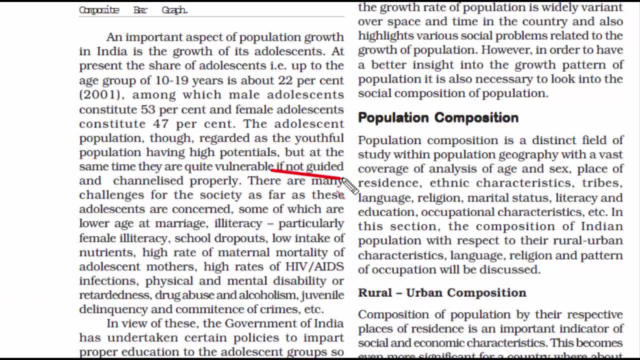 As we all know, for many of us, the age of adolescence is a vulnerable period of one's life. Here it's written. if not guided and channelized properly, there are many challenges for the society as far as these adolescents are concerned, some of which are lower age of marriage, illiteracy. 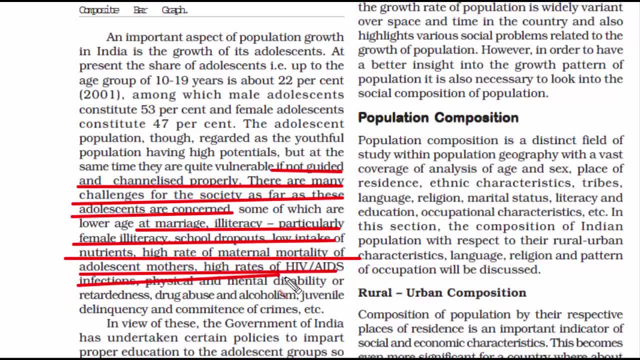 particularly female: illiteracy, school dropouts, low intake of nutrients, high rate of maternal mortality of adolescent mothers, high rates of HIV AIDS infections, physical and mental disability, drug abuse and alcoholism, juvenile delinquency, delinquency and committance of crimes, etc. 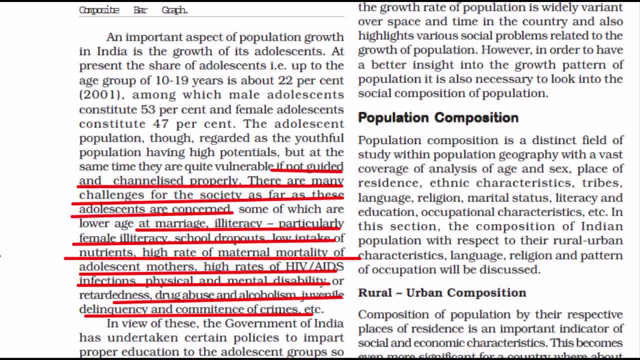 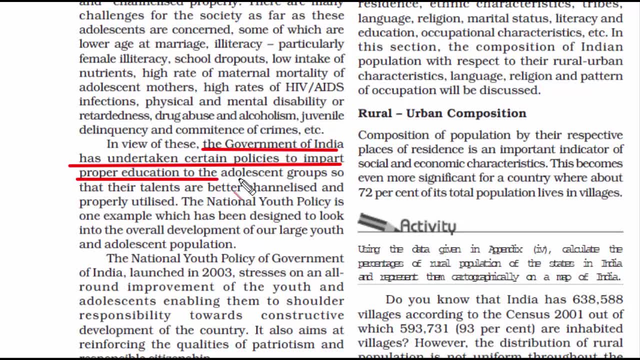 Yeah, so these are the problems that exist not in India, but everywhere in the world, So naturally, it is the respective government's duty to look into it and do something about it. After all, these young people are going to join the workforce. 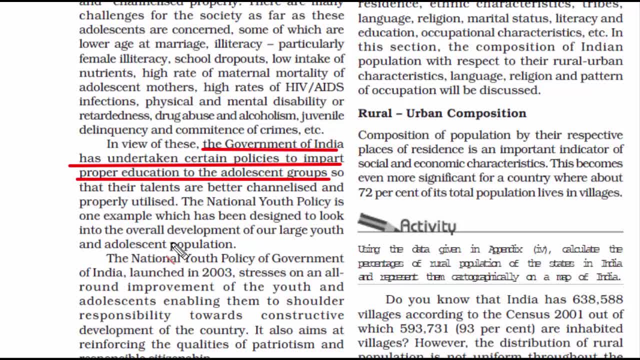 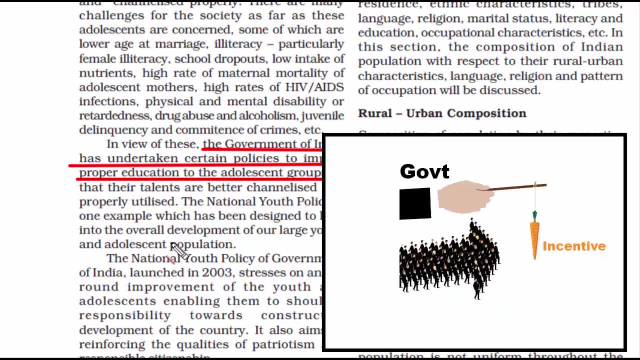 So, be it in economic sense or moral sense, the government has to do something about it. And one more thing you have to understand is that government can do two things: Either it will give incentive to encourage certain behavior, or it will create a law to discourage certain behaviors. 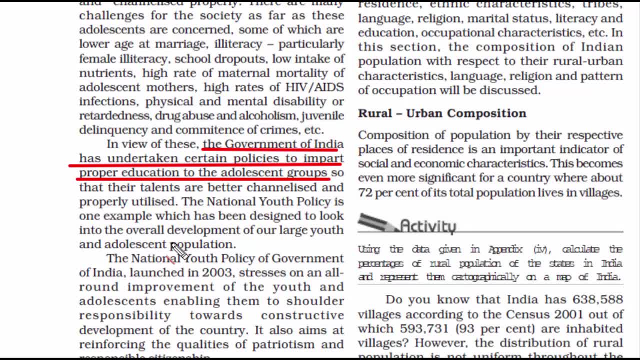 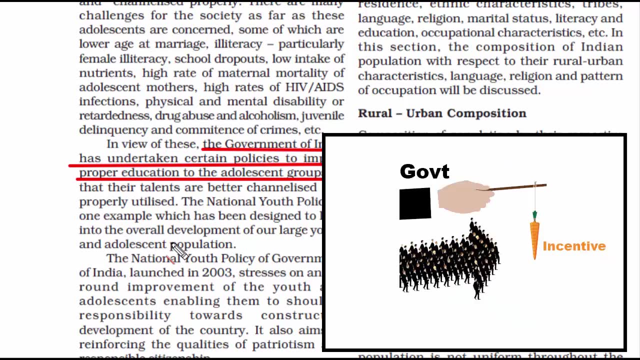 These are two effective ways government controls its citizens. Keeping that in mind, the government of India has undertaken certain policies to impart proper education to the adolescent groups so that their talents are better channelized and properly utilized. You see, the government is talking about incentives to encourage certain behavior. 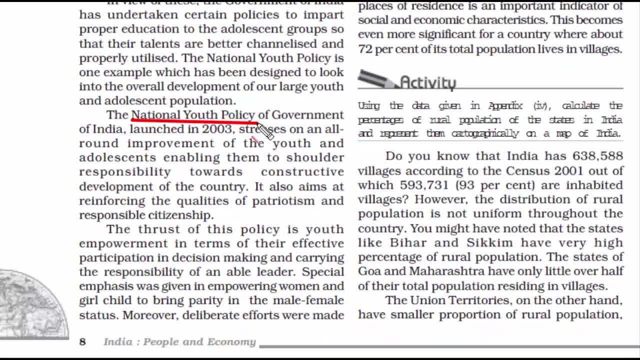 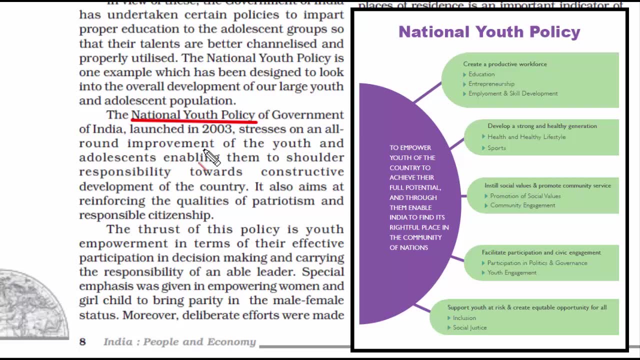 The National Youth Policy is one example, Which has been designed to look into the overall development of our large youth and adolescent population. It was formulated in 2003.. The idea of this program is to identify five well-defined objectives and 11 priority areas. 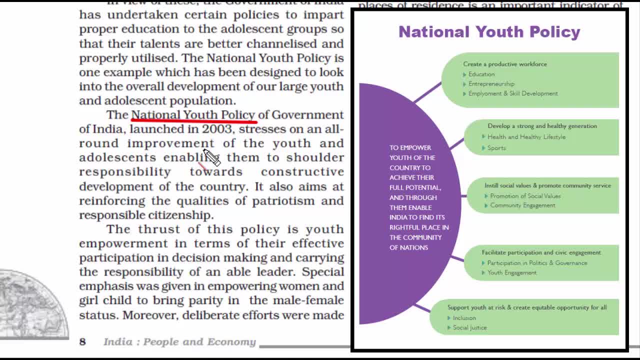 that empowers youth to achieve their full potential and which, in turn, will contribute to the progress of the nation. The priority areas are education, skill development and employment, entrepreneurship, health and healthy lifestyle, Sports, promotion of social values, community engagement, participation in politics and governance, youth engagement, inclusion and social justice. 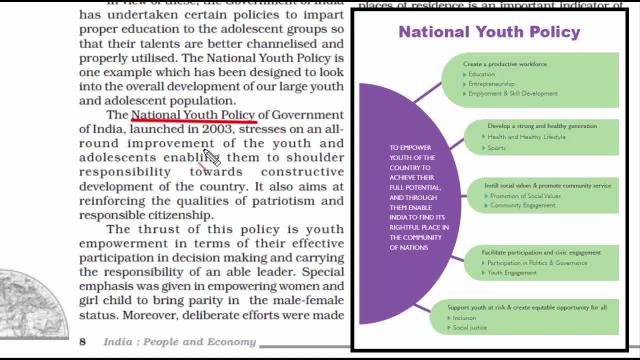 and which, in turn, will contribute to the progress of the nation. The priority areas are education, skill development and employment, entrepreneurship, health and healthy lifestyle, sports, promotion of social values, community engagement, participation in politics and governance, youth engagement, inclusion and social justice. 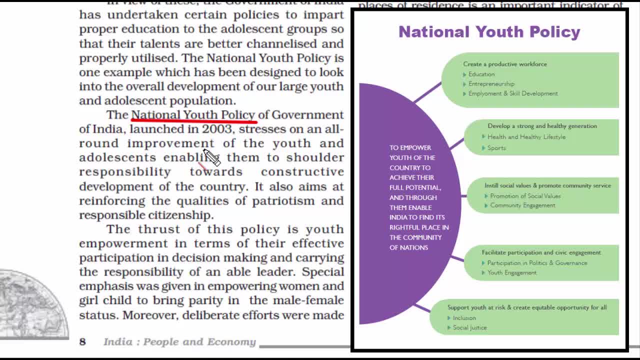 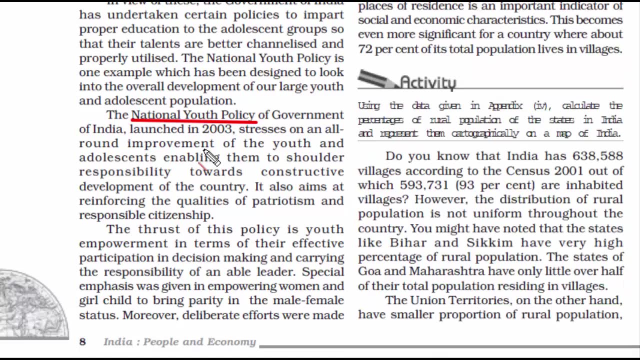 Again, the whole idea behind National Youth Policy is to have a framework where the government and non-government stakeholders can tap into the young human resources by enabling them to realize their full potential. that will further contribute to the progress of the nation. If you notice how we are slowly going, step by step, into the fine details of Indian population, 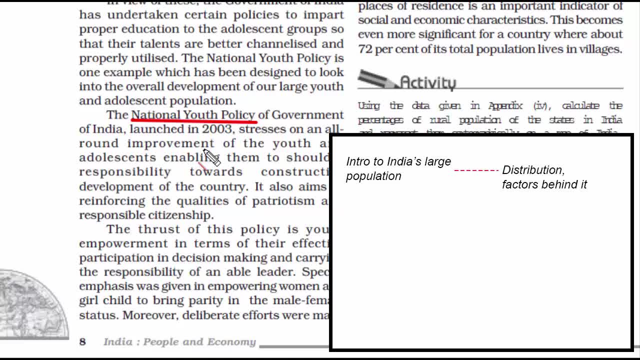 At first we learned about India's large population. After that its distribution and what are the factors behind it. Then we learned about the density of the population. After that we learned how population of India grew with time. We saw four phases of population growth. 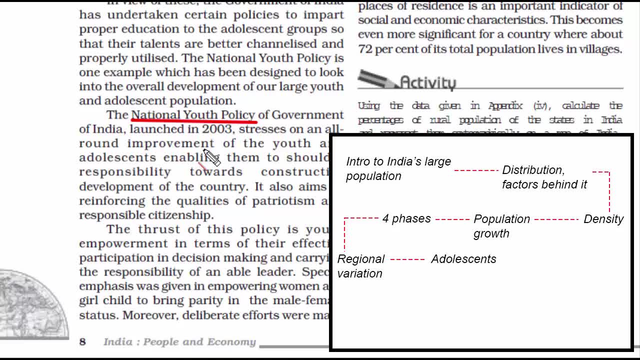 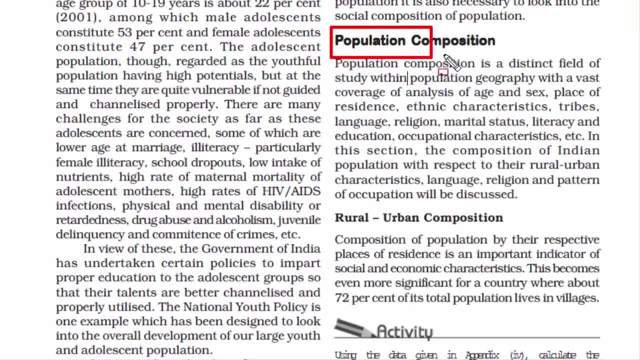 Then we saw population growth patterns within states and regions. After that we learned about the adolescence population, which is also the youth of the country, And now we will look into the social composition of population When we look at the words population composition. 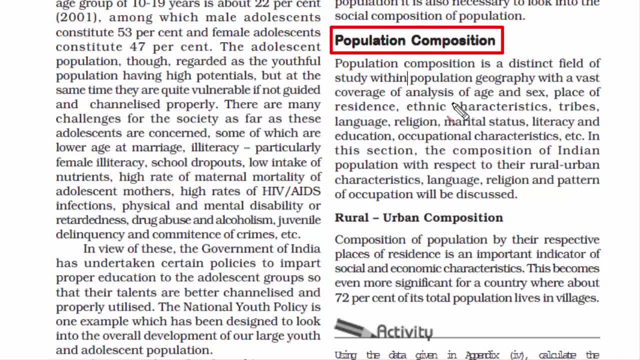 it means: what is the population composed of? What are the ingredients that makes up the population? Just like how a dish is prepared and it has different variety of ingredients, similarly a population also has some ingredients, or you can say different characteristics such as age and sex. 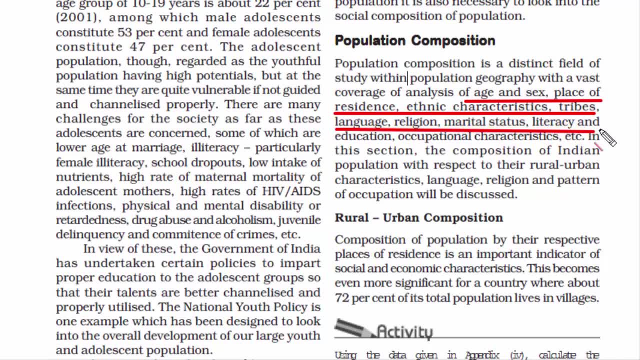 place of residence, ethnic characteristics, tribes, language, religion, marital status, literacy and education, occupational characteristics, etc. But in this chapter we will read about the composition of Indian population with respect to their rural to urban characteristics, language, religion and pattern of occupation. 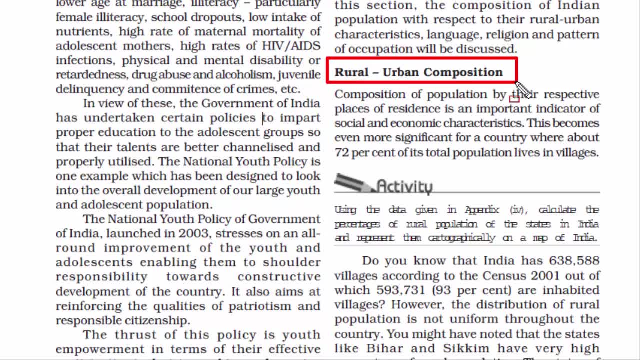 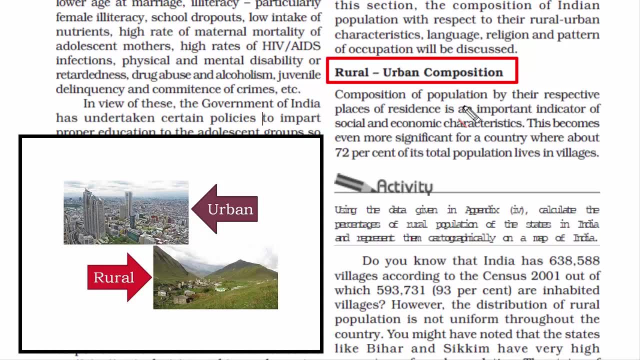 Let's look at the rural to urban composition. Any population is divided into two parts: rural and urban. In other words, you have to be aware where does the population reside. I mean, how much of it is in the urban area and how much of it is in the rural area. 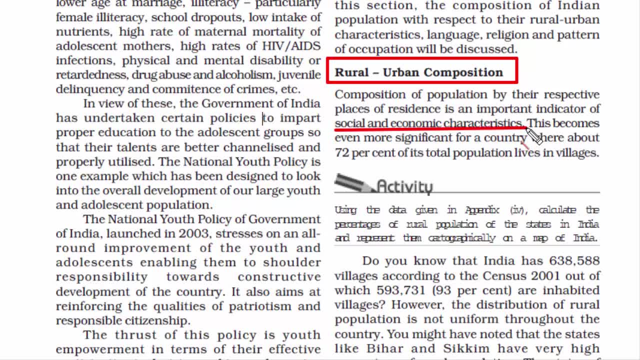 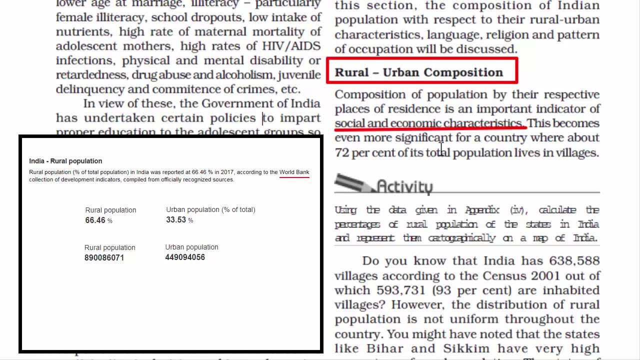 Because that will tell you a lot about a country's population in terms of social and economic characteristics. We know that urban areas are more developed. It has more facilities, infrastructure, opportunity, etc. According to the World Bank, in India, the rural population was reported at 66.46% in 2017.. 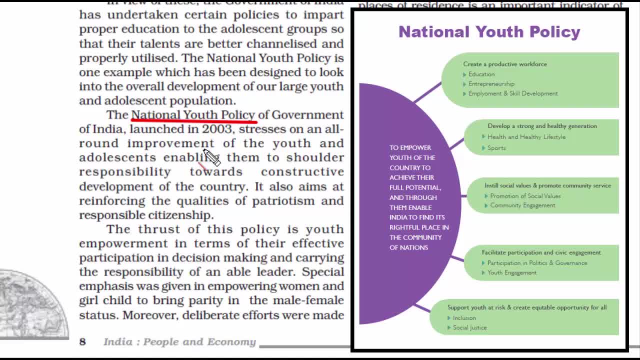 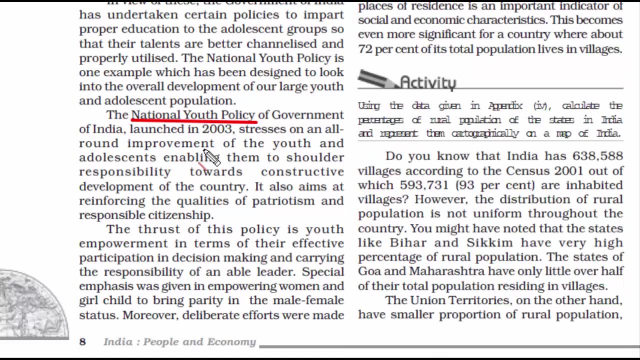 Again, the whole idea behind National Youth Policy is to have a framework where the government and non-government stakeholders can tap into the young human resources by enabling them to realize their full potential. that will further contribute to the progress of the nation. If you notice how we are slowly going, step by step, into the fine details of Indian population, 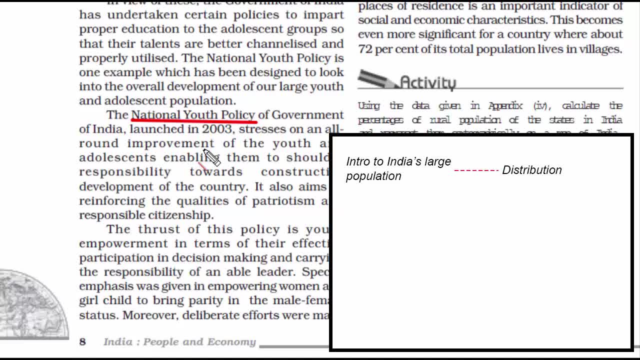 At first we learned about India's large population, after that its distribution and what are the factors behind it. Then we learned about the density of the population. After that we learned how population of India grew with time. We saw four phases of population growth. 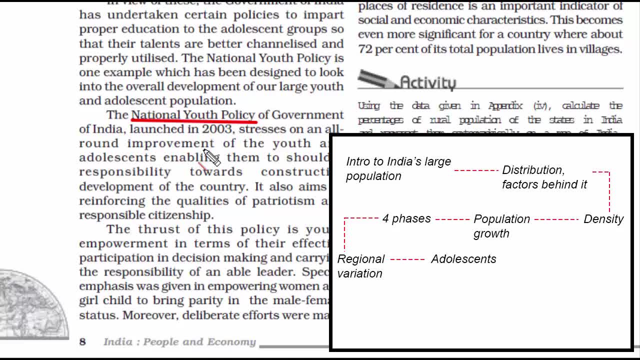 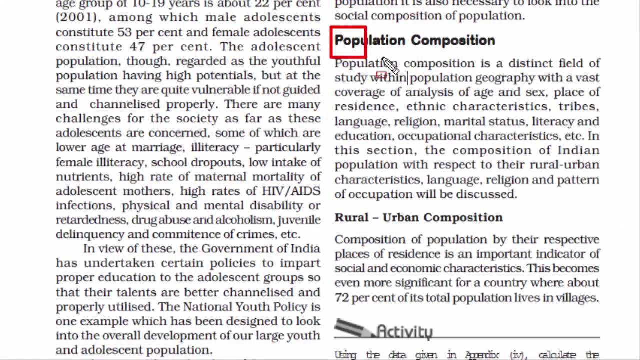 Then we saw population growth patterns within states and regions. After that we learned about the adolescence population, which is also the youth of the country. And now we will look into the social composition of population, The social composition of population. When we look at the words population composition, it means: what is the population composed of? 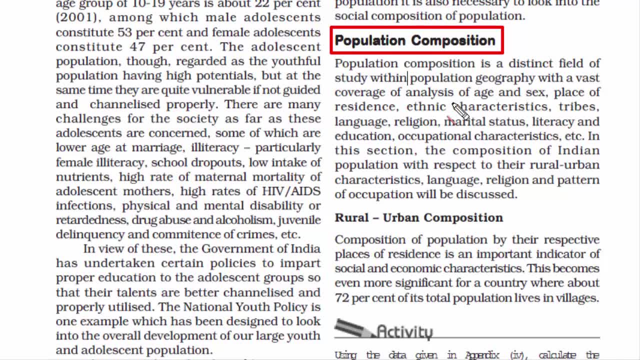 What are the ingredients that makes up the population? Just like how a dish is prepared and it has different variety of ingredients, Similarly a population also has some ingredients, or you can say different characteristics, such as age and sex, place of residence, ethnic characteristics, tribes, language, religion, marital status, literacy and education, occupational characteristics, etc. 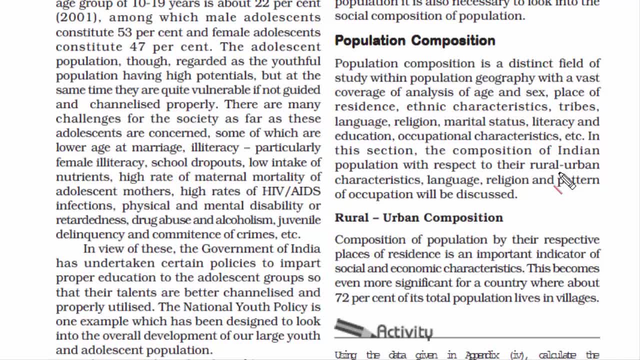 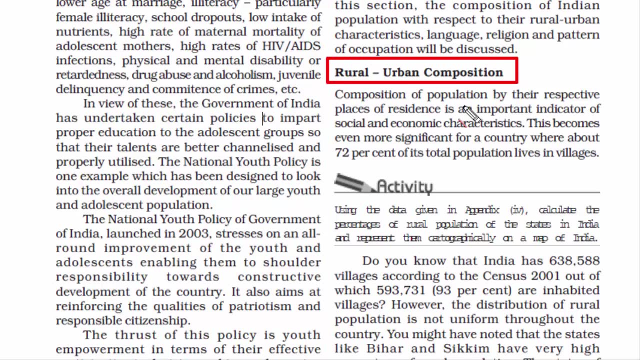 But in this chapter we will read about the composition of Indian population with respect to their rural to urban characteristics, language, religion and pattern of occupation. Let's look at the rural to urban composition. Any population is divided into two parts: rural and urban. 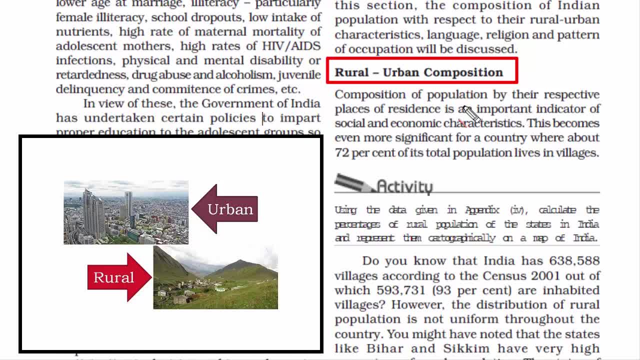 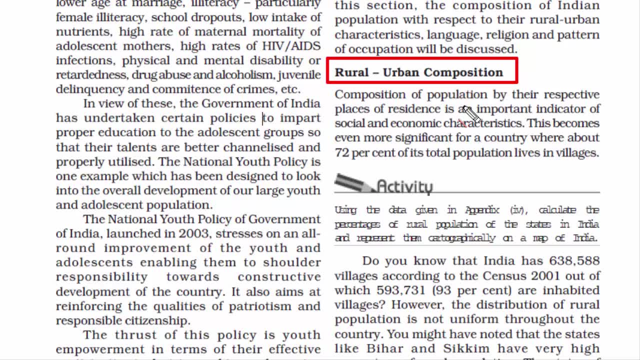 In other words, you have to be aware where does the population reside, I mean how much of it is in the urban area and how much of it is in the rural area, Because that will tell you a lot about a country's population in terms of social and economic characteristics. 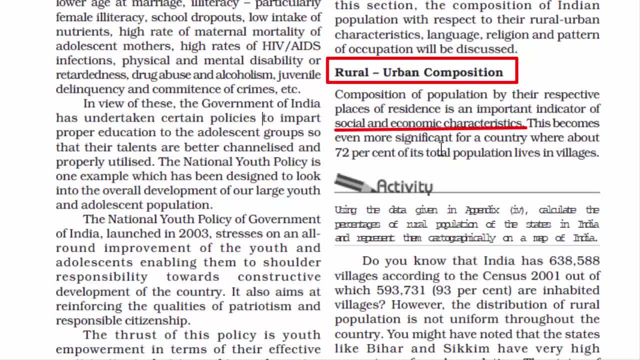 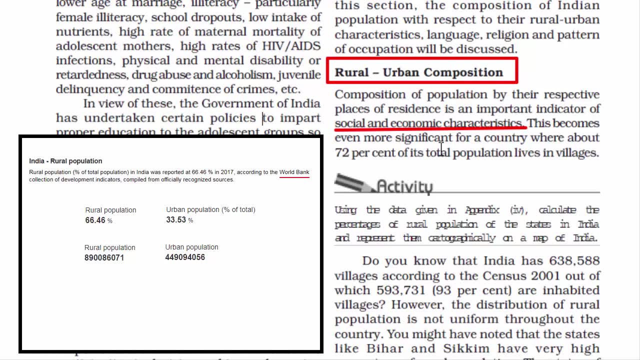 We know that urban areas are more developed. It has more facilities, infrastructure, opportunity, etc. According to the World Bank, in India, the rural population was reported at 66.46% in 2017.. And the urban population is at 33.53%. 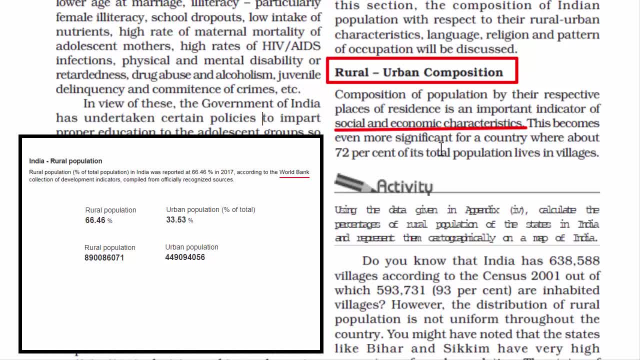 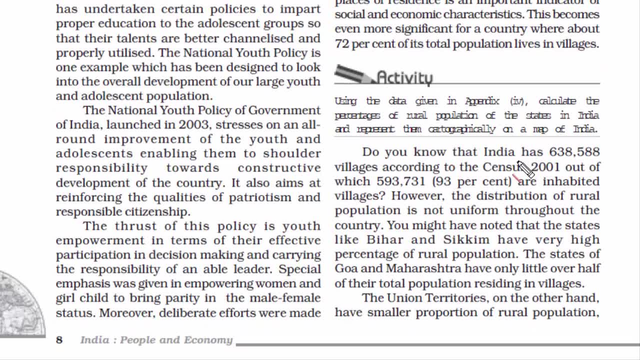 And the urban population is at 33.53%. The data that you see in this chapter is from 2001 census. Anyhow, I am giving you the latest figures In this book. the data is slightly old Again. as per the 2001 census, India has around 6,38,588 villages. 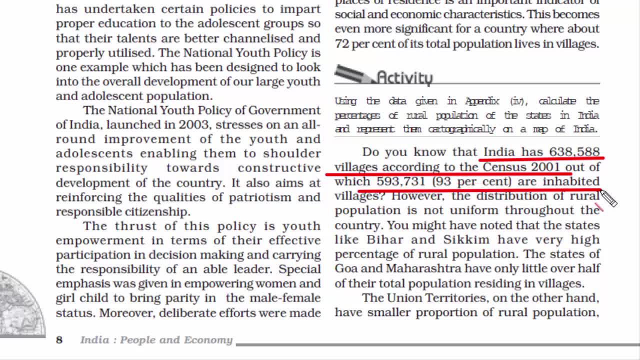 out of which 5,93,731 inhabited villages, meaning here people live. As per 2011 census, India has around 6,50,244 villages. Now, the distribution of all these villages are uneven throughout the country, Meaning there are some states and union territories where villages and rural population 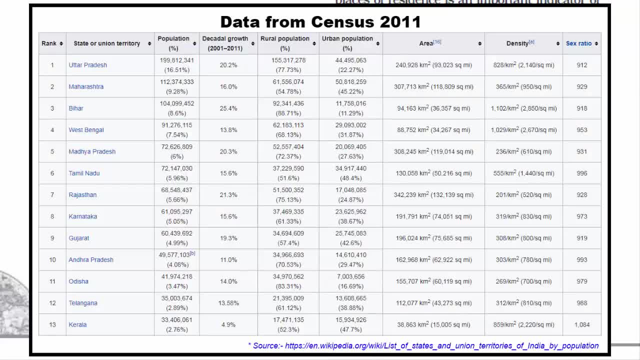 are more compared to the other states. What you can do is look for state-wise rural and urban population data And see which state has more rural population. Census of India provides this kind of information on every 10 years gap. Compare it and see whether the rural population has remained same or decreased. 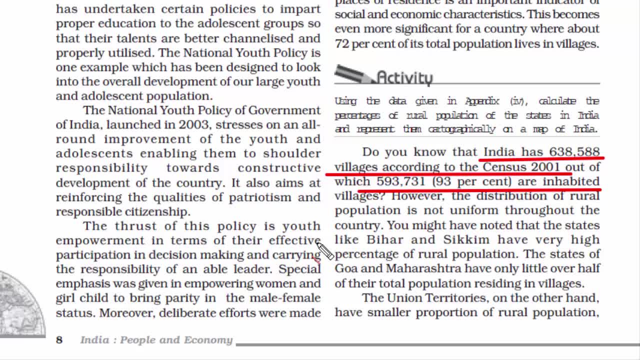 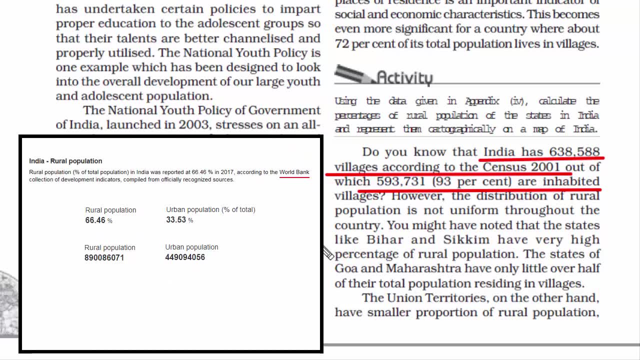 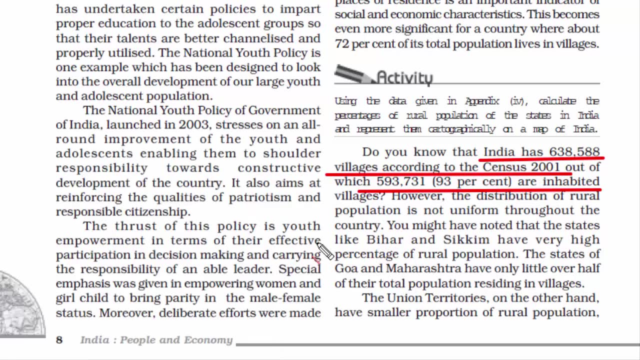 You will also find out whether, to what extent, rural to urban migration has taken place Anyhow. at present, the rural population of India is much higher than the urban population. However, the urban population is showing a much faster rate of growth, mainly due to enhanced economic development and improvement in health and hygienic conditions. 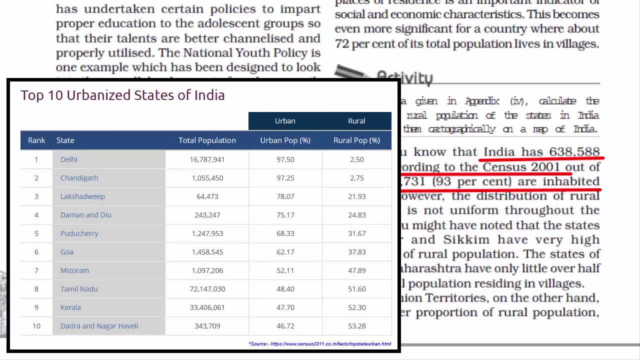 Here is the list of top 10 urbanized states and union territories of India, as per the 2011 census. Among all the states and union territories, the National Capital Territory of Delhi and the Union Territory of Chandigarh are most urbanized, with 97.5% and 97.25% urban population respectively. 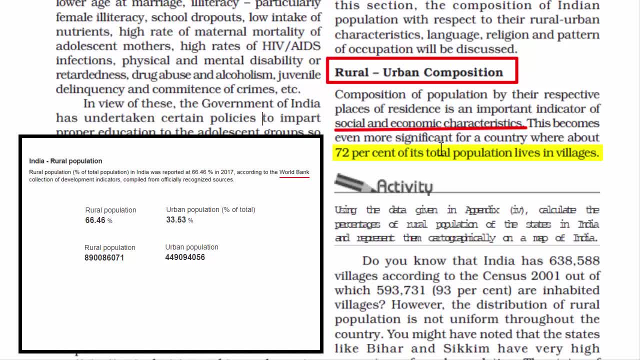 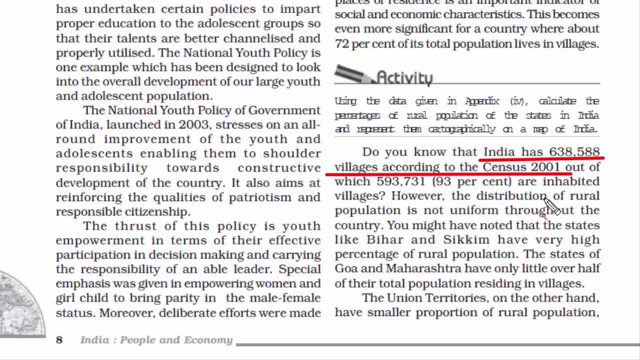 The data that you see in this chapter is from 2001 census. Anyhow, I am giving you the latest figures In this book. the data is slightly old. Again, as per the 2001 census, India has around 6,38,588 villages, out of which 5,93,731 inhabited villages, meaning here people live. 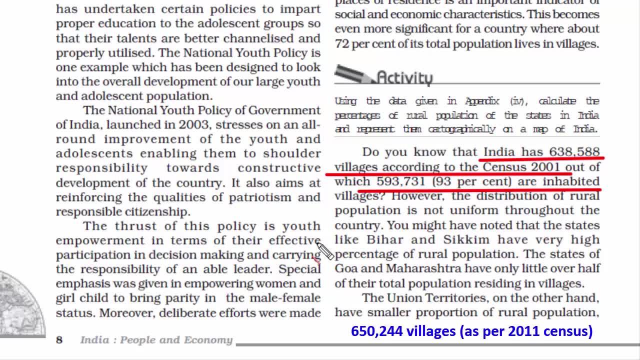 As per 2011 census, India has around 6,50,244 villages. Now, the distribution of all these villages are uneven throughout the year, Meaning there are some states and union territories where villages and rural population are more compared to the other states. 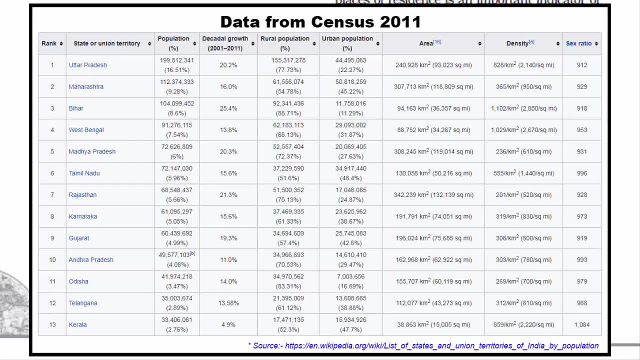 What you can do is look for state-wise rural and urban population data And see which state has more rural population. Census of India provides this kind of information on every 10 years gap. Compare it and see whether the rural population has remained same or decreased. 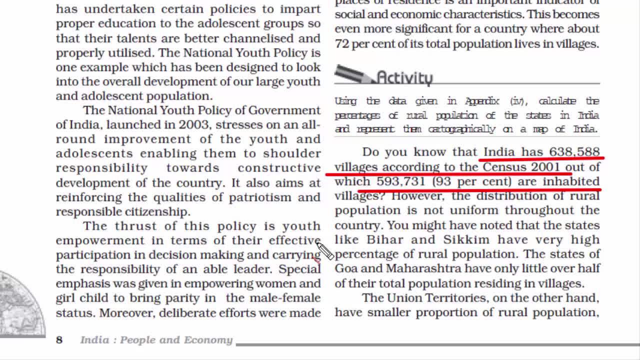 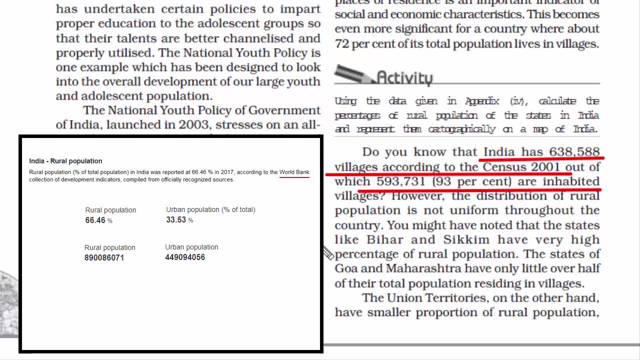 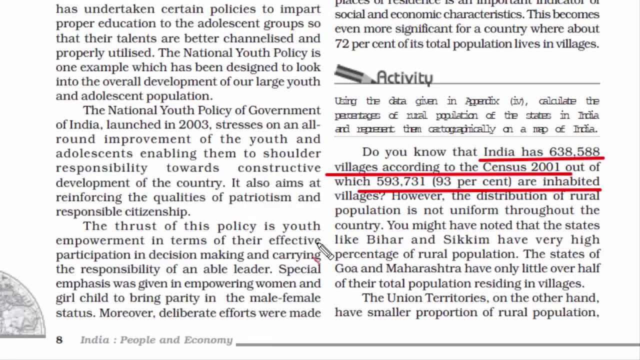 You will also find out whether, to what extent, rural to urban migration has decreased Anyhow. at present, the rural population of India is much higher than the urban population. However, the urban population is showing a much faster rate of growth, Mainly due to enhanced economic development and improvement in health and hygienic conditions. 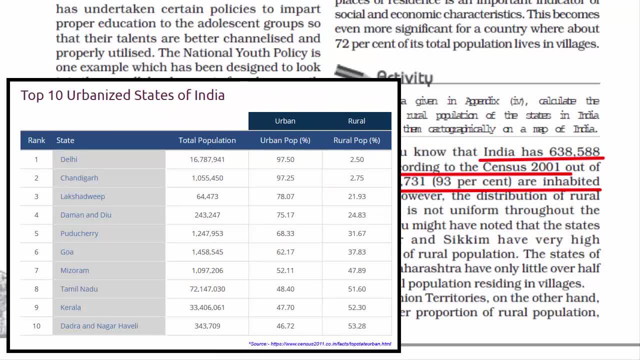 Here is the list of top 10 urbanized states and union territories of India, as per the 2011 census. Among all the states and union territories, the National Capital Territory of Delhi and the Central Capital Territory of India and the Union Territory of Chandigarh. 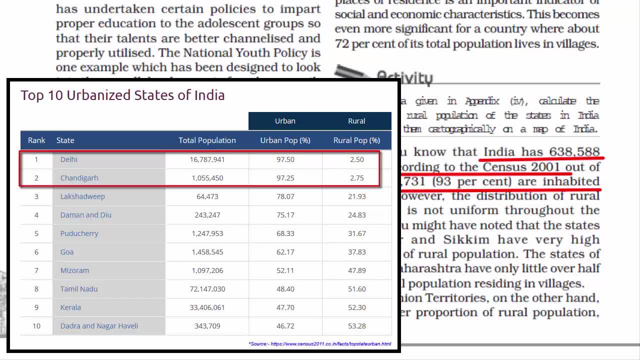 are most urbanized, with 97.5% and 97.25% urban population respectively, Followed by Damanandu, which is at 75.2%, and Puducherry, which is at 68.3%. Among states, Goa is now the most urbanized state, with 62.2% urban population. 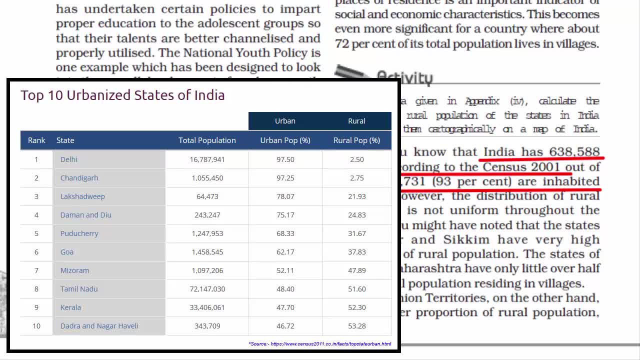 Followed by Damanandu, which is at 75.2%, and Puducherry, which is at 68.3%. Among states, Goa is now the most urbanized state, with 62.2% urban population, A significant increase since 2001, when urban population of Goa was 49.8%. 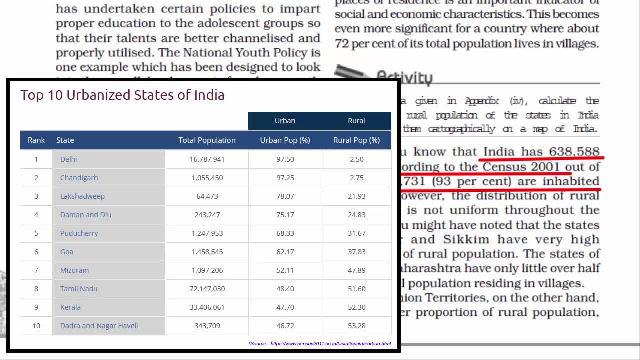 Another significant instance of rapid urbanization is that of Kerala. Its urban population is now at 47.7%, while a decade ago it was just 25.9%. Among the northeastern states, Mizoram is most urbanized, with 51.5% urban population. 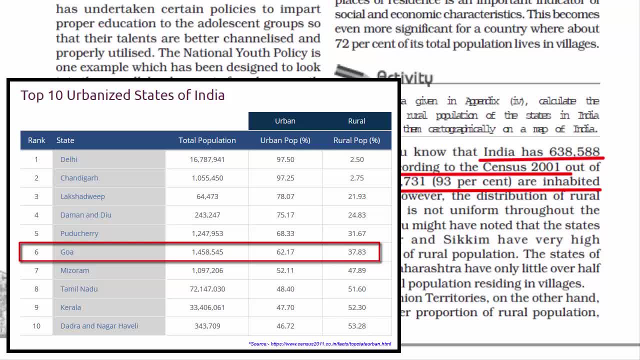 A significant increase since 2001,, when urban population of Goa was 49.2%. Another significant instance of rapid urbanization is that of Kerala. Its urban population is now at 47.7%, while a decade ago it was just 25.9%. 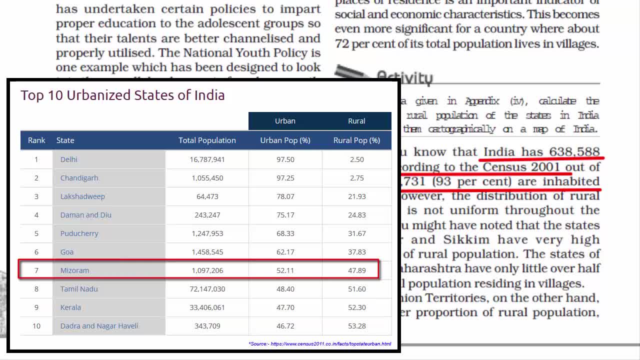 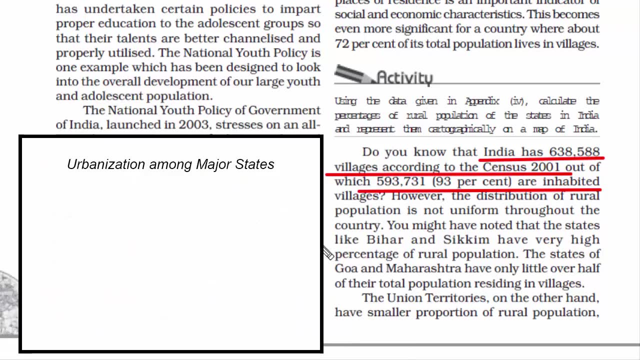 Among the northeastern states, Mizoram is most urbanized, with 51.5% urban population, Though in terms of absolute contribution to total urban population in the country, Mizoram's contribution is just 0.1%. Among major states, Tamil Nadu continues to be the most urbanized state, with 48.4%. 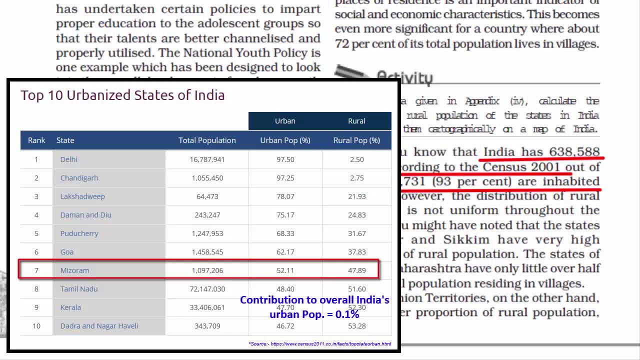 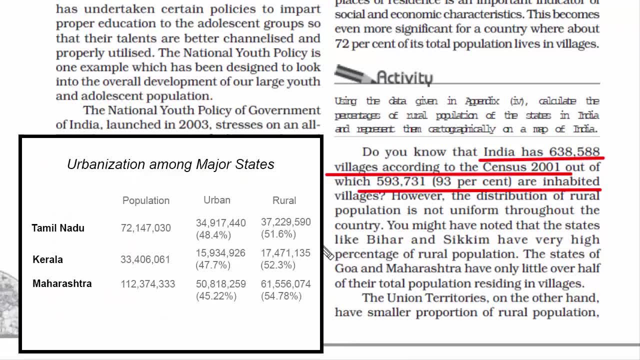 Though, in terms of absolute contribution to total urban population in the country, Mizoram's contribution is just 0.1%. Among major states, Tamil Nadu continues to be the most urbanized state, with 48.4% of the population living in urban areas. 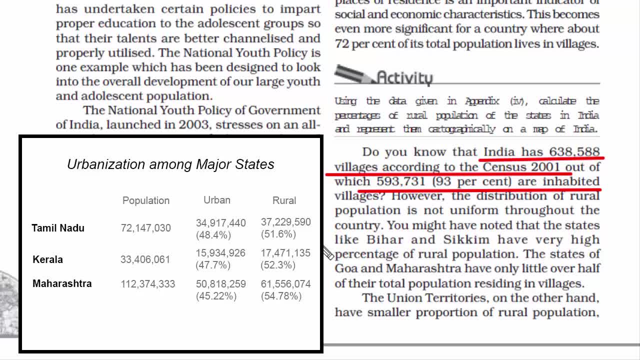 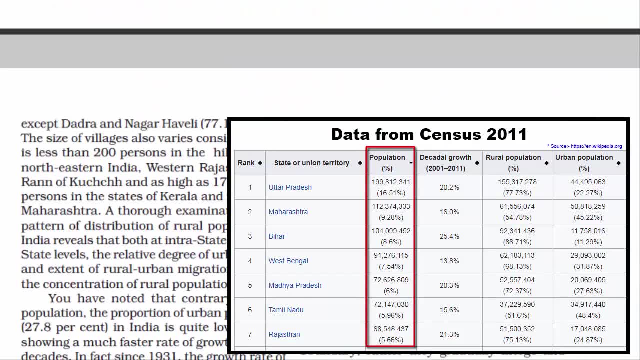 followed now by Kerala, which is at 47.7%, and then Maharashtra, which is at 45.2%. Now, if you look at the top 5 states with highest population, you will notice none of them are part of the most urbanized states. 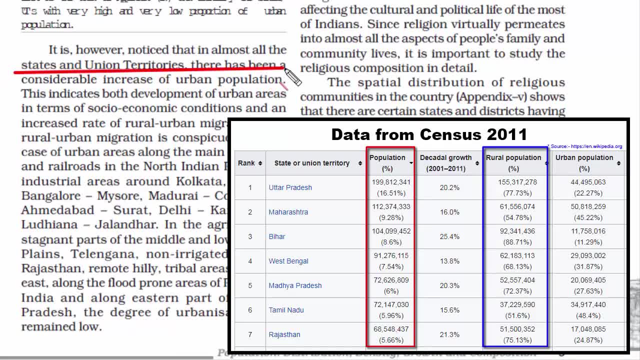 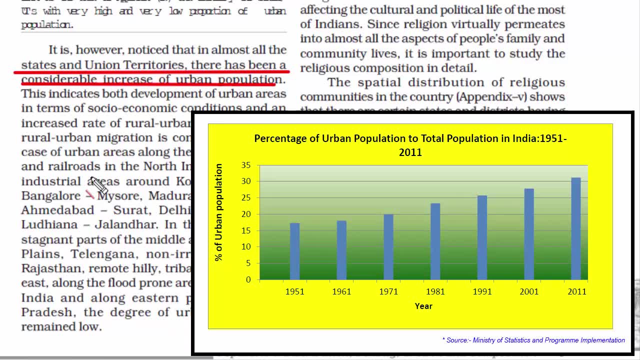 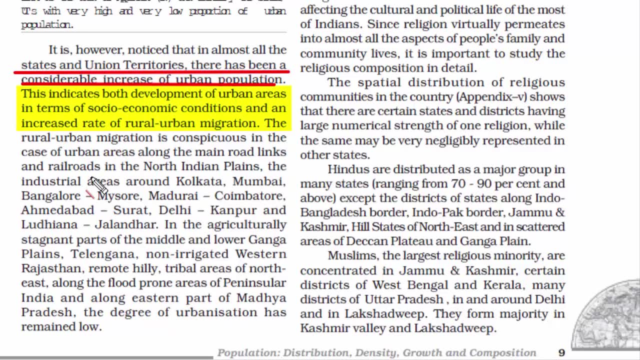 Although these states have high population, but the rural population percentage is more than the urban. However, in almost all states and union territories, there has been a considerable increase of urban population, And that only indicates two things: The urban areas have developed in terms of socio-economic conditions. 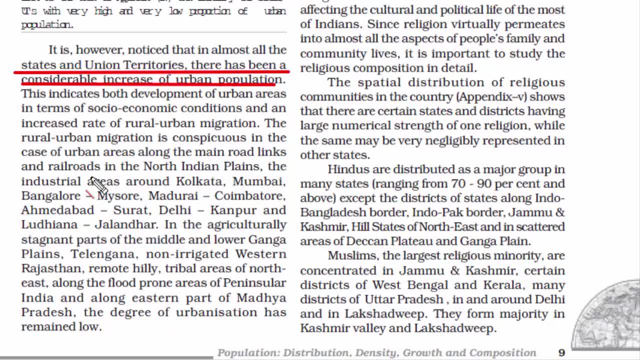 and an increased rate of rural to urban migration. Now I'll tell you a little bit about migration. Migration means movement of anything from one place to another. In this chapter we are dealing with the population, Hence we'll talk about human migration. 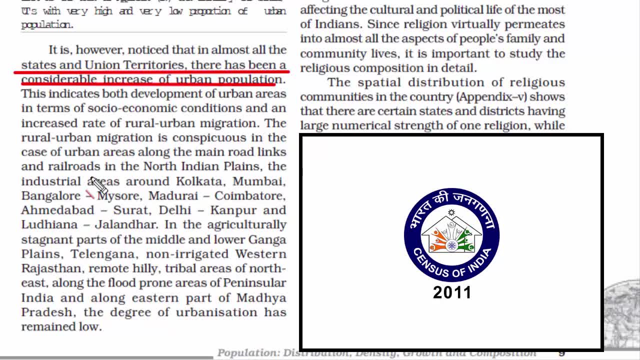 The government of India collects data through census, which is done for every 10 years. The way government takes a note of migrants is by looking at a person's current place of residence. If it is anywhere other than their last residence, that's how migrants are counted. 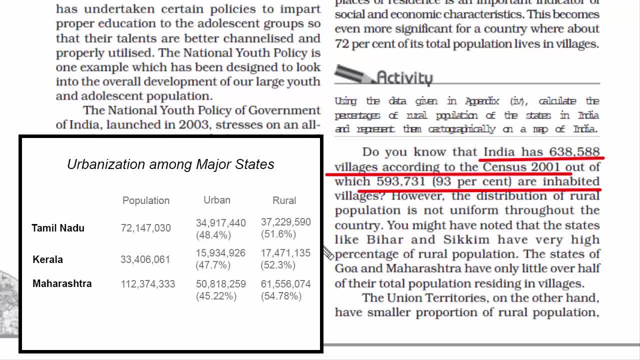 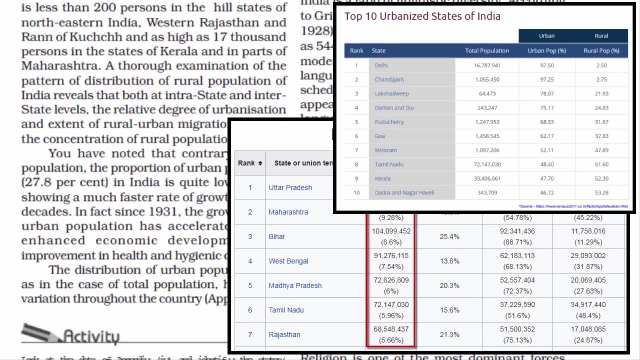 of the population living in urban areas, followed now by Kerala, which is at 47.7%, and then Maharashtra, which is at 45.2%. Now, if you look at the top 5 states with highest population, you will notice none of them are part of the most urbanized states. 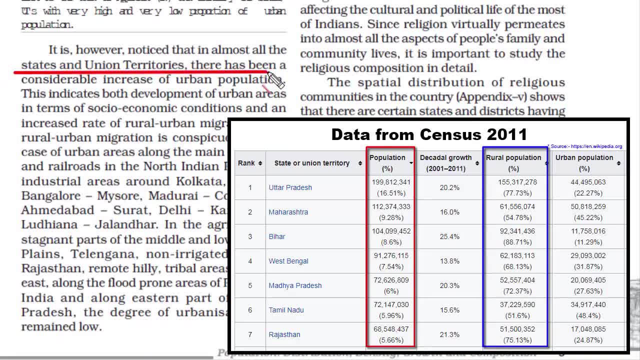 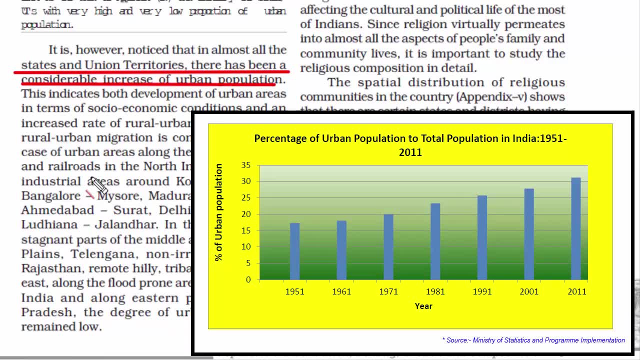 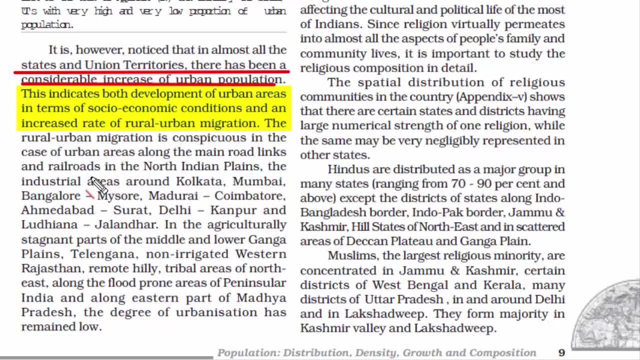 Although these states have high population, the rural population percentage is more than the urban. However, in almost all states and union territories, there has been a considerable increase of urban population, And that only indicates two things: The urban areas have developed in terms of socio-economic conditions. 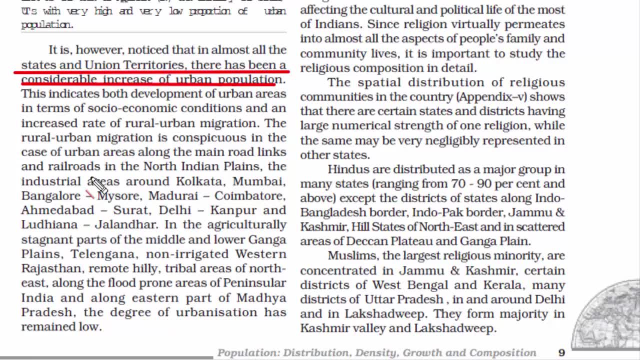 and an increased rate of rural to urban migration. Now I'll tell you a little bit about migration. Migration means movement of anything from one place to another. In this chapter we are dealing with the population, Hence we'll talk about human migration. 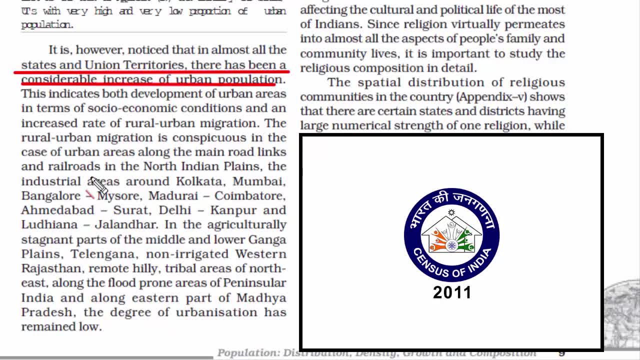 The government of India collects data through census, which is done for every 10 years. The way government takes a note of migrants is by looking at a person's current place of residence. If it is anywhere other than their last residence, that's how migrants are counted. 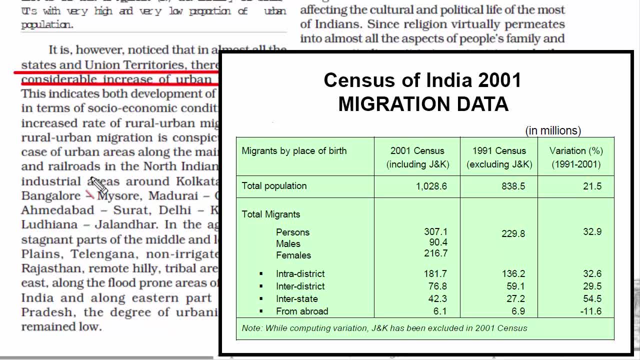 Now at the lowest level of presentation. migration can be seen from four angles. They are intra-district, inter-district, interstate and from abroad. Intra-district migration means movement going on between a single district. Inter-district migration means movement between two or more districts. 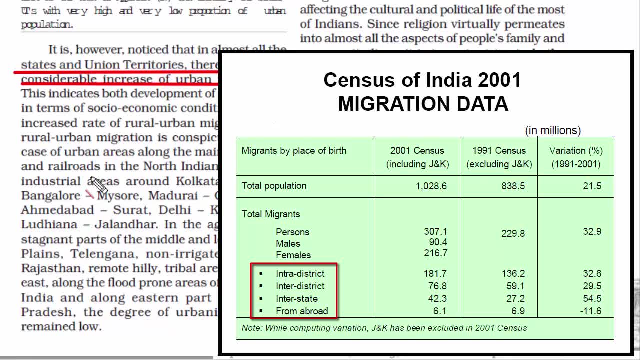 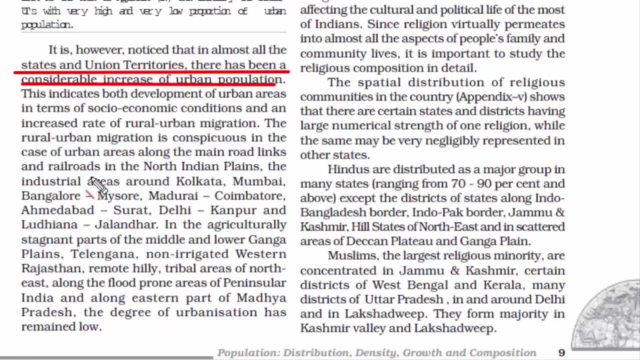 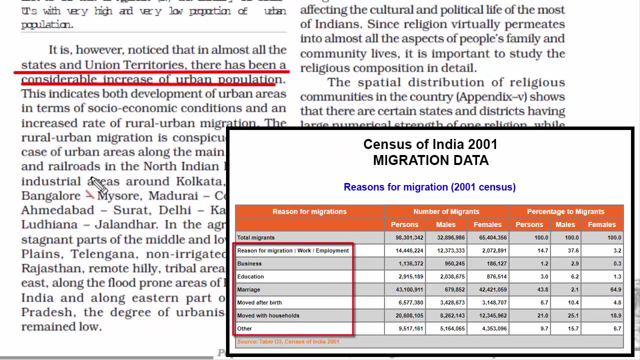 Interstate migration means movement between two or more states. From abroad means the number of migrants from other countries living in India. Now let's look at some of the reasons for migration. Government of India categorizes the reasons into following ways: Employment, business, education, marriage. 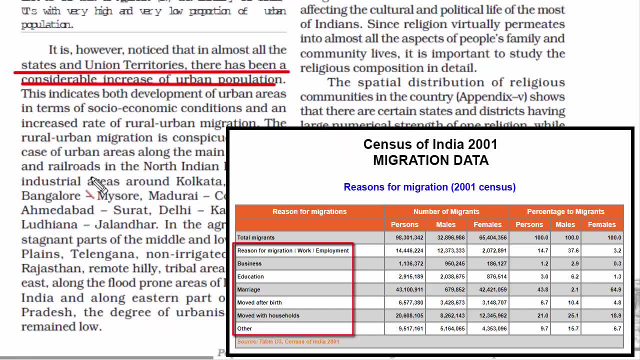 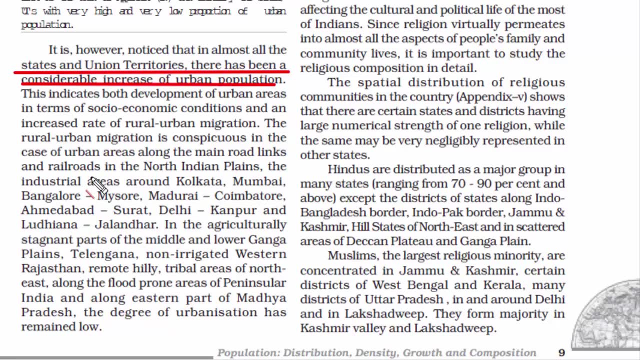 moved after birth, moved with household and others. Marriage was cited as the predominant reason for migration among females. Among males, the most important reason for migration was work and employment. One of the reasons behind rural to urban migration is employment or work. I want you to have a general overview of the rural to urban migration through this map. 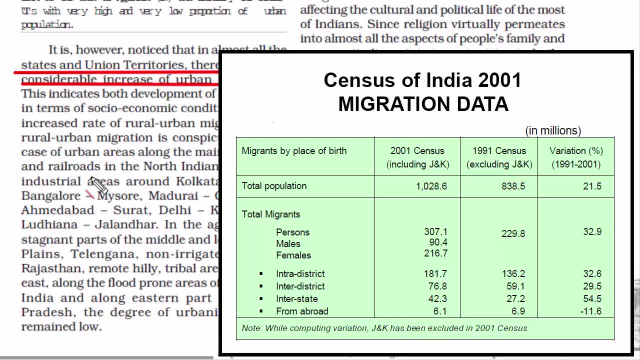 Now, at the lowest level of presentation. migration can be seen from four angles. They are intradistrict, interdistrict, interstate and from abroad. Intradistrict migration means movement going on between a single district. Interdistrict migration means movement between two or more districts. 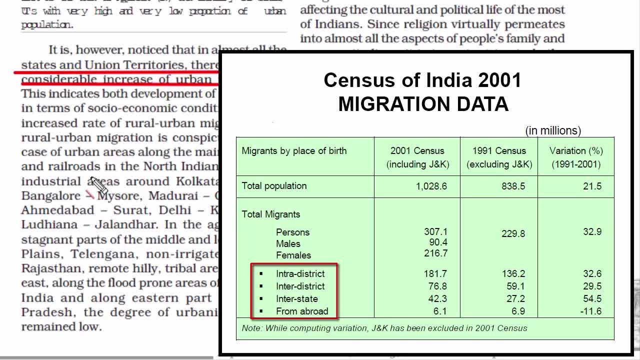 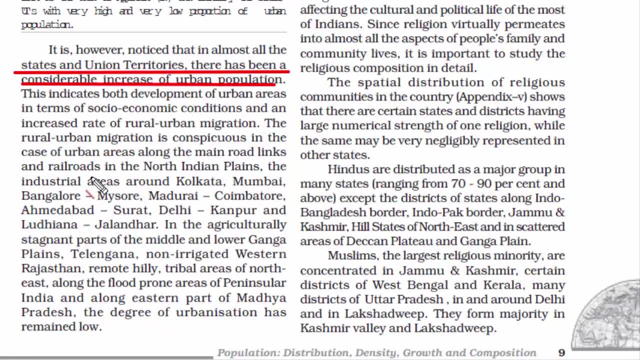 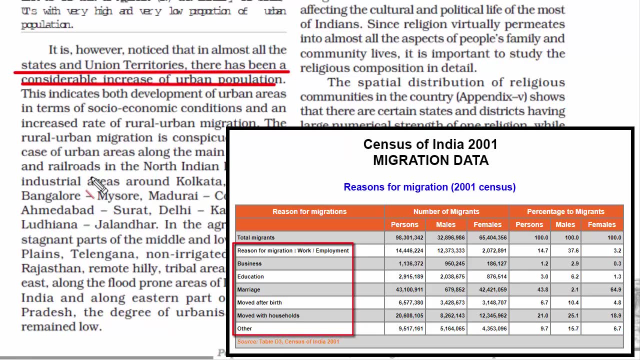 Interstate migration means movement between two or more states. From abroad means the number of migrants from other countries living in India. Now let's look at some of the reasons for migration. Government of India categorizes the reasons into following ways: Work, employment, business, education, marriage, moved after birth, moved with household and others. 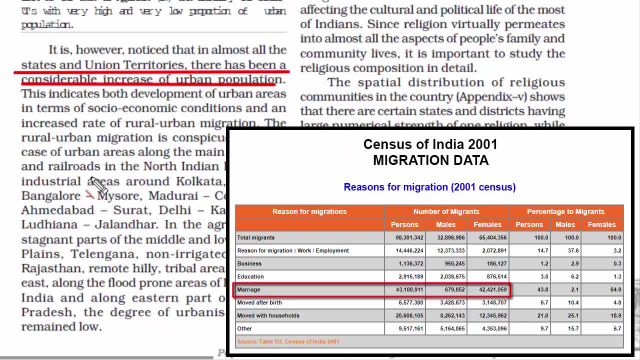 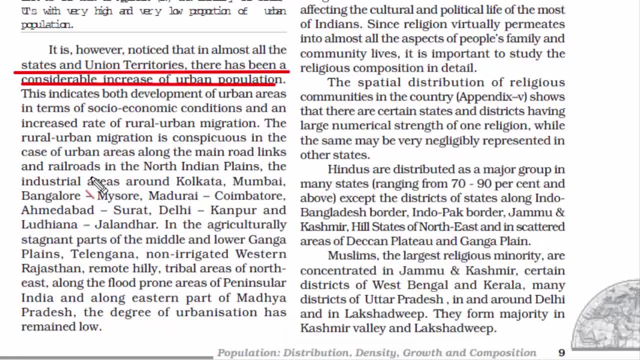 Marriage was cited as the predominant reason for migration among females. Among males, the most important reason for migration was work and employment. One of the reasons behind rural to urban migration is employment or work. I want you to have a general overview of the rural to urban migration. 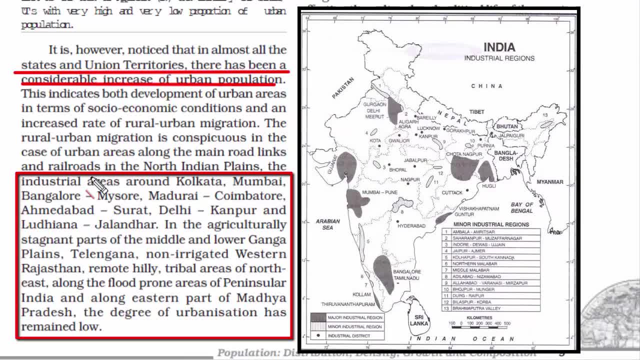 If you look at the industrial regions in India, most of the people migrate to these regions for work and employment. Hence the level of migration in these regions are high. If you look at middle and lower Ganga plains, then region of Telangana. 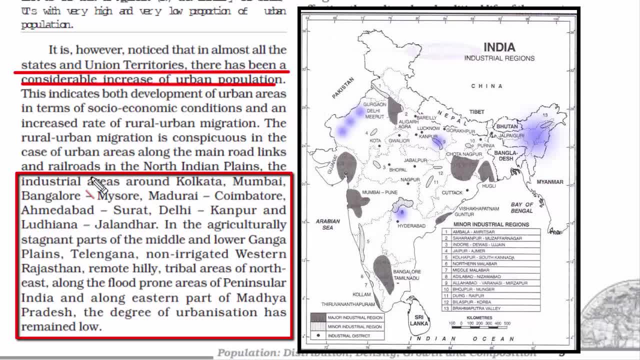 non-irrigated western Rajasthan, remote hilly tribal areas of northeast, along the flood prone areas of peninsular India and along eastern part of Madhya Pradesh. the degree of urbanization has remained low. Now we'll look at the linguistic composition of India's population. 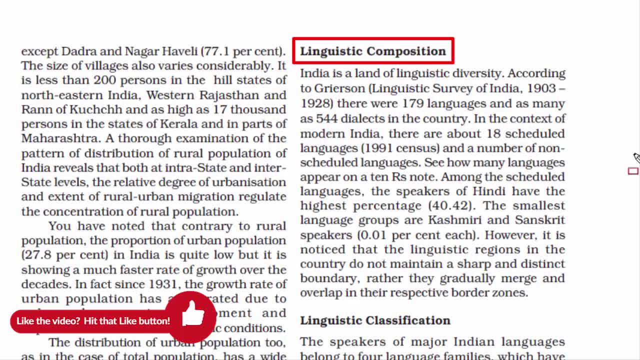 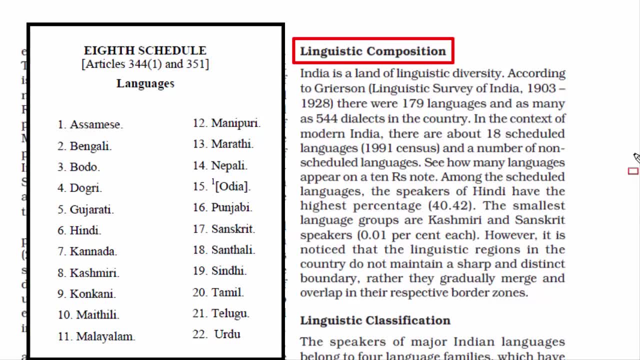 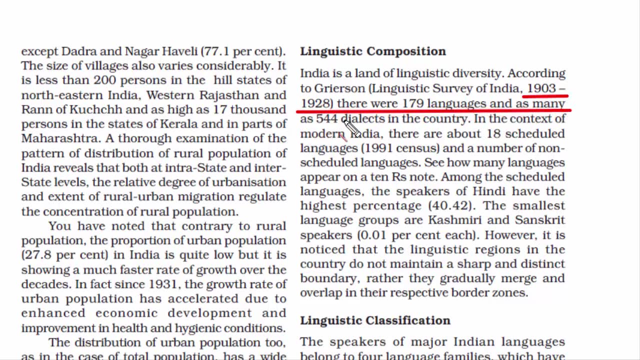 In other words, we'll try to understand the population in terms of the languages they speak. We know that, as per the 8th schedule of the constitution specifies, India has 22 official languages. Here it says there were 179 languages and as many as 544 dialects in the country during 1903 to 1928.. 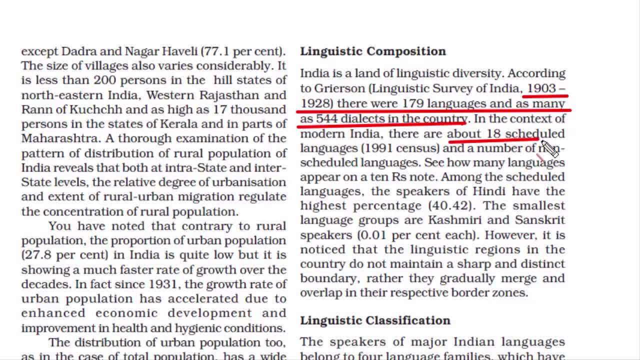 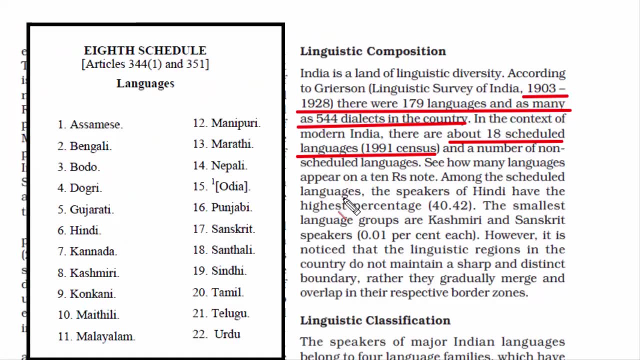 In the context of modern India, there are about 18 scheduled languages as per the 1991 census. These are some old data. presently, as per the 2011 census, There are 22 scheduled languages and 99 non-scheduled languages. That means of the total population of India. 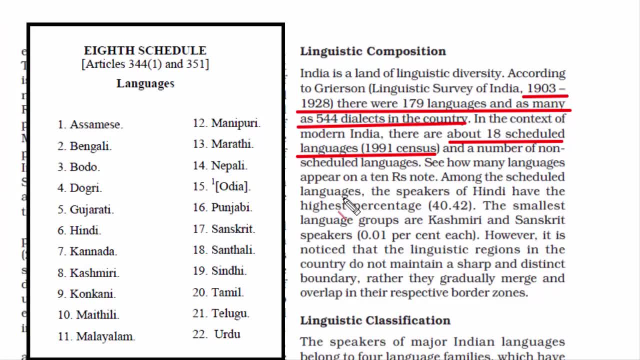 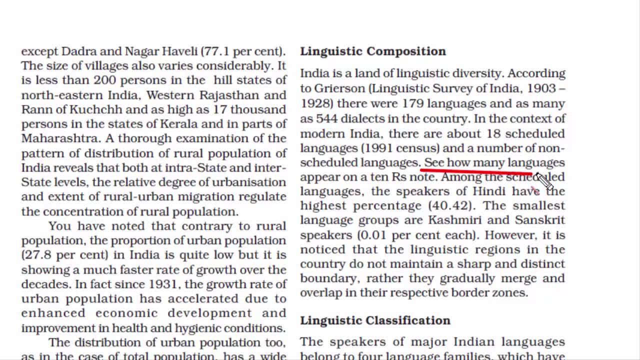 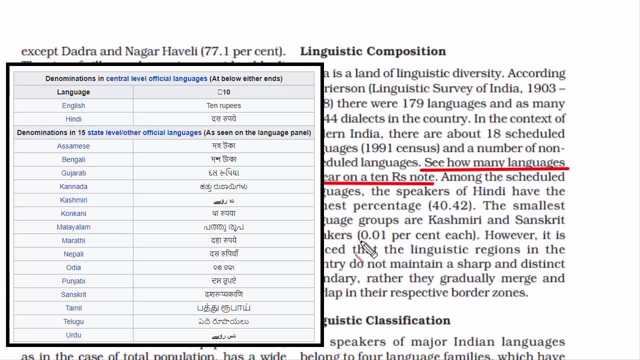 96.71% speak one of the 22 scheduled languages as their mother tongue. The remaining 3.29% speak other languages. Here it says: see how many languages appear on a 10 rupees note. On a 10 rupees banknote, the amount is written in 17 different languages. 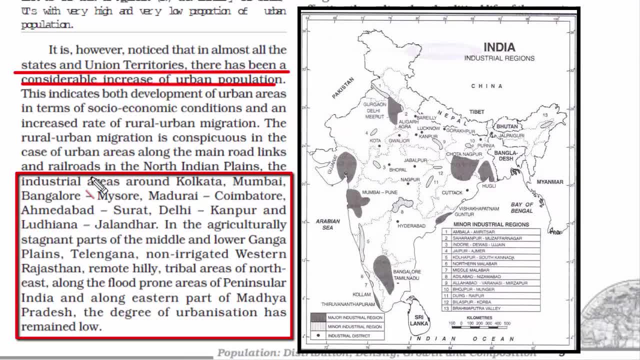 If you look at the industrial regions in India, most of the people migrate to these regions for work and employment. Hence the level of migration in these regions are high. If you look at middle and lower Ganga plains, then region of Telangana. 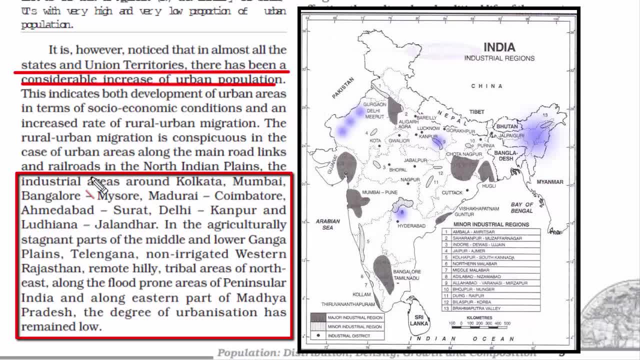 non-irrigated western Rajasthan, remote, hilly tribal areas of northeast, along the flood-prone areas of peninsular India and along eastern part of Madhya Pradesh. the degree of urbanization has remained low. Now we'll look at the linguistic composition of India. 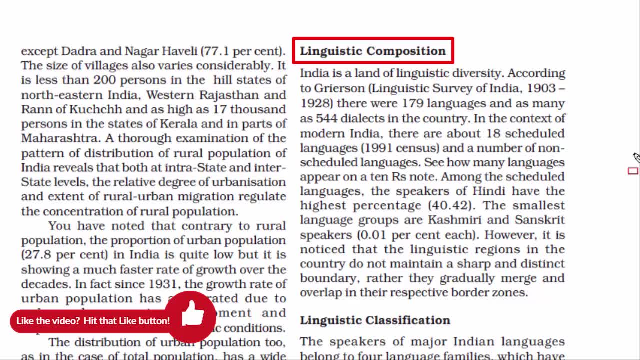 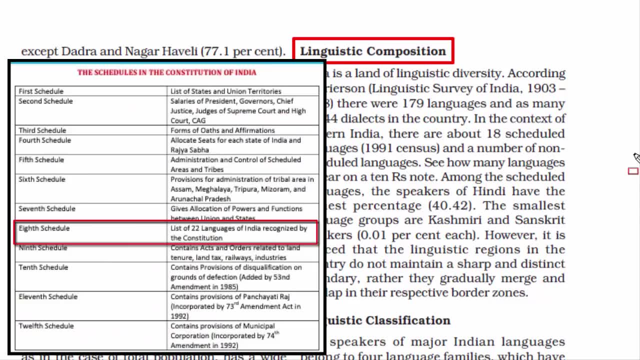 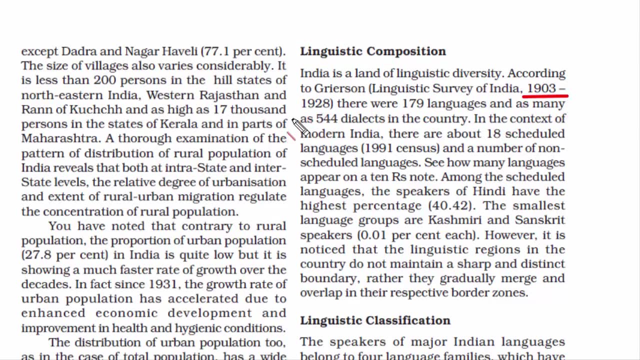 In other words, we'll try to understand the population in terms of the languages they speak. We know that, as per the 8th schedule of the constitution specifies, India has 22 official languages. Here it says there were 179 languages and as many as 544 dialects in the country during 1903 to 1928.. 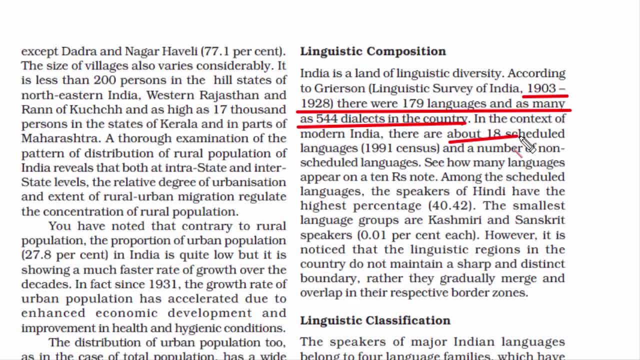 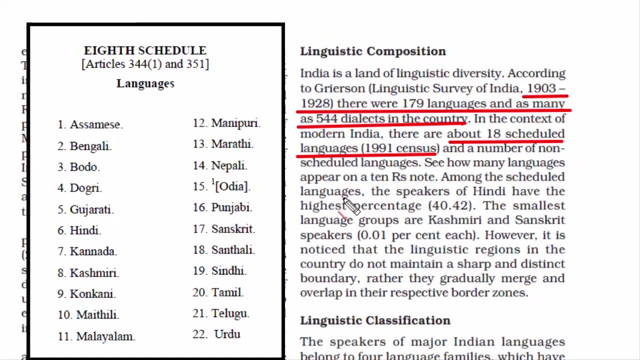 In the context of modern India, there are about 18 scheduled languages as per the 1991 census. These are some old data. presently, as per the 2011 census, There are 22 scheduled languages and 99 non-scheduled languages. That means of the total population of India. 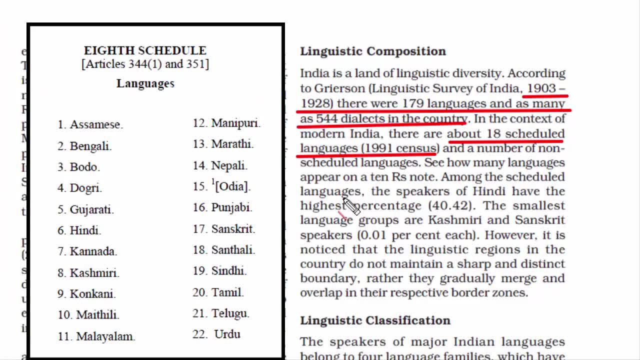 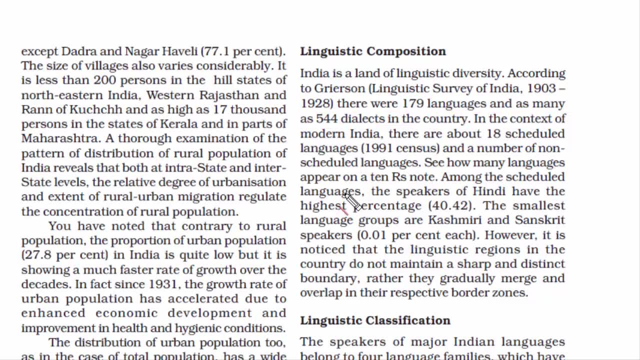 96.71% speak one of the 22 scheduled languages As their mother tongue. the remaining 3.29% speak other languages. Here it says: see how many languages appear on a 10 rupees note. On a 10 rupees bank note. 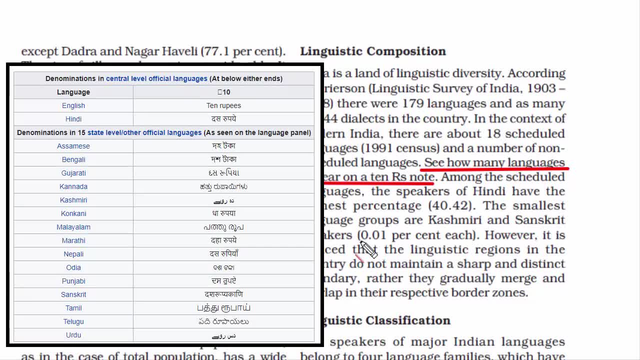 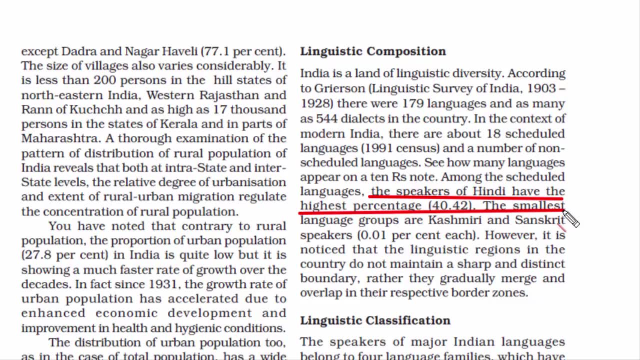 the amount is written in 17 different languages. Here it says: among the scheduled languages, the speakers of Hindi have the highest percentage, that is at 40.42%. The smallest language groups are Kashmiri and Sanskrit speakers, which are at 0.01% each. 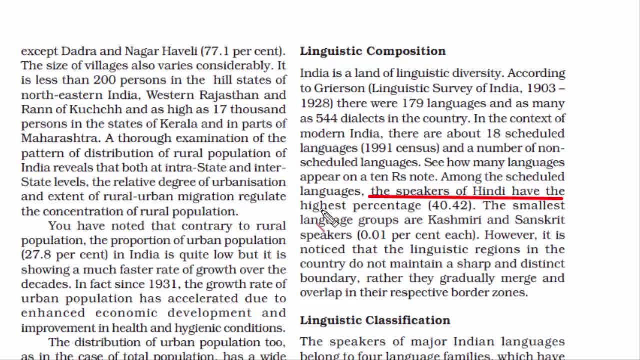 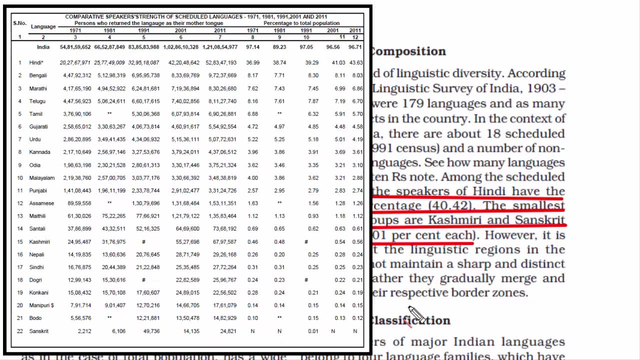 Here it says: among the scheduled languages, the speakers of Hindi have the highest percentage, that is at 40.42%. The smallest language groups are Kashmiri and Sanskrit speakers, which are at 0.01% each. If you look at 2011 census data, 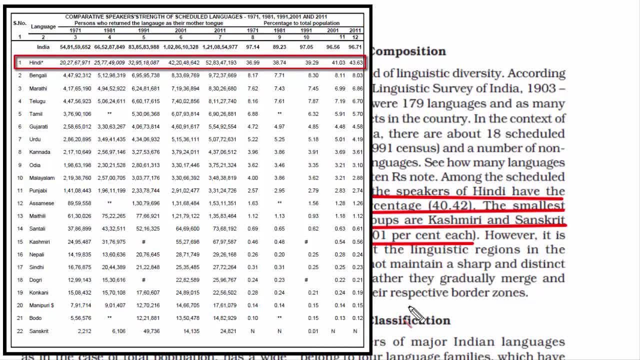 If you look at 2011 census data, Hindi is spoken by majority of the population and Sanskrit is spoken by very few people. However, Kashmiri speakers are large in number. In fact, people who speak Manipuri and Bodo are less in number compared to Kashmiri. 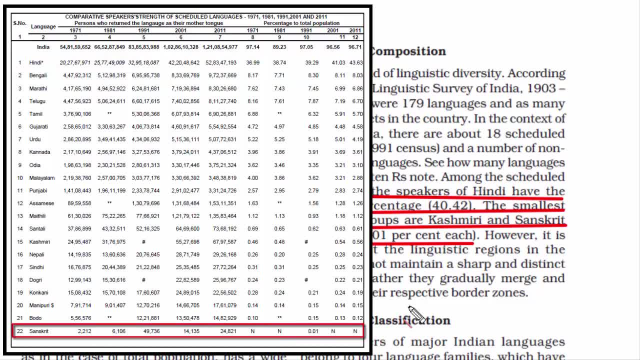 Hindi is spoken by majority of the population and Sanskrit is spoken by very few people. However, Kashmiri speakers are large in number. In fact, people who speak Manipuri and Bodo are less in number compared to Kashmiri. Just have a look at this table. Have an overview of it. That's it. 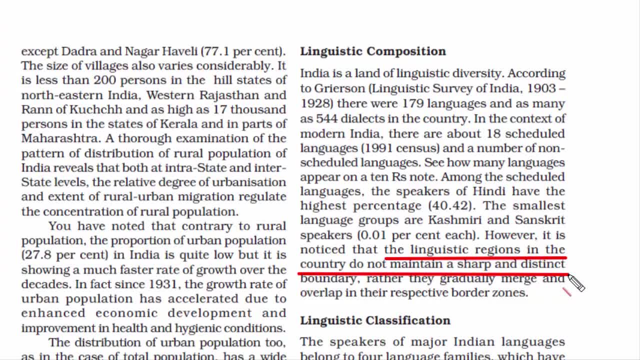 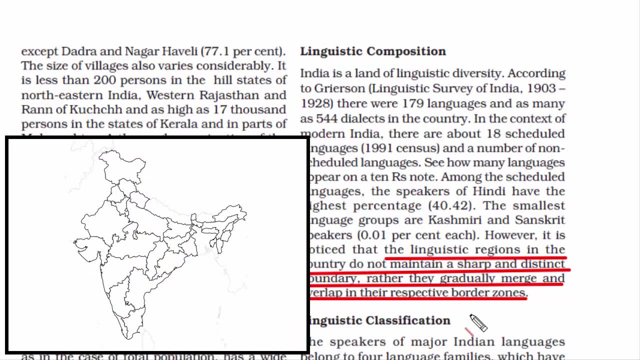 These last lines are important. It says the linguistic regions in the country do not maintain a sharp and distinct boundary. Rather, they gradually merge and overlap in their respective border zones. What it means is when you look at a political map of India, you'll see all these states and their borders right. 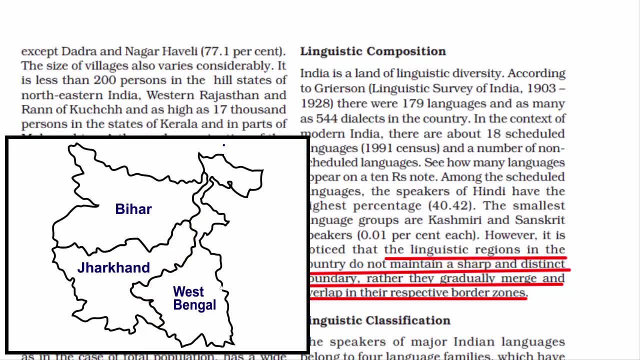 And it is easy for us to say: this side of the border has these kind of people and that side has that kind of people, But then there is no such sharp boundary when it comes to language and culture. Of course, the domicile status will be different. 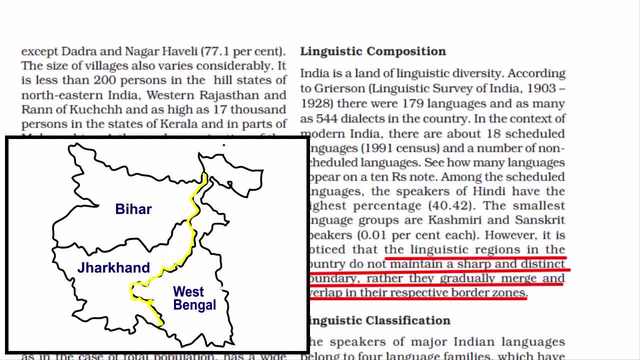 But then there is no such sharp boundary when it comes to language and culture. For example, the western border of West Bengal touches with Bihar. That means the people who reside at the western border of West Bengal will have some cultural and linguistic effect of Bihar. 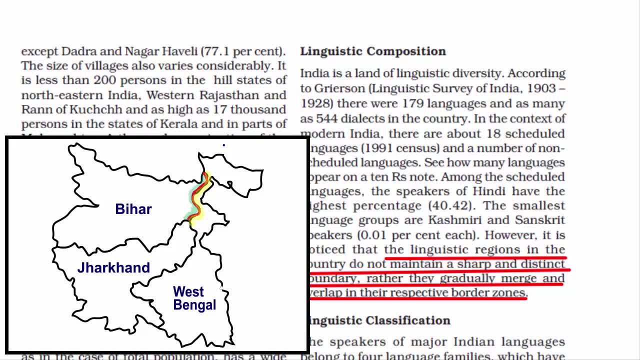 Similarly at the eastern border of Bihar will show some signs and effects of the Bengali culture. However, the authenticity of the culture and language is mostly found at the centre or away from the border zone. You can also call it the gradient phenomena. Gradients means the absence of a clear boundary. 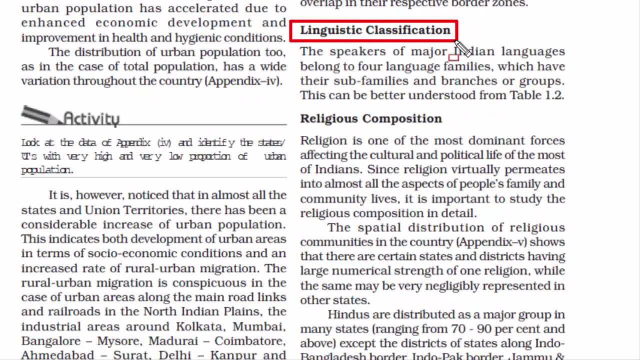 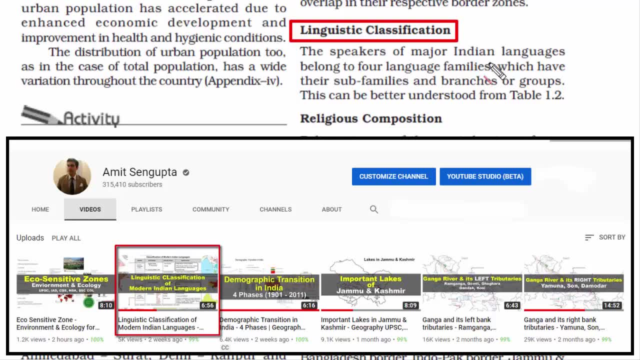 Let's look at the linguistic classification of modern Indian languages. I have made a separate video on this as well, where I have explained the linguistic classification of modern Indian languages. I would recommend you watch that video, because this topic requires some time, hence I chose to make a separate video on it. 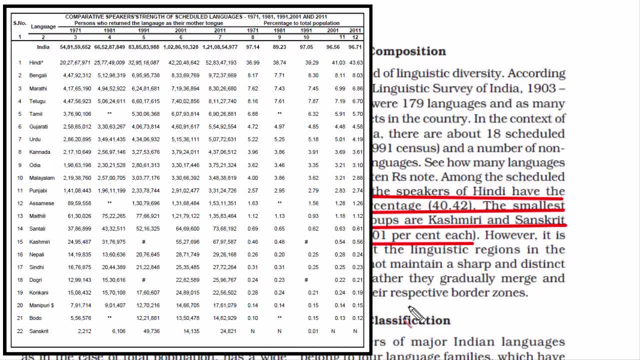 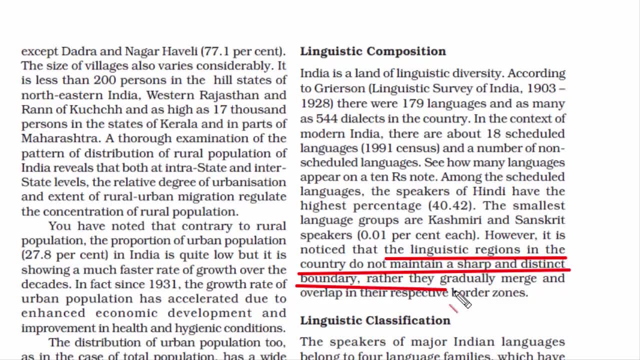 Just have a look at this table, Have an overview of it. That's it. These last lines are important. It says the linguistic regions in the country do not maintain a sharp and distinct boundary. Rather, they gradually merge and overlap in their respective border zones. 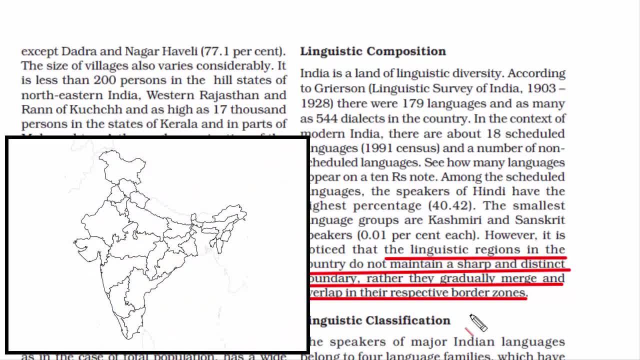 What it means is, when you look at a political map of India, you'll see all these states and their borders right And it is easy for us to say this side of the border has these kind of people and that side has that kind of people. 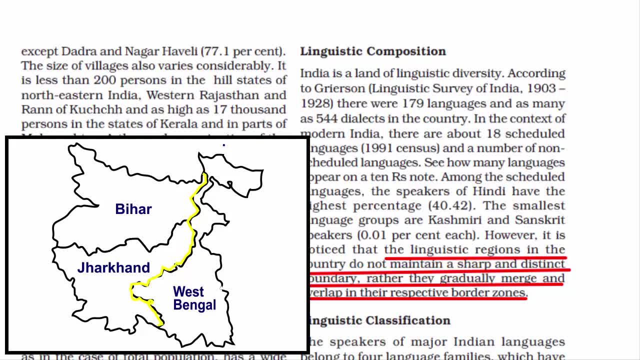 But then there is no such sharp boundary when it comes to language and culture. Of course, the domicile status will be different, But then there is no such sharp boundary when it comes to language and culture. For example, the western border of West Bengal touches with Bihar. 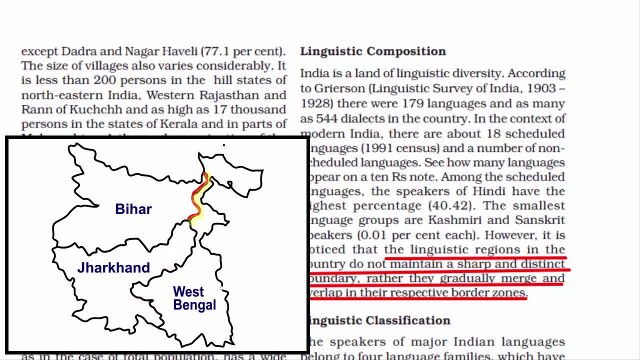 That means the people who reside at the western border of West Bengal will have some cultural and linguistic effect of Bihar. Similarly, at the eastern border of Bihar will show some signs and effects of the Bengali culture. However, the authenticity of the culture and language. 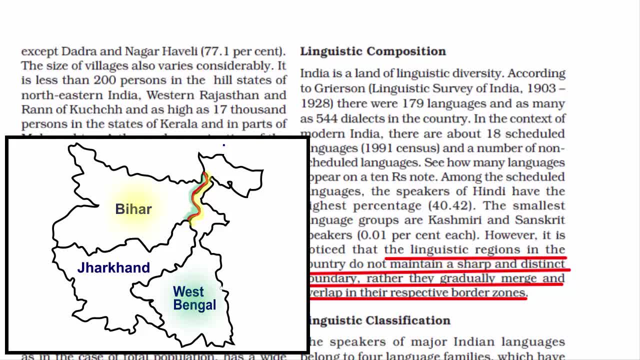 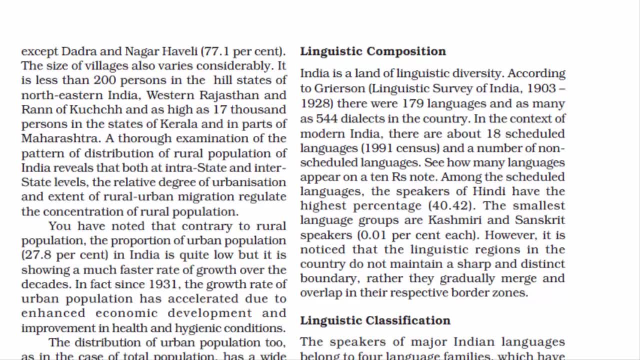 is mostly found at the centre or away from the border zone. You can also call it the gradient phenomena. Gradients means the absence of a clear boundary. Let's look at the linguistic classification of modern Indian languages. I have made a separate video on this as well. 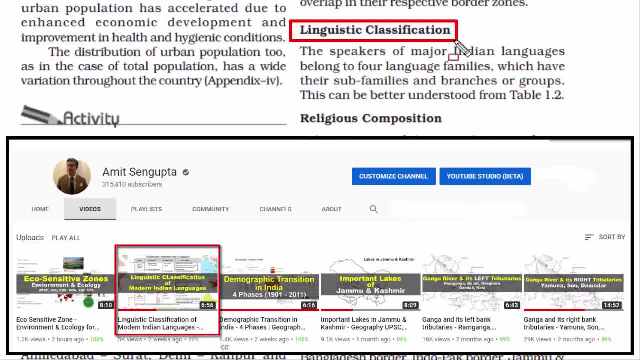 where I have explained the linguistic classification of modern Indian languages. I would recommend you watch that video, because this topic requires some time. hence I chose to make a separate video on it. I have put the link in the description, or you can simply search for linguistic classification of modern Indian languages. 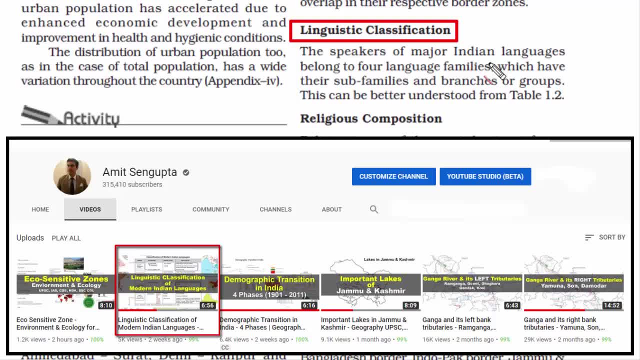 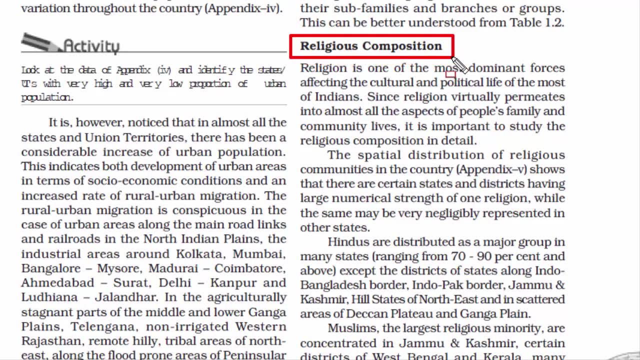 I have put the link in the description, or you can simply search for linguistic classification of modern Indian languages and you will get it. So please watch that video and you will get this topic. Now we will go to the next component of population composition, which is in terms of religious composition. 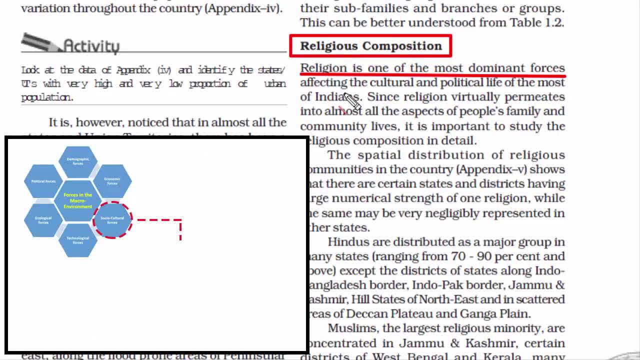 Here it says: religion is one of the most dominant forces affecting the cultural and political life of most Indians. Now, throughout India's history, religion has been an important part of the country's culture. We know that culture and religion are not the same, but then they are very close. 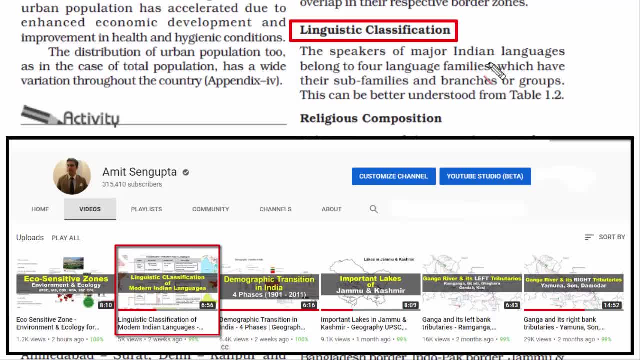 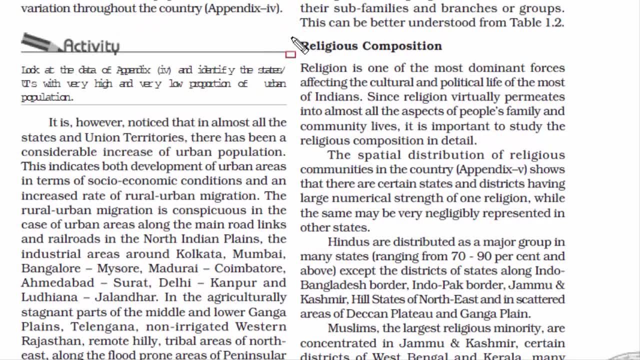 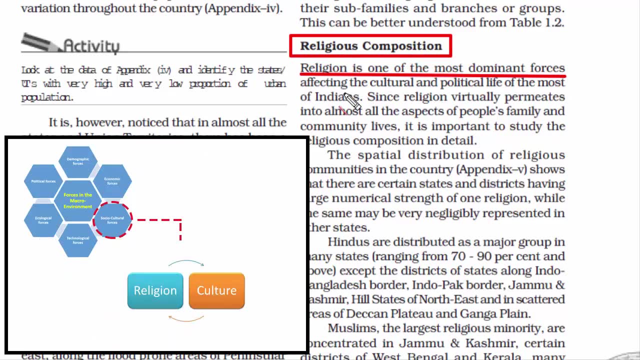 and you will get it. So please watch that video and you will get this topic. Now we will go to the next component of population composition, which is in terms of religious composition. Here it says Religion is one of the most dominant forces affecting the cultural and political life. 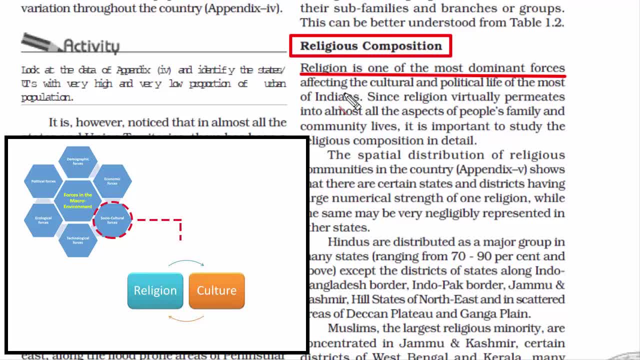 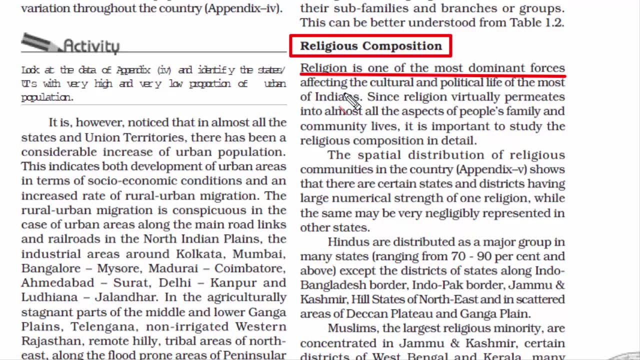 of most Indians. Now, throughout India's history, religion has been an important part of the country's culture. We know that culture and religion are not the same, But then they are very close. Something that has been passed down to your family for generations becomes your culture, right. 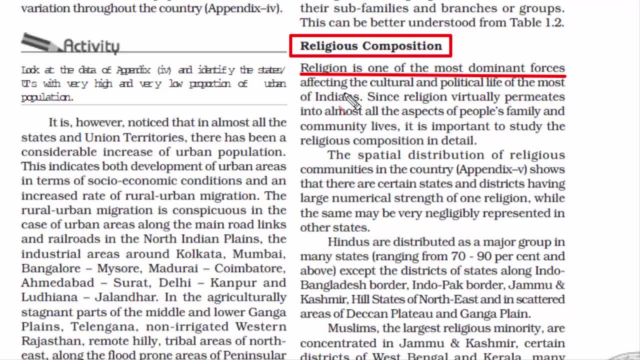 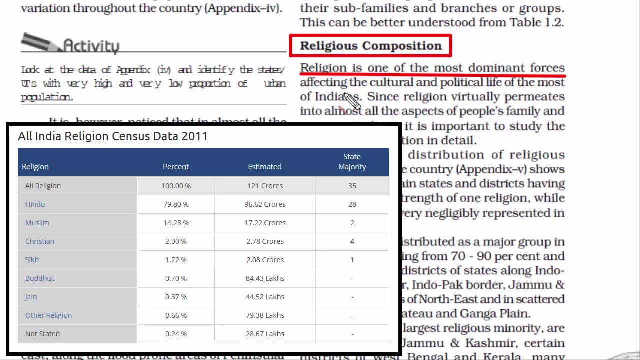 Something that has been passed down to your family for generations becomes your culture, right, And religion is an important ingredient which is passed down for generations in India, And that is how it becomes the most dominant force. Here is the distribution of population of India by religion, as per the 2011 census data. 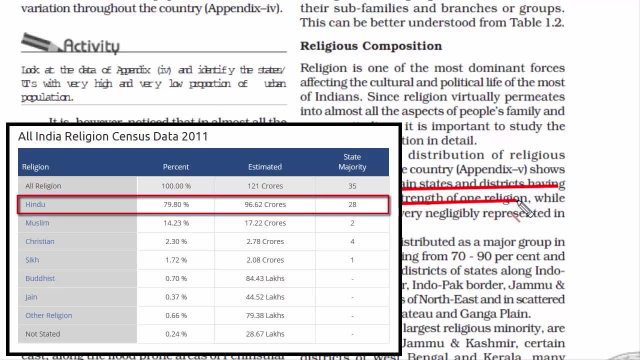 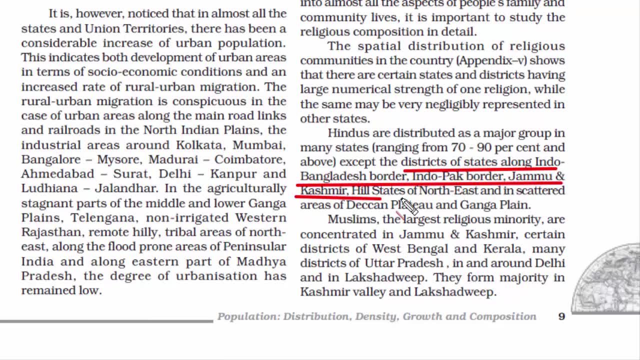 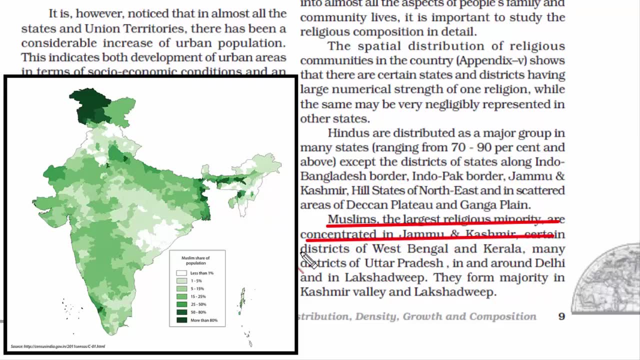 You will notice some states have large numerical strength of one religion, which is Hinduism. But if you look at the border states that are along with India-Bangladesh border and India-Pakistan border, Muslims are quite large in number. States like Jammu and Kashmir, then some districts of West Bengal, Uttar Pradesh and Kerala, even the Lakshadweep island, have Muslim population in majority in the form of minorities. 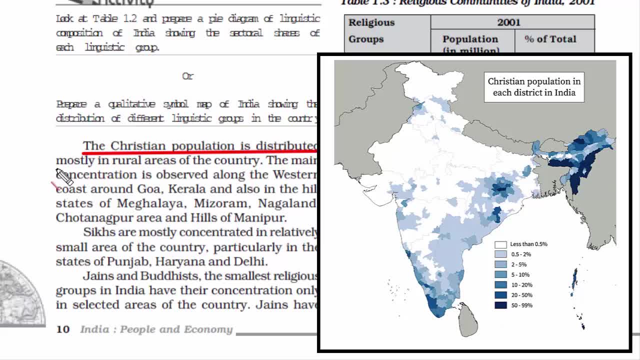 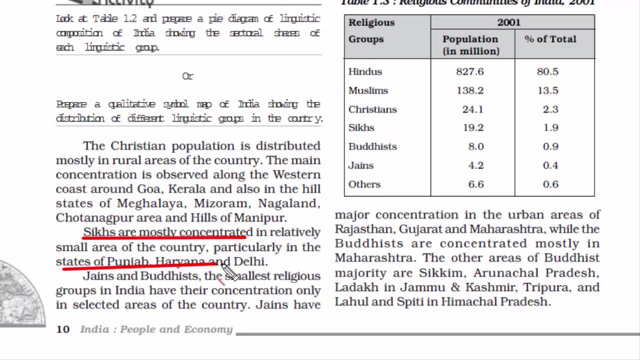 If you look at the Christian population, it is distributed mostly in rural areas of India. However, in states like Kerala, northeastern states, here the Christian population is quite large in number. Then, if you look at the Sikh religion, they are concentrated in small area of the country, particularly in the states of Punjab. 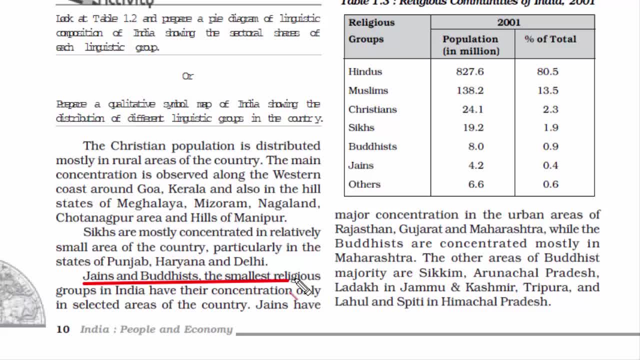 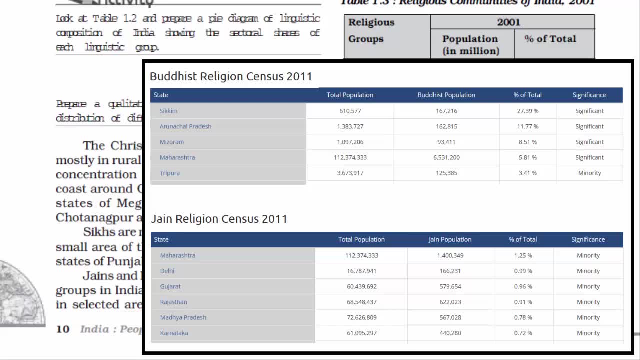 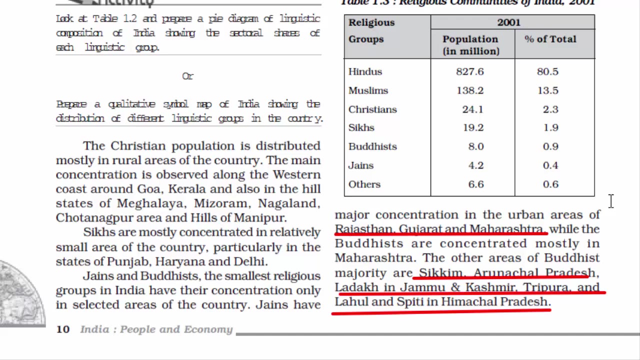 Haryana and Delhi. Then comes Jainism and Buddhism, The smallest religious groups in India. The majority of the Jain population lives in the states of Maharashtra, Rajasthan, Gujarat and Madhya Pradesh. Similarly, Buddhism is largely concentrated in areas of Sikkim, Arunachal Pradesh, Mizoram, Maharashtra, Tripura, Ladakh and Jammu and Kashmir and Himachal Pradesh. 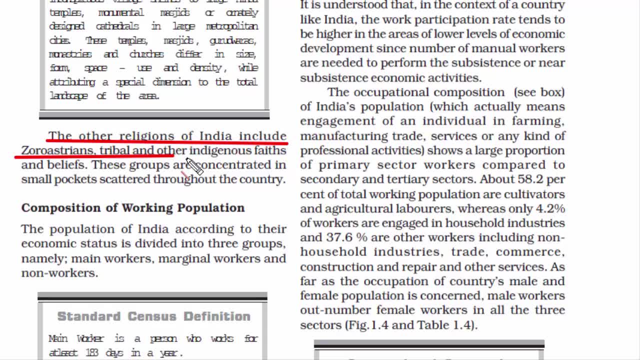 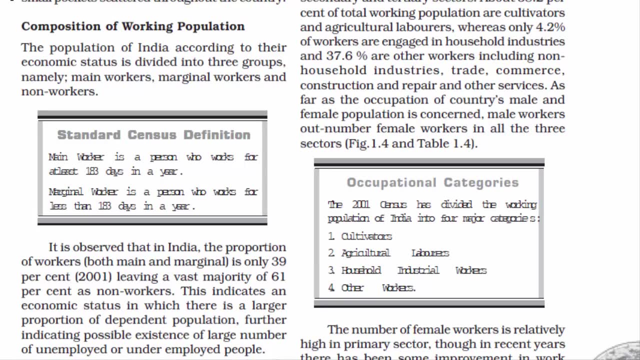 The other religions of India include Zoroastrians, Tribal Muslims and Sikhs. These groups are concentrated in small pockets scattered throughout the country. So this was the religious composition of the Indian population. Now we will go to the next topic: composition of working population. 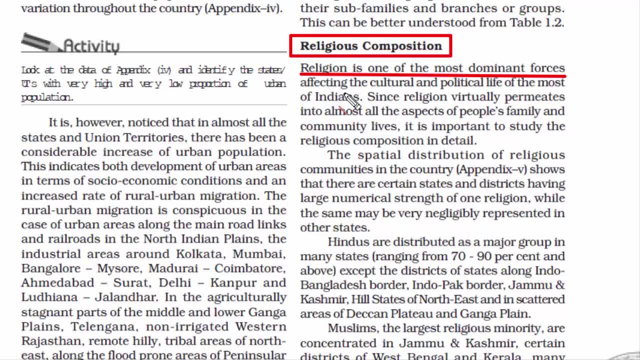 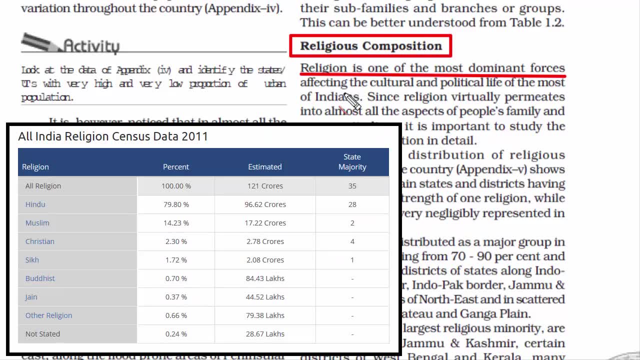 And religion is an important ingredient which is passed down for generations in India And that is how it becomes the most dominant force. Here is the distribution of population of India by religion, as per the 2011 census data. You will notice some states have 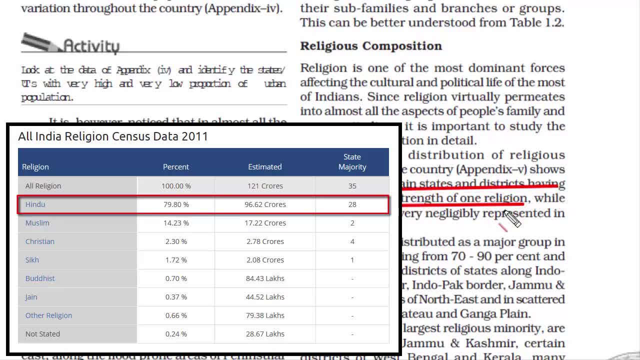 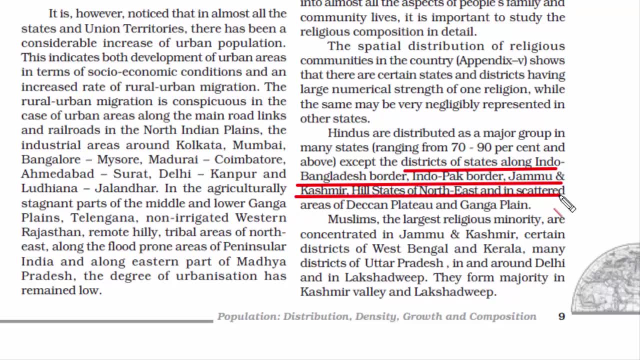 large numerical strength of one religion, which is Hinduism. But if you look at the border states that are along with India-Bangladesh border and India-Pakistan border, Muslims are quite large in number, States like Jammu and Kashmir, then some districts of West Bengal. 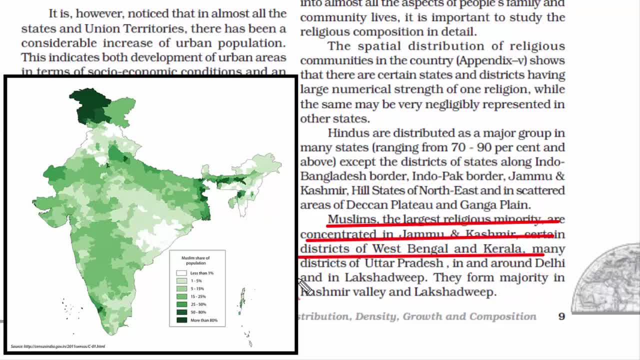 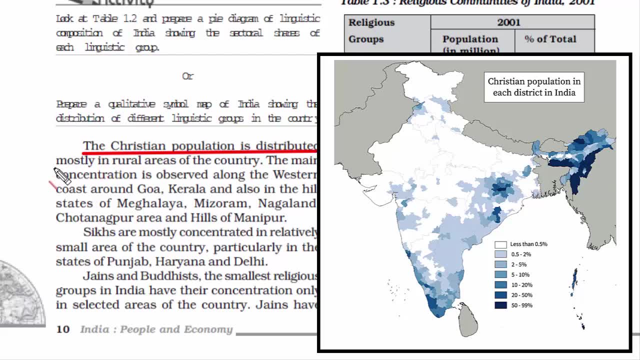 Uttar Pradesh and Kerala, even the Lakshadweep island, have Muslim population in majority in the form of minorities. If you look at the Christian population, it is distributed mostly in rural areas of India. However, in states like Kerala, north-eastern states, here the Christian population is quite large in number. 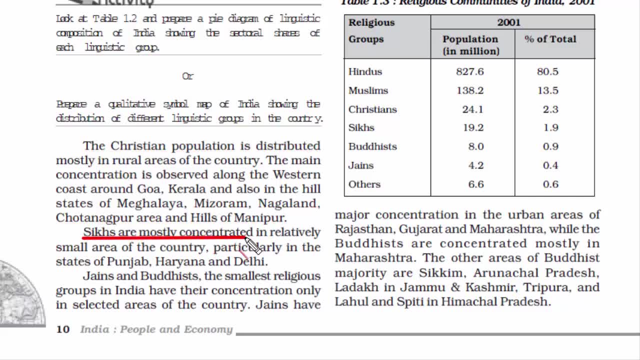 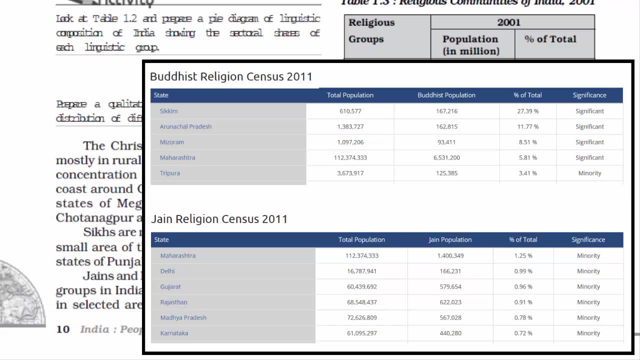 Then, if you look at the Sikh religion, they are concentrated in small area of the country, particularly in the states of Punjab, Haryana and Delhi. Then comes Jainism and Buddhism, the smallest religious groups in India. The majority of the Jain population lives in the states of Maharashtra, Rajasthan, Gujarat and Madhya Pradesh. 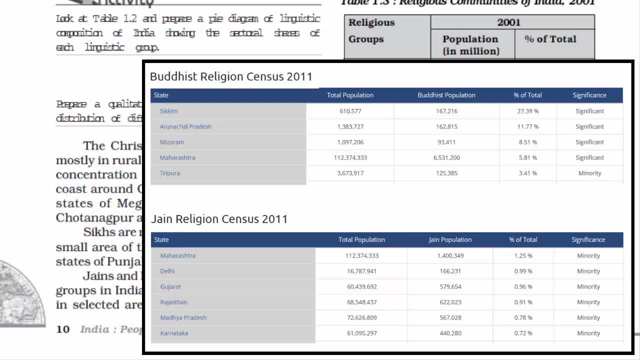 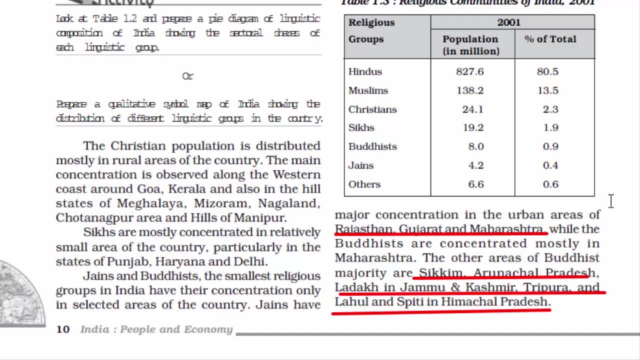 Similarly, Buddhism is largely concentrated in areas of Sikkim, Arunachal Pradesh, Mizoram, Maharashtra, Tripura, Ladakh and Jammu and Kashmir and Himachal Pradesh. The other religions of India include Zoroastrians. 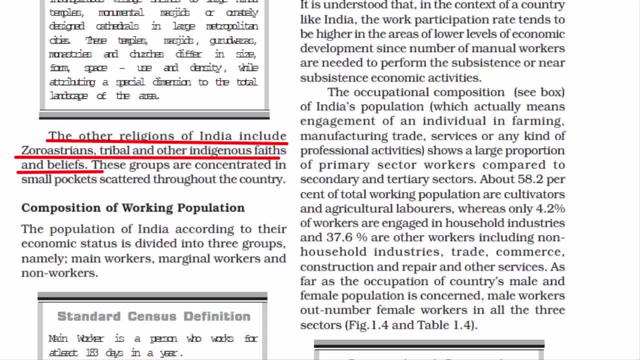 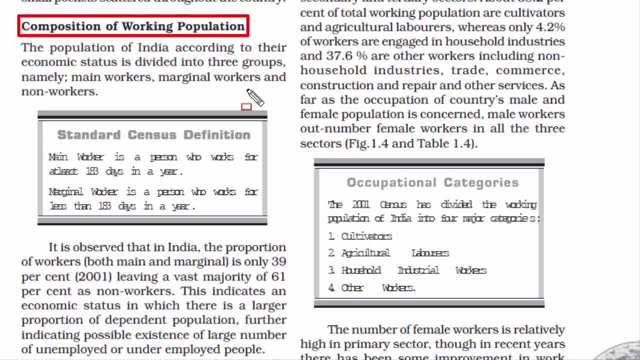 tribal and other indigenous faiths and beliefs. These groups are concentrated in small pockets scattered throughout the country. So this was the religious composition of the Indian population. Now we'll go to the next topic: composition of working population. The moment we see the word working. 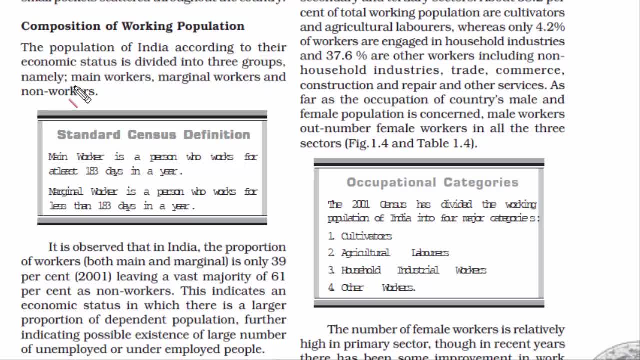 immediately think in terms of the economy. Working population refers to the number of people who are willing and eligible to work and their age has to be 15 years and above, People who are still undergoing studies, housewives and persons above the age of 64. 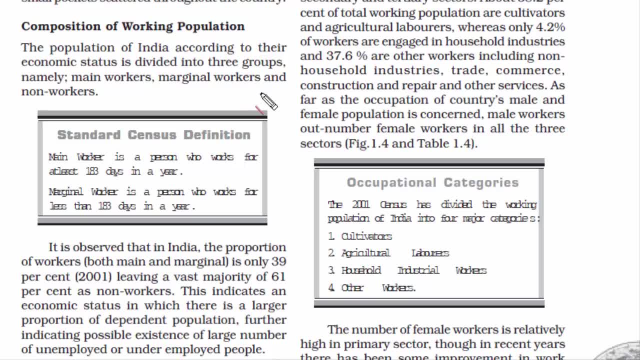 The moment we see the word working, immediately think in terms of the economy. Working population refers to the number of people who are willing and eligible to work, and their age has to be 15 years and above. People who are still undergoing studies, housewives and persons above the age of 64 are not included in the labour force. 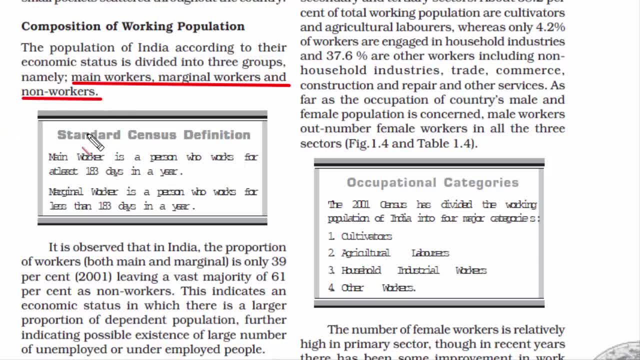 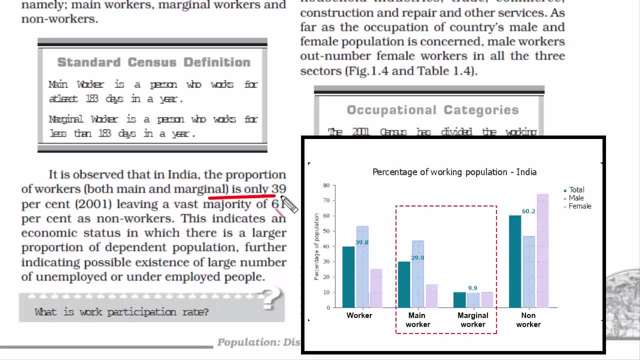 Here it's written. there are basically three types of workers: main workers, marginal workers and non-workers. The proportion of workers, both main and marginal, is only 39% as per the 2001 census, leaving a vast majority of 61% as non-workers. 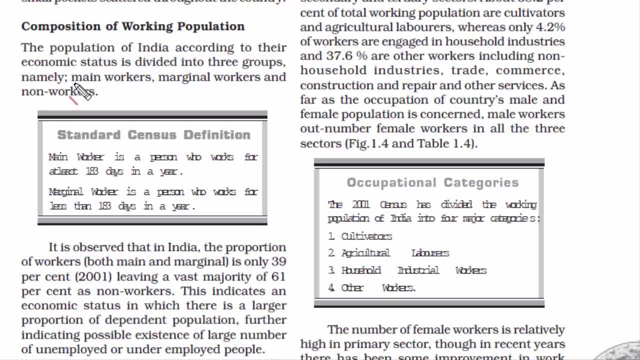 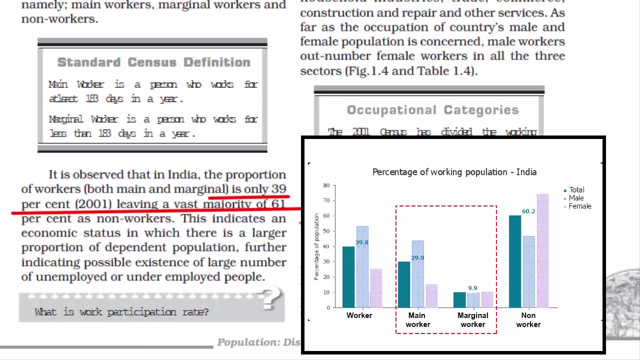 are not included in the labour force. Here it is written. there are basically three types of workers: main workers, marginal workers and non-workers. The proportion of workers, both main and marginal, is only 39% as per the 2001 census, leaving a vast majority of 61% as non-workers. 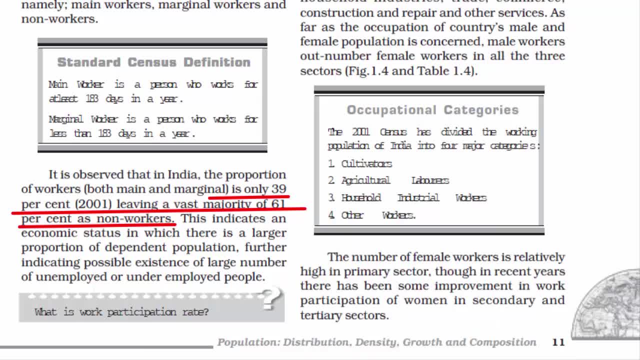 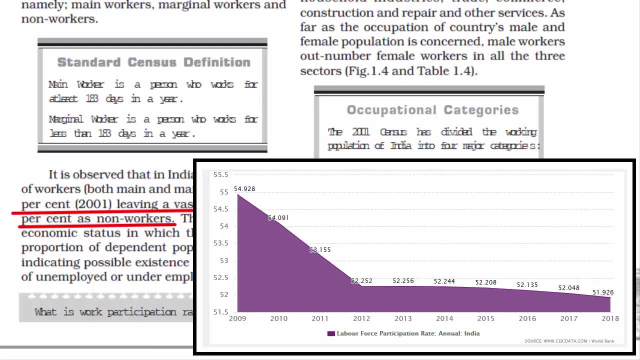 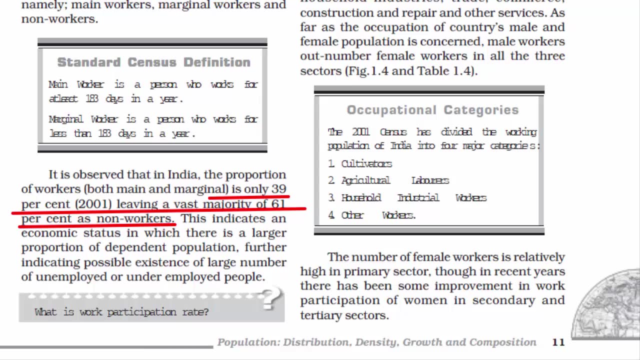 Now this is almost 18 years old data. Currently, the scenario is different. The percentage of non-workers in India is at 49.8% as of 2007-18.. That means almost half of India's working age population is not contributing to any economic activity. 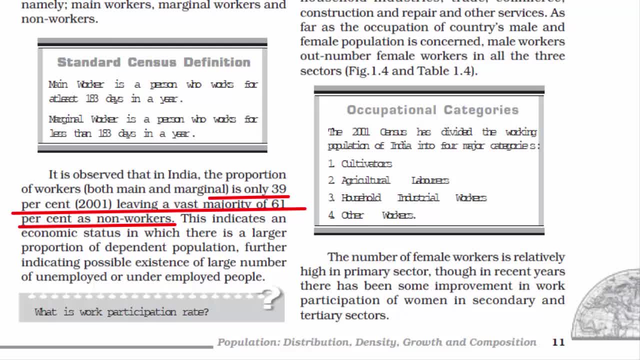 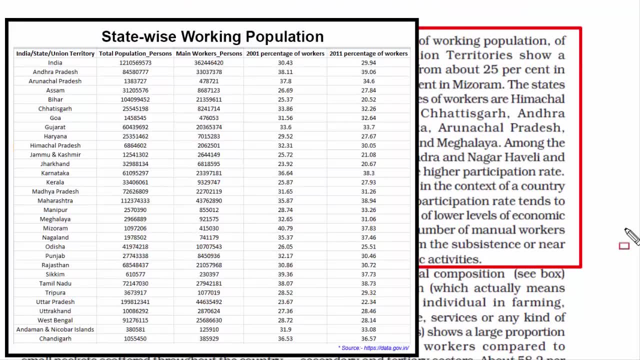 The percentage of non-workers are far more in rural areas than in urban areas. Here is the 2001 and 2011 data on state-wise working population in India. As you can see, in many states the employment rate has dropped or pretty much remained the same. 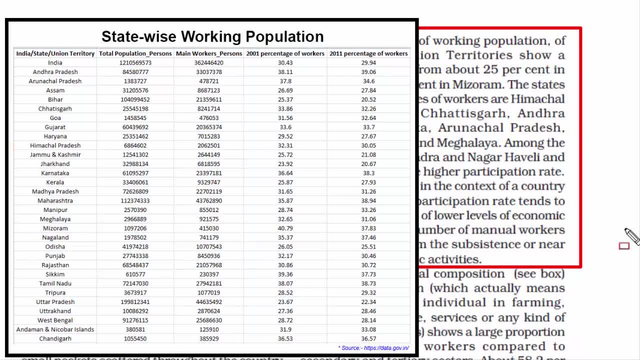 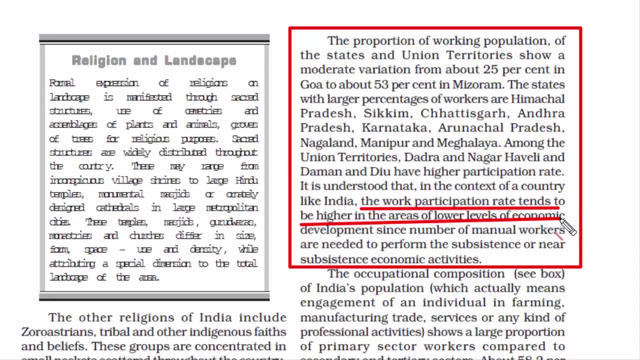 Barely. there is any major change. By looking at the data, you will also realise that the states or the union territories where the working population is high, those states are not really high on any economic development. So the point is, work participation rate tends to be higher. 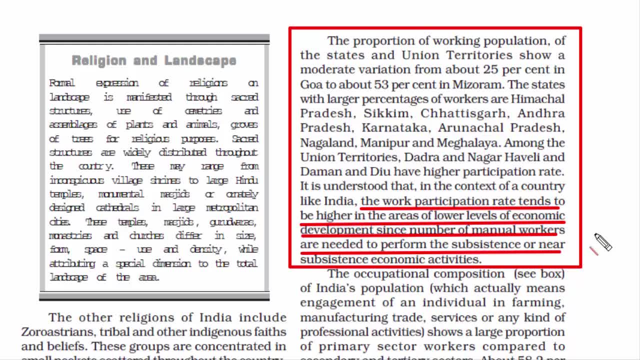 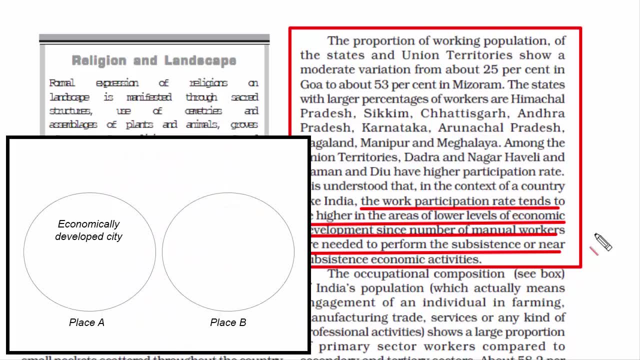 in the areas of lower levels of economic development, Simply because of the requirement of manual labour or workers, If I have to say it in an informal way. suppose there are two places. place A is highly developed, machines are deployed and workers are less who earn decent amount of living. 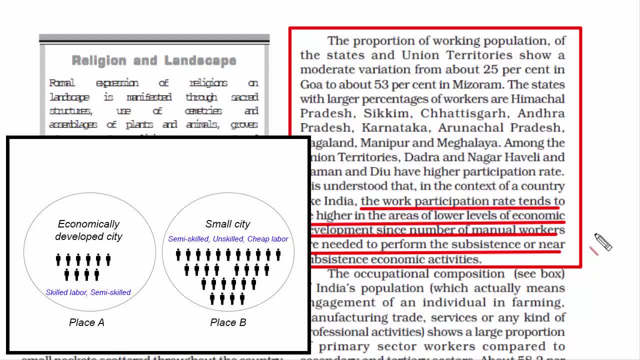 Now place B is not developed, but the number of workers are more doing hard labour at nominal pay. From the above it may look. the work participation rate is high in place B even though there is no development. So this is what the case is when we look at this data. 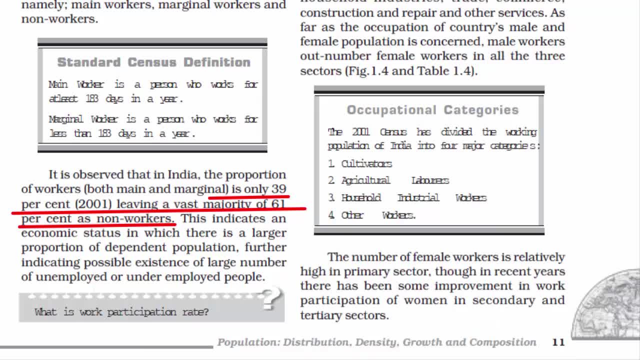 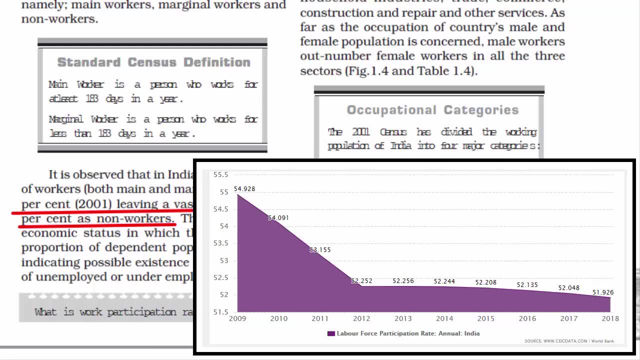 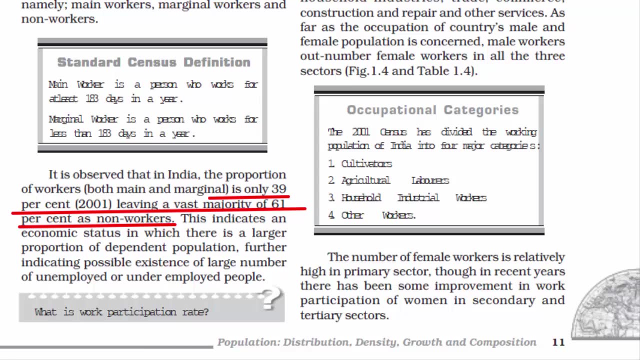 Now this is almost 18 years old data. Currently, the scenario is different. The percentage of non-workers in India is at 49.8% as of 2007-18.. That means almost half of India's working age population is not contributing to any economic activity. 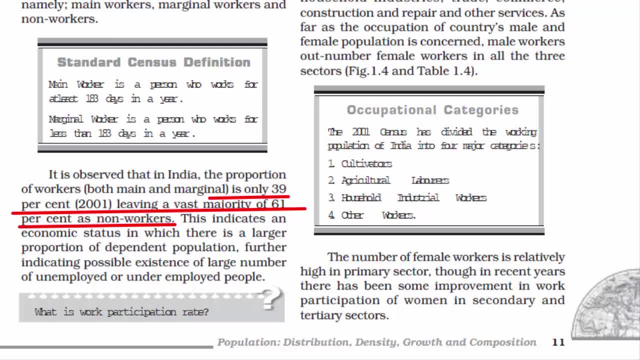 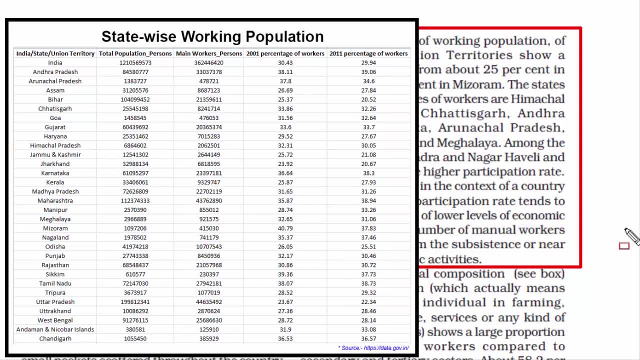 The percentage of non-workers are far more in rural areas than in urban areas. Here is the 2001 and 2011 data on state-wise working population in India. As you can see, in many states the employment rate has dropped or pretty much remained the same. 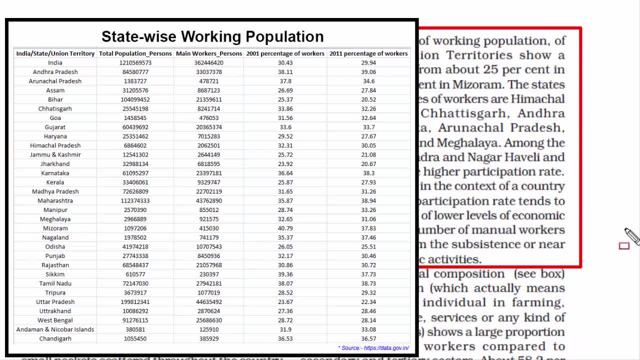 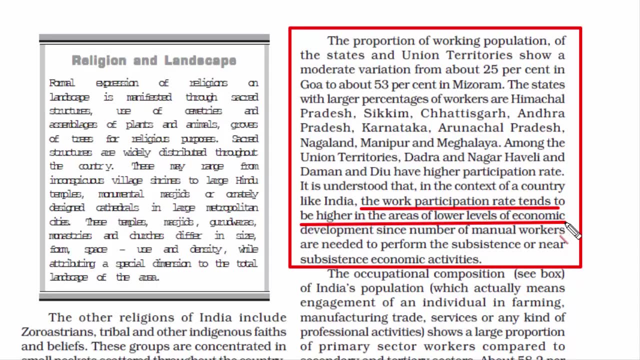 Barely. there is any major change. By looking at the data, you will also realize that the states or the union territories where the working population is high, those states are not really high on any economic development. So the point is, work participation rate tends to be higher in the areas of lower levels of economic development. 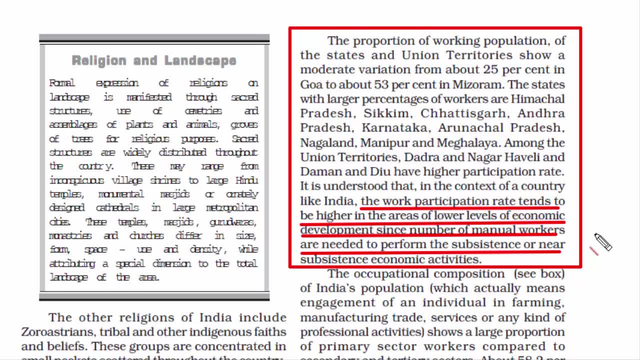 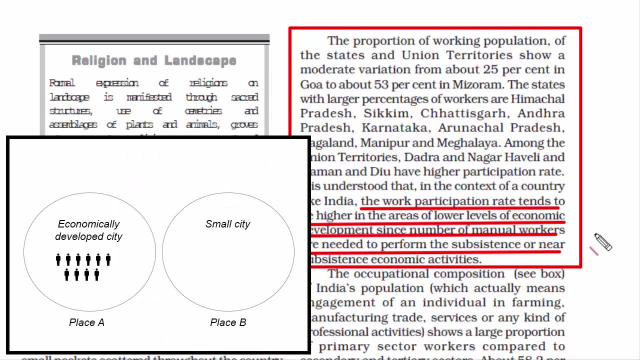 Simply because of the requirement of manual labour or workers, If I have to say it in an informal way. suppose there are two places. Place A is highly developed, machines are deployed and workers are less who earn decent amount of living. Now, place B is not developed, but the number of workers are more, doing hard labour at nominal pay. 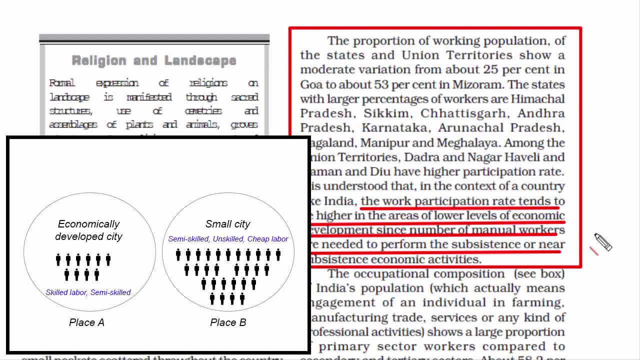 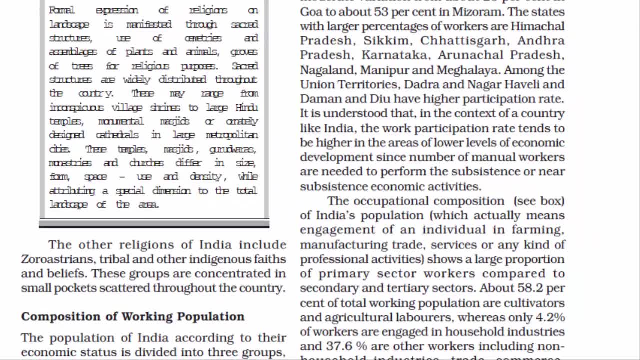 From the above it may look, the work participation rate is high in place B, even though there is no development. So this is what the case is. when we look at this data Now, in a society, you will find different types of occupation, where people are engaged in different sectors of the economy. 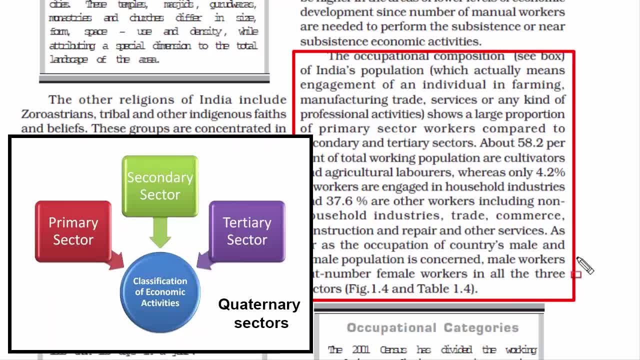 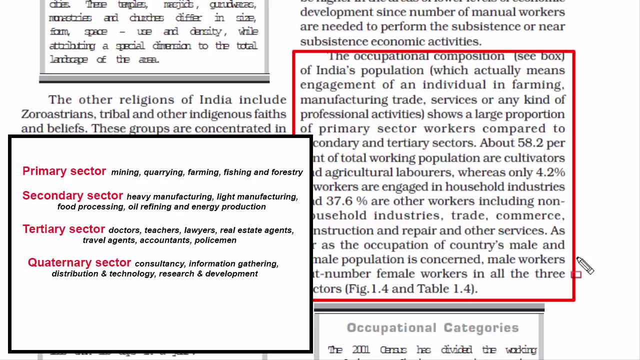 We call them primary, secondary and tertiary and also quaternary sectors. Examples of primary sector works are mining, quarrying, farming, fishing and forestry. Basically in this, the raw materials are processed into a finished product. Similar examples of secondary sector works are heavy manufacturing, light manufacturing. 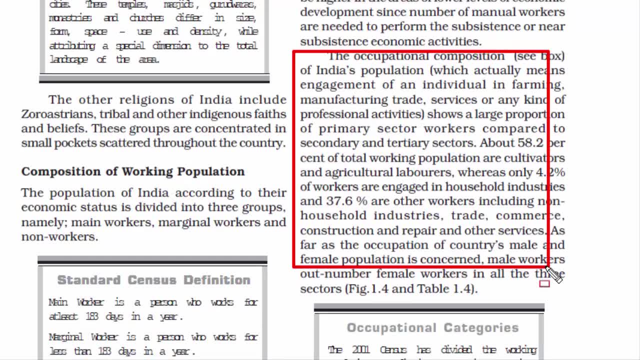 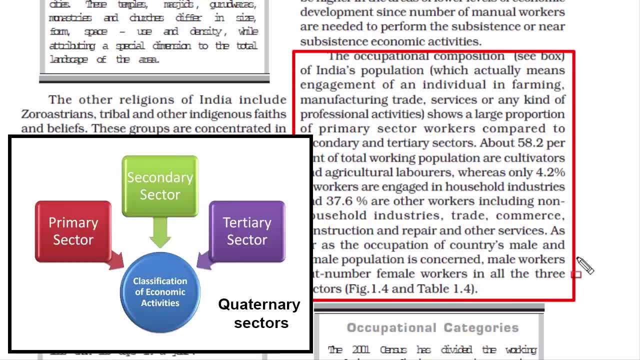 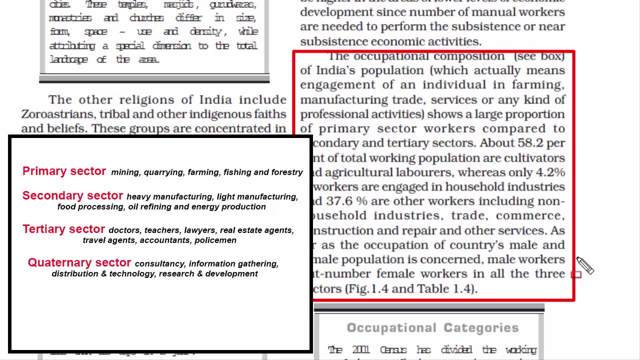 Now, in a society, you will find different types of occupation where people are engaged in different sectors of the economy. We call them primary, secondary and tertiary and also quaternary sectors. Examples of primary sector works are mining, quarrying, farming, fishing and forestry. Basically, in this, the raw materials are processed. 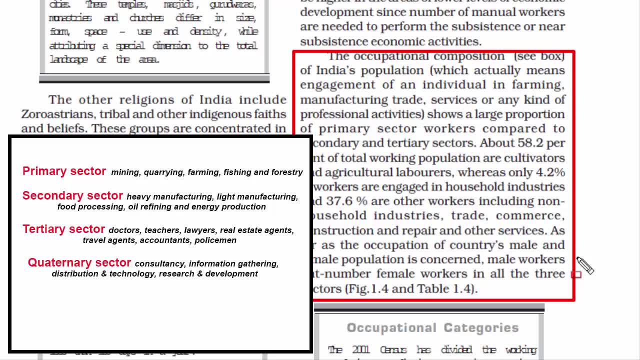 into a finished product. Similar examples of secondary sector works are heavy manufacturing, light manufacturing, food processing, oil refining and energy production. Basically, they take the raw materials produced by the primary sector and process them into manufactured goods. Example of tertiary sector jobs are doctors, teachers, lawyers. 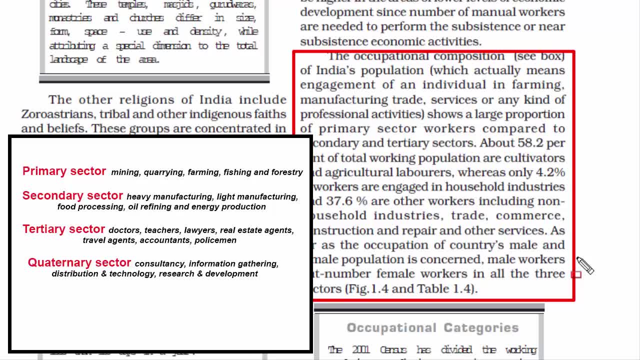 real estate agents, travel agents, accountants, policemen, etc. Basically, they produce intangible value, meaning value that has no physical form, but it generates high percentage of GDP and employment. And quaternary sector includes jobs like consultancy, information gathering, distribution and technology research and development. 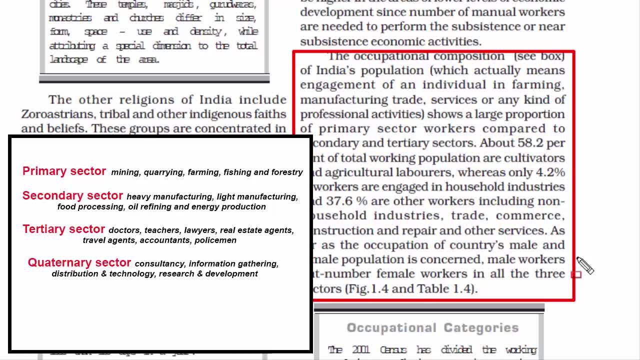 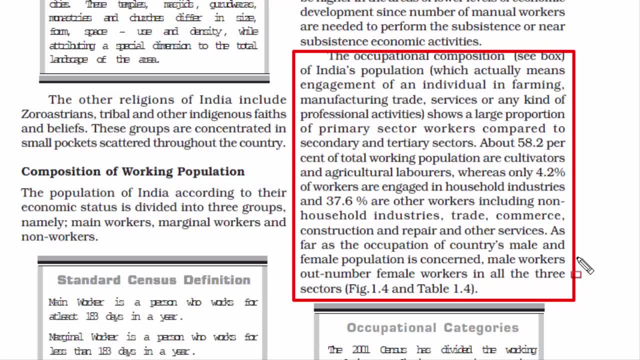 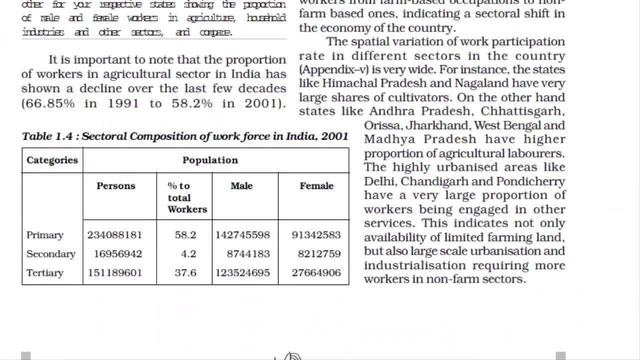 It is basically knowledge based part of the economy which typically includes knowledge oriented jobs. Broadly, these four different sectors are summed up under three broad categories: agricultural sector, industrial sector and service sector. Here in table 1.4, you can see the sectoral composition of a workforce in India. 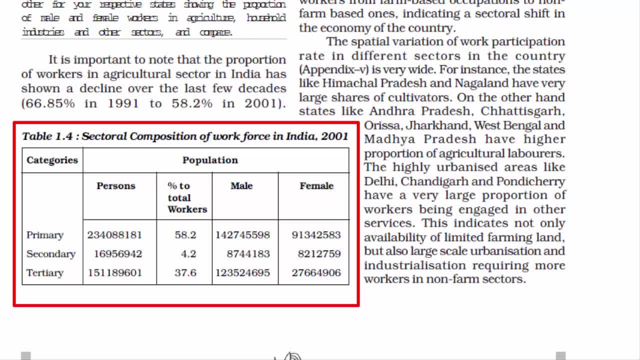 as per 2001 data. This table shows the number of people employed in different sectors And it also shows the male and female contribution. Clearly, male workers have outnumbered female workers in all the three sectors, Since the data is from 2001. 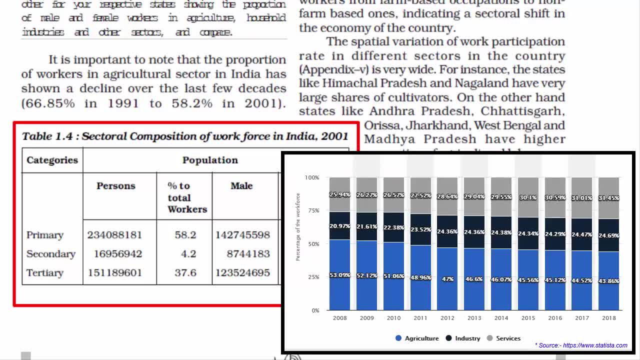 the present distribution of workforce across economic sector is this: You will notice the percentage of workforce in agriculture has reduced, But it has increased in the tertiary and secondary sector. Now I could not find the data on gender wise work contribution in different sectors of the economy. 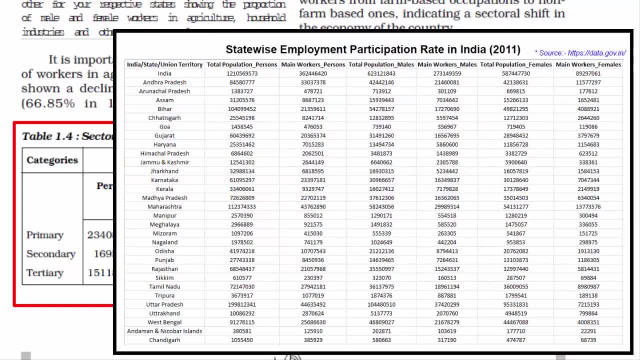 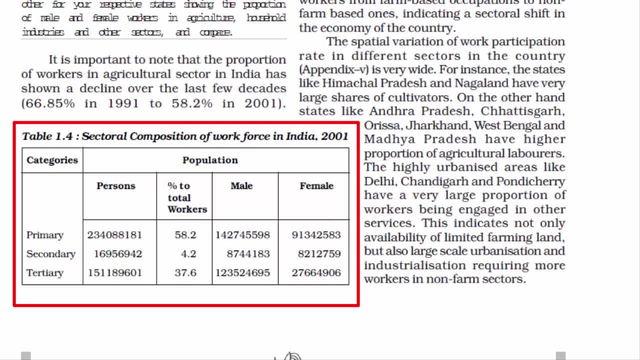 While we do have data on state wise participation of male and female in the economy, but that is not the point. What we need is sector wise male and female contribution in the economy, And in that we can see the trend as to where the women contribute more compared to men. 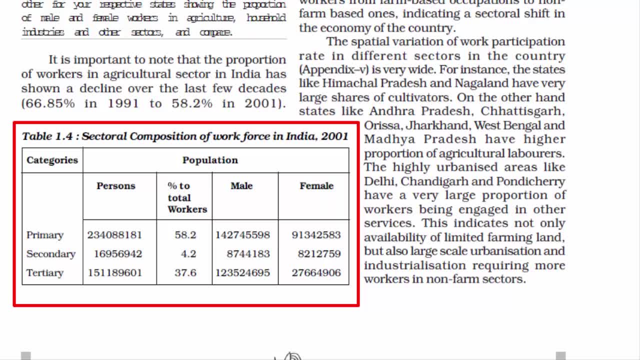 Because in recent years there has been some improvement in work participation of women in secondary and tertiary sector. If you find any data, please paste the link in the comment section so that people can look at it. Here is a map of India that shows the agricultural clusters. 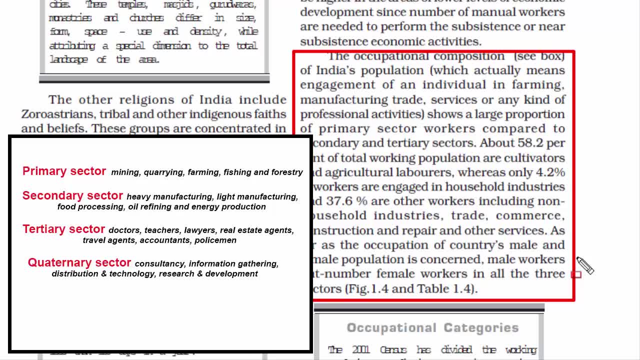 food processing, oil refining and energy production. Basically, they take the raw materials produced by the primary sector and process them into manufactured goods. Examples of tertiary sector jobs are doctors, teachers, lawyers, real estate agents, travel agents, accountants, policemen, etc. 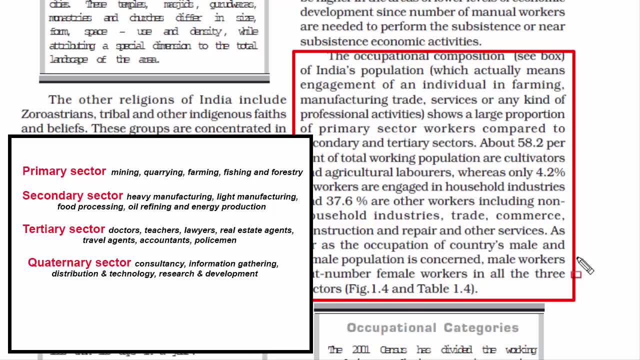 Basically, they produce intangible value, meaning value that has no physical form, But it generates high percentage of GDP and employment. And quaternary sector includes jobs like consultancy, information gathering, distribution and technology research and development. It is basically knowledge based part of the economy, which typically includes knowledge oriented jobs. 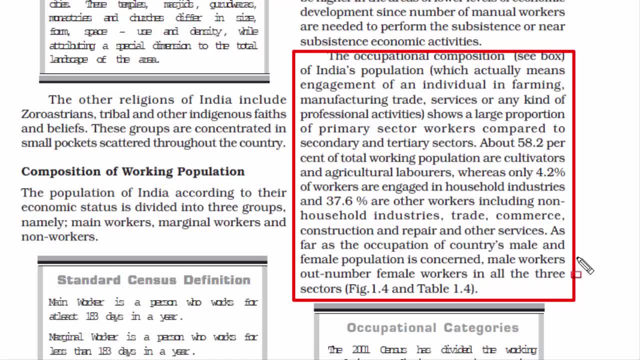 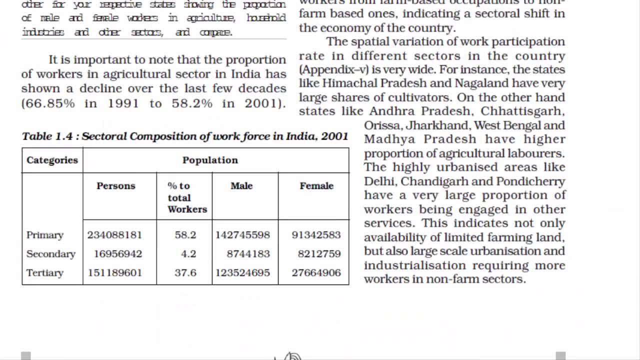 Broadly, these four different sectors are summed up under three broad categories: agricultural sector, industrial sector and service sector. Here in table 1.4, you can see the sectoral composition of workforce in India as per 2001 data. This table shows the number of people employed in different sectors. 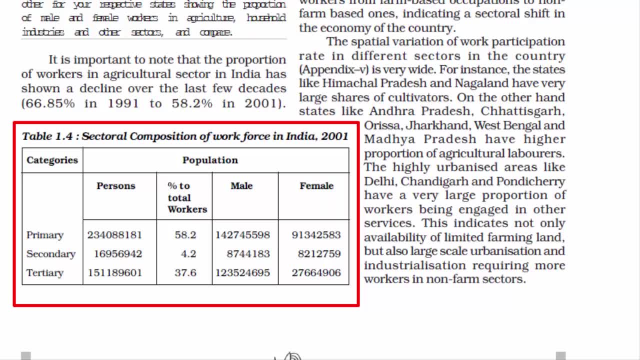 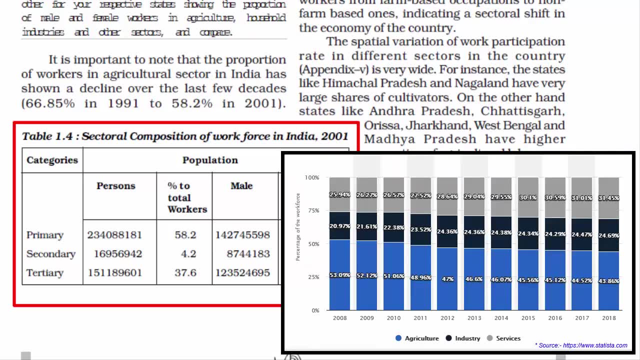 And it also shows the male and female contribution. Clearly, male workers have outnumbered female workers in all the three sectors Since the data is from 2001,. the present distribution of workforce across economic sector is this: You will notice the percentage of workforce in agriculture has reduced. 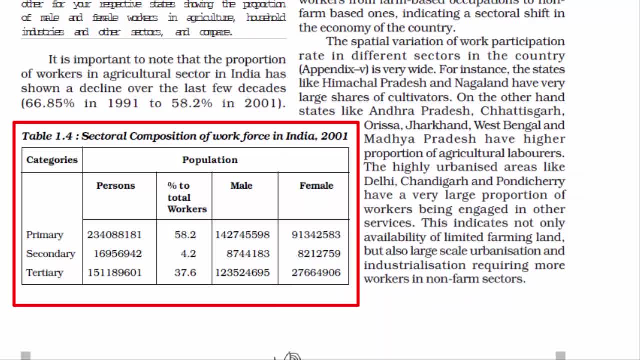 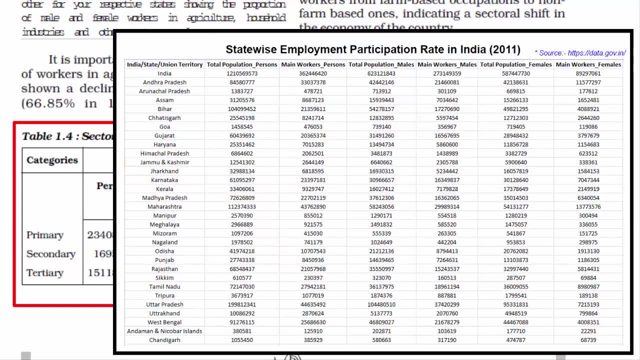 But it has increased in the tertiary and secondary sector. Now I could not find the data on gender wise work contribution In different sectors of the economy, While we do have data on state wise participation of male and female in the economy, But that is not the point. 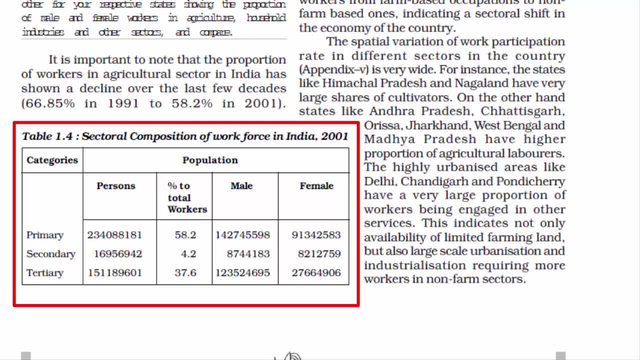 What we need is sector wise male and female contribution in the economy, And in that we can see the trend as to where the women contribute more compared to men, Because in recent years there has been some improvement in work participation of women in secondary and tertiary sector. 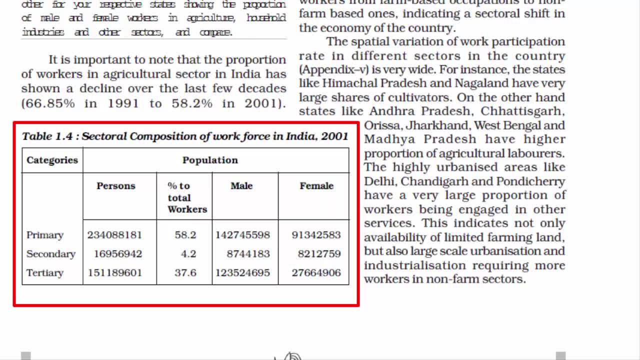 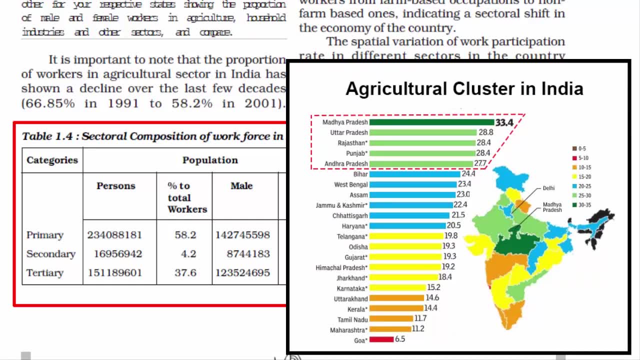 If you find any data, please paste the link in the comment section so that people can look at it. Here is a map of India that shows the agricultural clusters, In other words, the largest agricultural producing states of India. Now these are the major industrial regions of India. 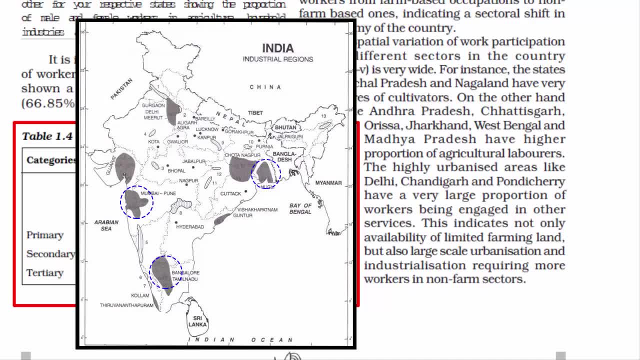 Mumbai to Pune Industrial Region, Hugli Industrial Region. Bangalore to Tamil Nadu Industrial Region. Gujarat Industrial Region, Chhota Nagpur Industrial Region. Vishakhapatnam to Guntur Industrial Region. Gurgaon to Delhi, Meerut Industrial Region. Coalfarm to Thiruvananthapuram Industrial Region. 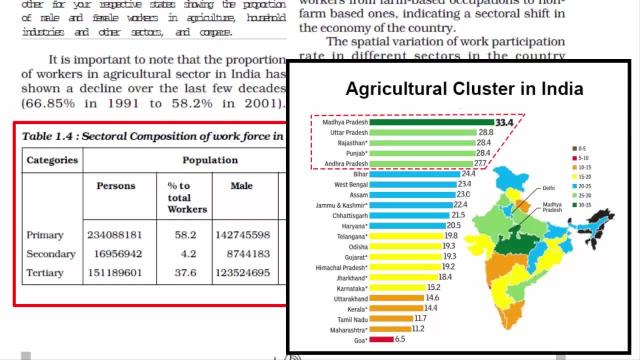 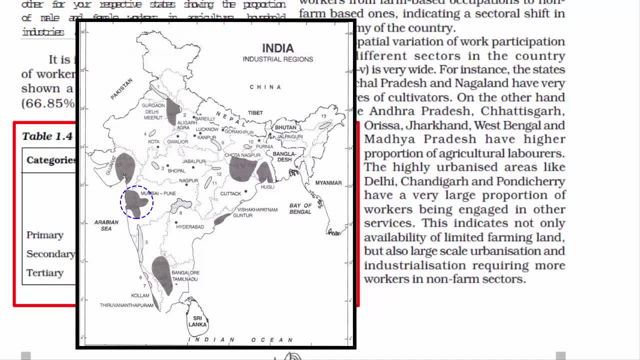 In other words, the largest agricultural producing states of India. Now these are the major industrial regions of India: Mumbai to Pune Industrial Region, Hooghly Industrial Region. Bangalore to Tamil Nadu Industrial Region, Gujarat Industrial Region, Chhota Nagpur Industrial Region. Vishakhapatnam to Guntur Industrial Region. 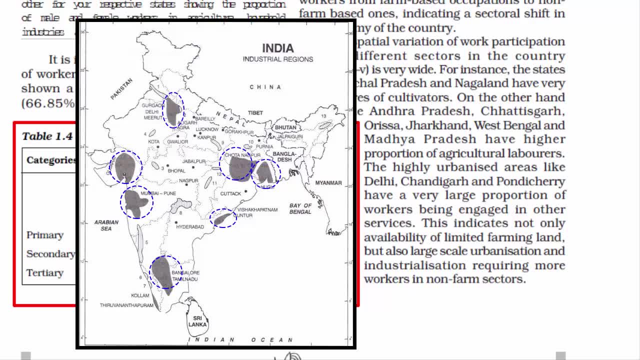 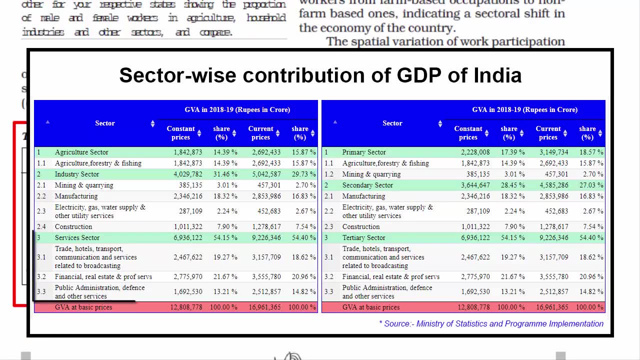 Gurgaon to Delhi, Meerut Industrial Region, Coal Farm to Thiruvananthapuram Industrial Region. Now coming to the service sector. Under service sector we have tourism IT services, So it's hard to get any data which directly shows which all states contribute. 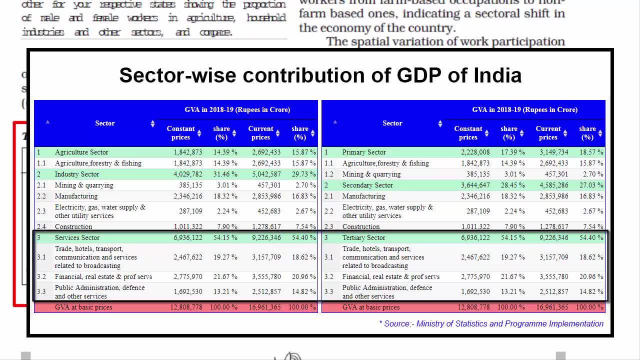 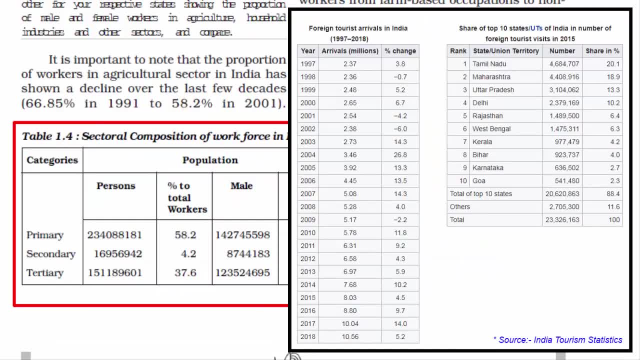 heavily in the service sector industry. What I've done is pulled out the data regarding which state contributes heavily in tourism and IT services In terms of tourism, since it is the major revenue generating industry, And here is the list of top 10 states of India. 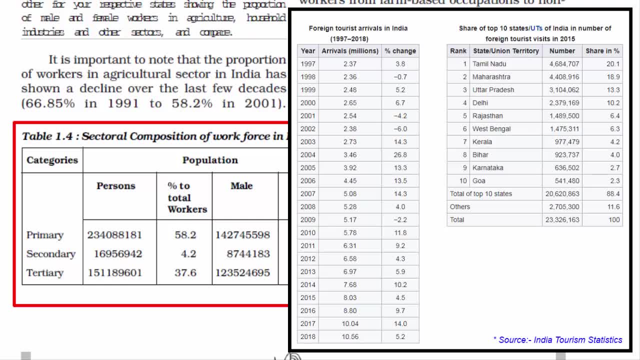 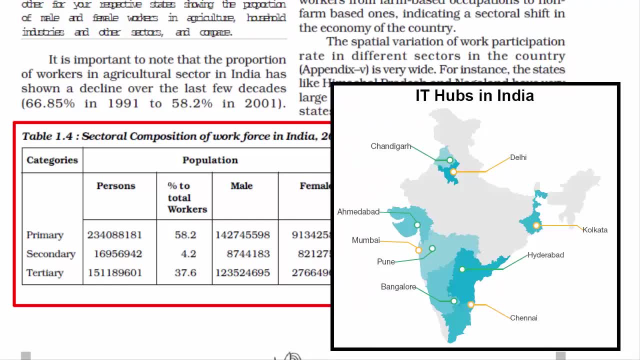 in terms of number of foreign tourists visits. The data is from 2015.. Have a look at it and get an overall idea about it. In terms of IT services, the major information technology hubs in India are located in the following cities: Bangalore, Hyderabad, Pune, Chennai, Delhi, Chandigarh, etc. 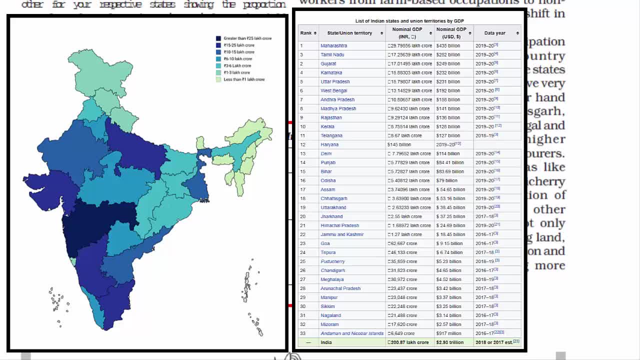 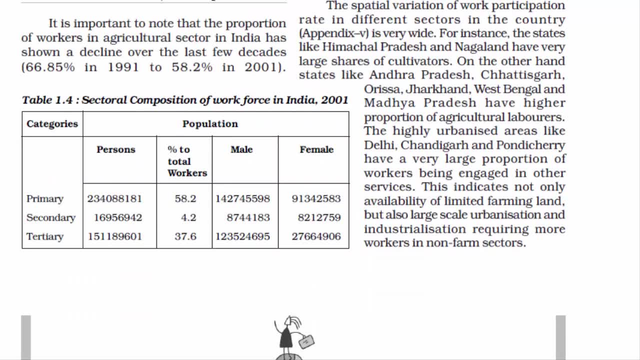 And finally, if you want to know which Indian state contributes maximum to India's GDP, here is the list. So with this we have come to an end of this chapter. The question answers can be found on the website. The link is there in the description. 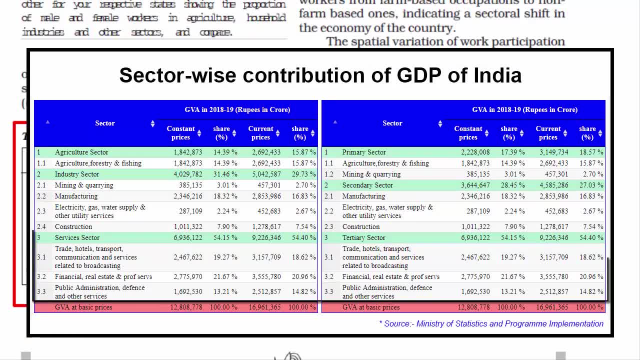 Now coming to the service sector. Under service sector we have tourism, IT services, So it's hard to get any data which directly shows which all states contribute heavily in the service sector industry. What I've done is pulled out the data regarding which state contributes heavily in tourism and IT services. 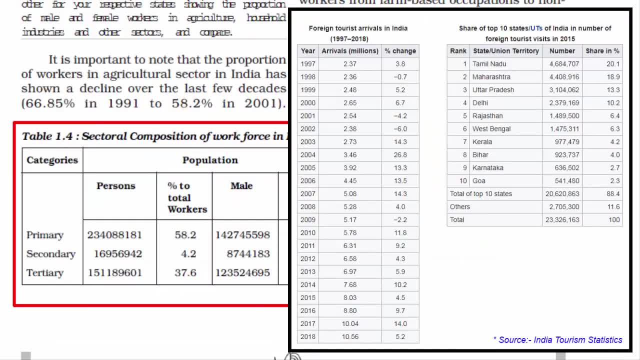 In terms of tourism, since it is the major revenue generating industry. And here is the list of top 10 states of India in terms of number of foreign tourists visits. The data is from 2015.. Have a look at it and get an overall idea about it. 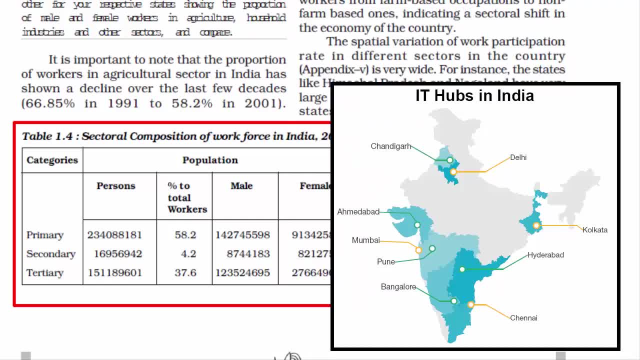 In terms of IT services, the major information technology hubs in India are located in the following cities: Bangalore, Hyderabad, Pune, Chennai, Delhi, Chandigarh, etc. And finally, if you want to know which Indian state contributes maximum to India's GDP, here is the list. 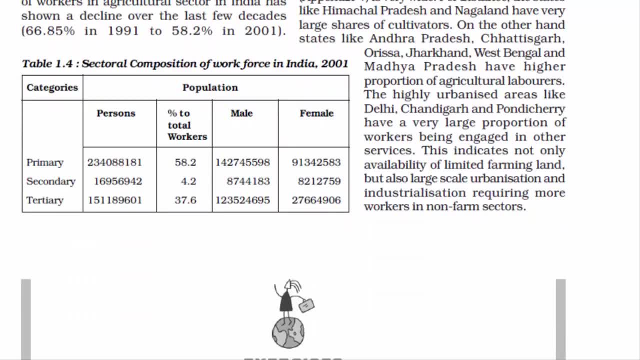 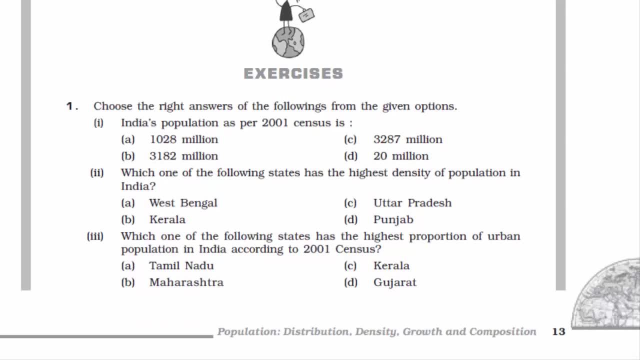 So with this we have come to an end of this chapter. The question answers can be found on the website. The link is there in the description, If at all you want to refer any data or do any further research on it. I have mentioned the sources from where I've collected and presented the facts and figures. 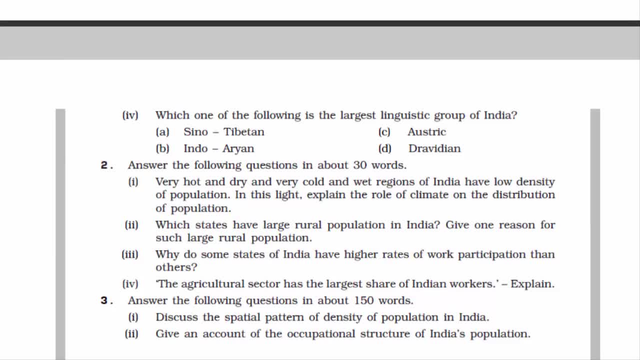 You can use the keyword, put it on Google and you'll get it. I hope you found this video informative. Let me know your thoughts in the comments section. Thanks for watching and I'll see you in the next one.